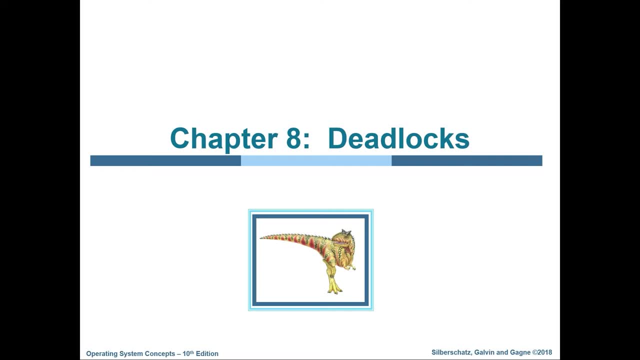 preserving the records. One more thing I'd like to say is that the software which we are using doesn't actually have a resource. What we need is a web folder, Big kind of a web folder that is made up of a lot, of, lots of different things can be resources. 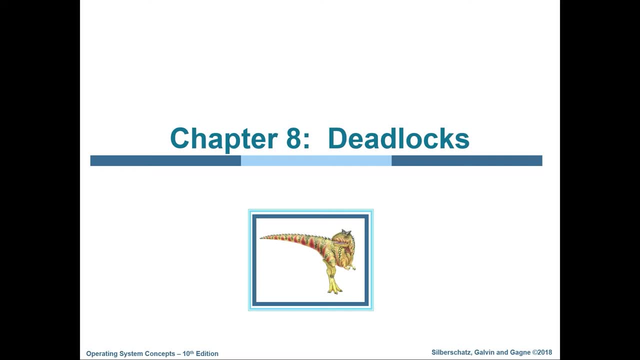 and processes need resources And it is not always guaranteed that when they request that resource from the operating system, that they always get it. And if they don't get it they have to wait. and if that resource which they need is being held by somebody else and that somebody else also needs more resources and they don't have. 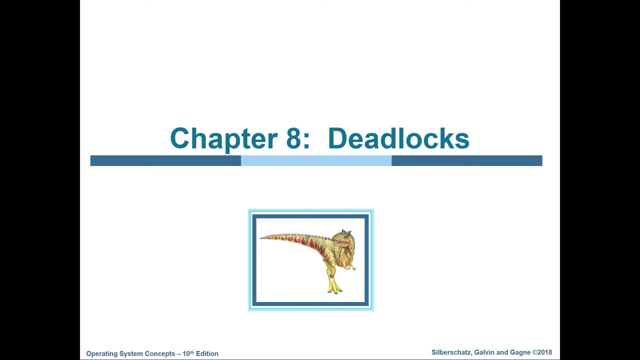 those resources. they are also waiting. And if there are a bunch of processes who are waiting on each of the consensus, try to go to Mongo 600 and find those resources. Yeah, reanimate those processes into yourorum for them to practice, And this is the process that they are. 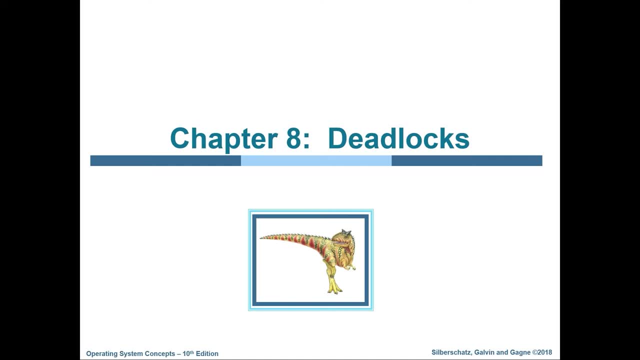 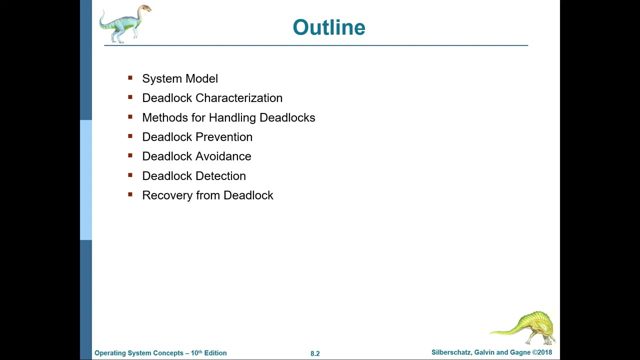 other for resources and they're not able to move anywhere. that means the system is in a deadlocked state. so let's see how this all works in this presentation. so this is the agenda for today's class. so we will be looking at the system model, in which we will see how we represent resources, processes and how we 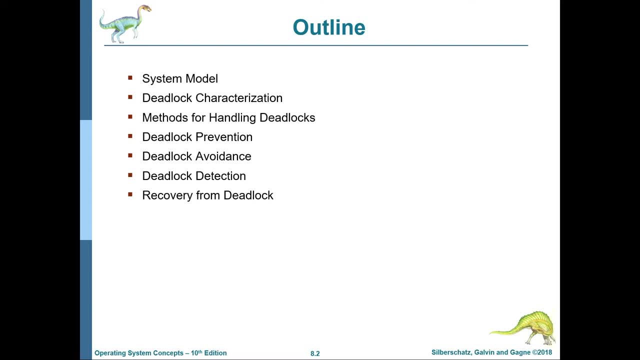 can represent them using a graph. right, so there can be requests, there can be assignments and different things. then we will move on to characterizing deadlocks. there are about four different conditions that must hold simultaneously for deadlocks to happen, and we will see each one of them in a 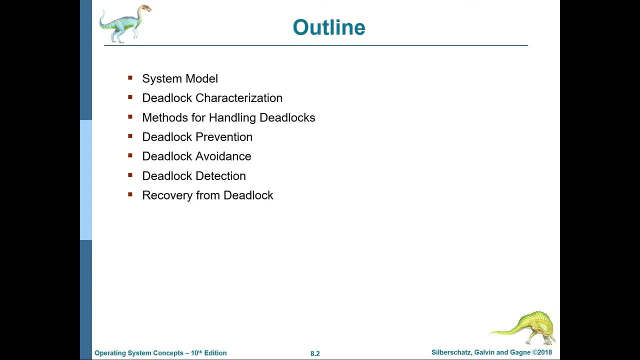 great amount of detail. then we will move on to see how deadlocks can be handled right so you can prevent deadlocks. you can avoid deadlocks or you can pretend that deadlocks never happen, or you can let deadlocks happen and know how to recover from. 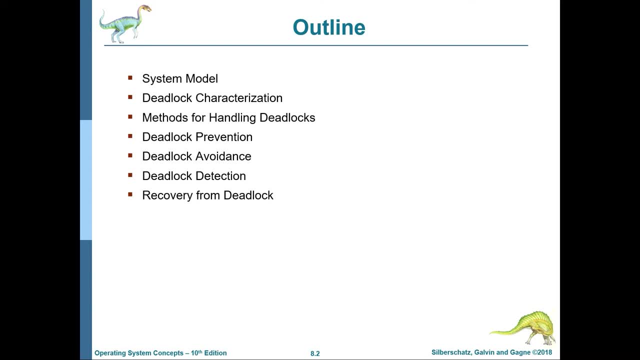 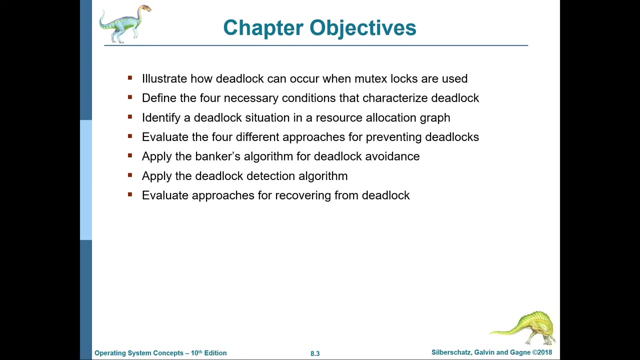 deadlocks right. so we will be looking at deadlock prevention, deadlock avoidance, deadlock detection and recovery from deadlocks. so these are the objectives of this chapter. so we will see a simple example in which we will use a couple of mutex locks and I will demonstrate to you how a deadlock can happen even in this very simple. 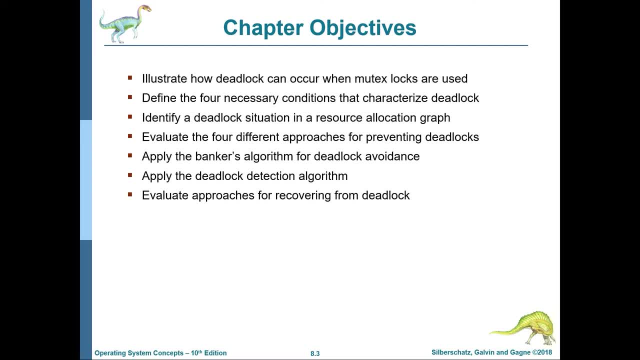 situation. then we will go on to define four necessary conditions that can characterize deadlocks, and these four conditions have to happen simultaneously at the same time for a deadlock to happen. then we will learn about resource allocation graph it is. it is basically a graph which has processes and resources on it and it has a bunch of request and assignment. 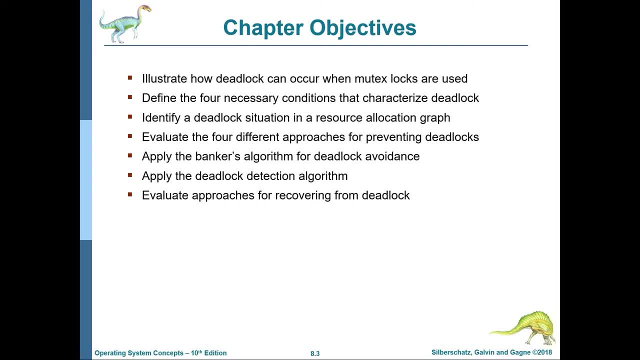 edges and we will see if the graph has cycles, whether that can signify a deadlock situation or not. Then we will investigate four different approaches for preventing deadlocks. So when I said before there are four necessary conditions, If we break one of those conditions, one or more, 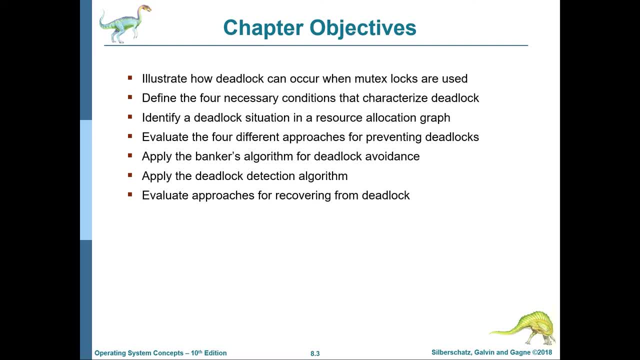 of them. then we can prevent deadlocks and we will see how to do that. Then we will move on to learning about deadlock avoidance. Prevention is good, but if you cannot always prevent, you can do your best to avoid the situation and we will see how simple algorithms like the banker's algorithm 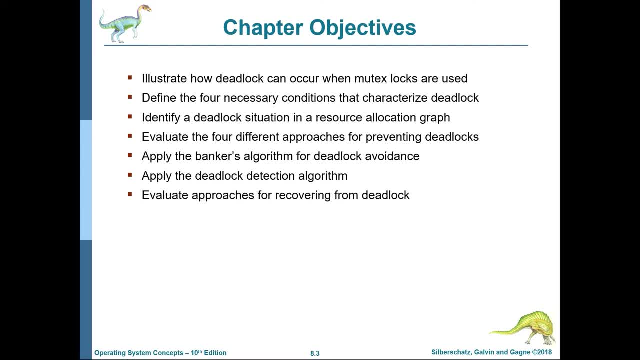 and other things can help us avoid deadlocks. Then we will move on to the next step, which is the deadlock avoidance. We will move on to see how a deadlock can be detected. if you could not prevent or avoid a deadlock, Well, you could detect a deadlock, because deadlocks will happen if you don't prevent or avoid them. 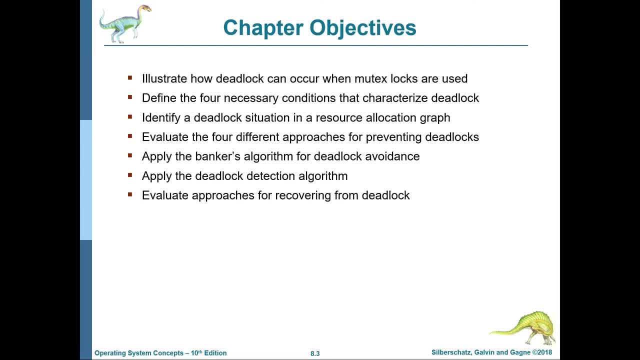 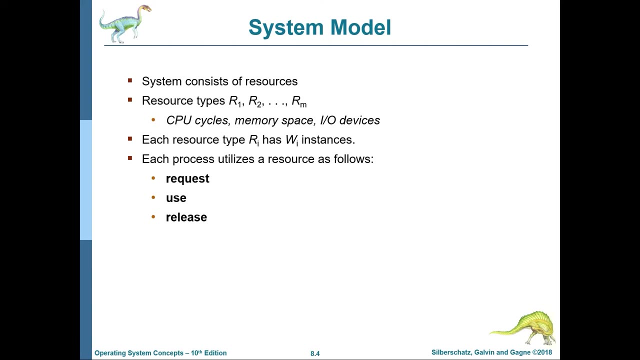 but you can do your best to detect them, and then we will learn about different approaches to recover from a deadlock. If it has happened, you have detected it. now you can recover from it. Let's look at the system model first. As I said before, we have a system model and we have a system model which is a system model. 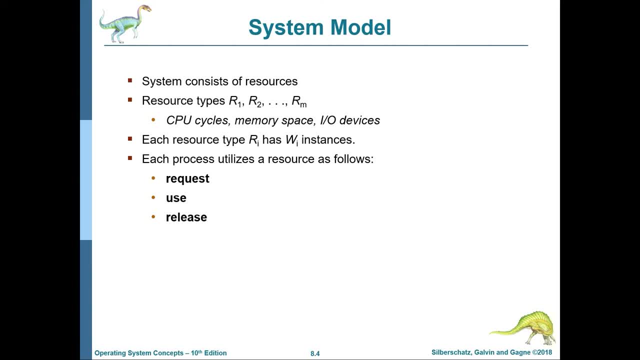 As I said before, a system consists of resources and the resources can be categorized into different types and we can number them, the types as r1, r2 up to rm. When I say types, I mean r1 could be all the cd-rom drives and there can be one or more than one cd-rom drives. that can all be. 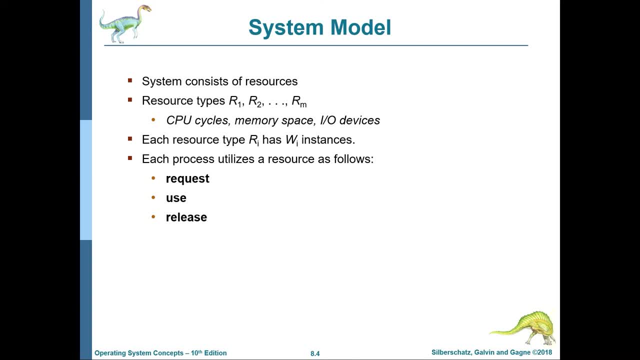 grouped into r1.. So r1 is a type and it can have one or more than one instances of that type of resource and it should not matter which one of them the operating system gives to a process when it is requested. So if there are three cd-rom drives they are all categorized as r1. that is a resource. 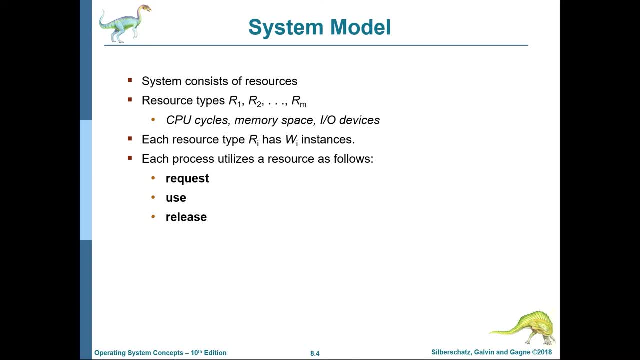 type, and if one of them is already occupied, then out of three, two of them are available, and next time another process comes and asks for a cd-rom drive, the operating system can give them any one of the two free cd-rom drives, And it should not matter which one it gives. So that is the concept of resource types. 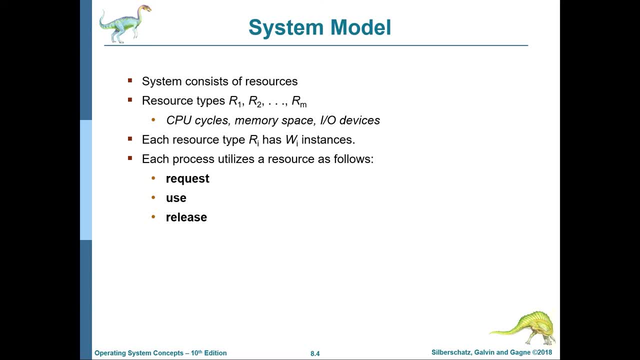 You should also keep in mind that things like very small things and important things like cpu cycles, memory space, are also examples of resources. Now, cpu cycles might look like something very, very normal and natural processes to hold on to, but they are also resources and you have learned before. 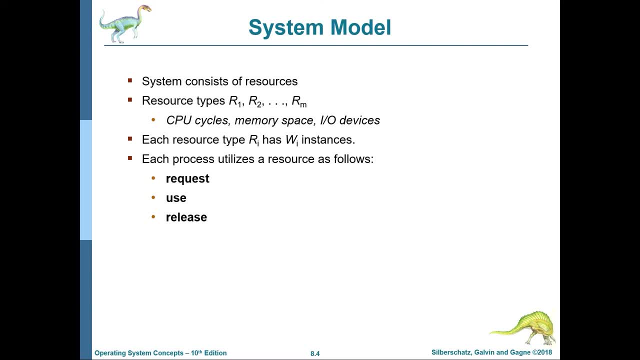 how the scheduler helps to maintain a fair access to cpu cycles by processes. So, as I said before, each resource type ri has wi instances as in: if r1 is a set of all cd-rom drives in your computer, then if it is, if it has three cd-rom drives, then wi, that is, w1, would be. three. Each process utilizes a resource type. So if r1 is a set of all cd-rom drives in your computer, then if it is, if it has three cd-rom drives, then wi, that is, w1, would be three. Each process utilizes a resource type. So if r1 is a set of all cd-rom drives in your computer, then if it is, if it has three cd-rom drives, then wi, that is, w1, would be three. 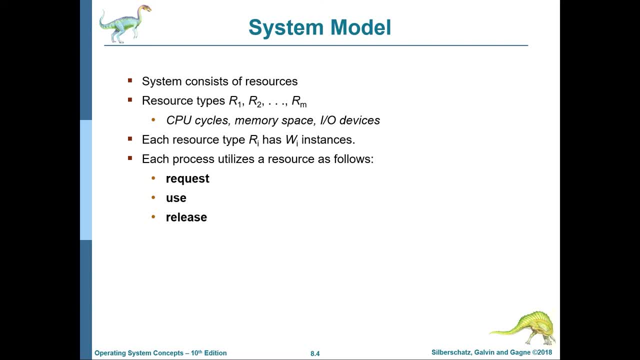 Each process utilizes a resource type. So if r1 is a set of all cd-rom drives in your computer, then if it is, if it has three cd-rom drives, then wi, that is, w1, would be three. Each process utilizes a resource as follows: right. 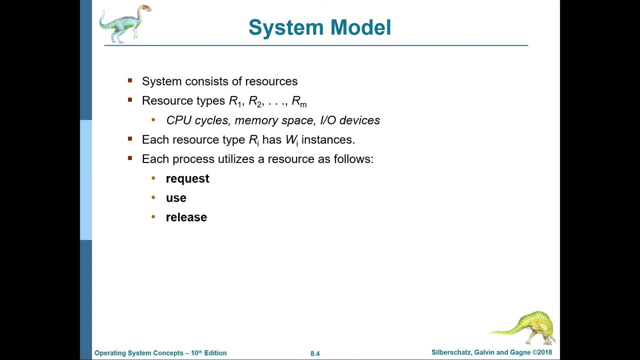 So it must request a resource to the operating system. and what can happen? if it does not get the resource right away, Then it must wait right. So in your scheduling chapter you learned about the process states, So there could be new processes, ready processes, running processes, blocked processes. 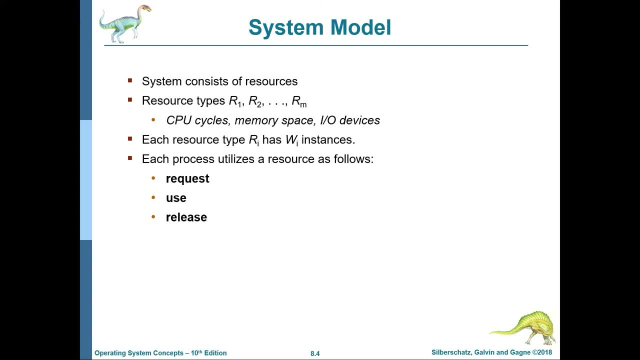 and processes in the exit or terminated state. So what are the blocked processes doing? Because they asked for a resource or a lock and they could not get it, so they had to wait until the operating system was able to give it to them. So a process will make a request for a resource. 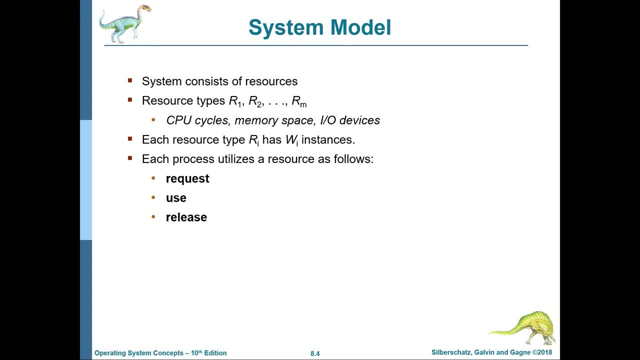 If it gets it, then it will use the resource and after it has used the resource, it has to release the resource back to the operating system. When it requests and it does not get the resource, it has to wait until the operating system gets the resource back from another process. 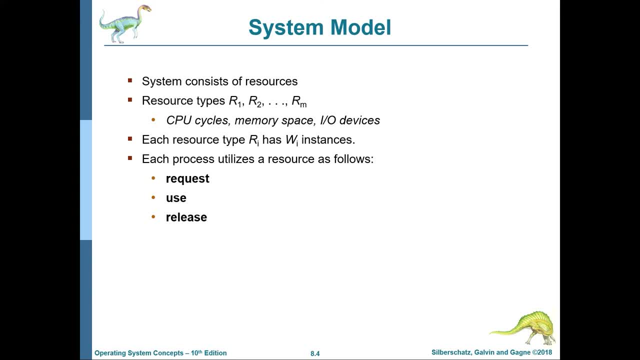 and then it gives it to this process, which has been waiting for that resource. Let's look at a very simple example on how a deadlock can happen with semaphores. So we have two semaphores, S1 and S2, each initialized to 1.. 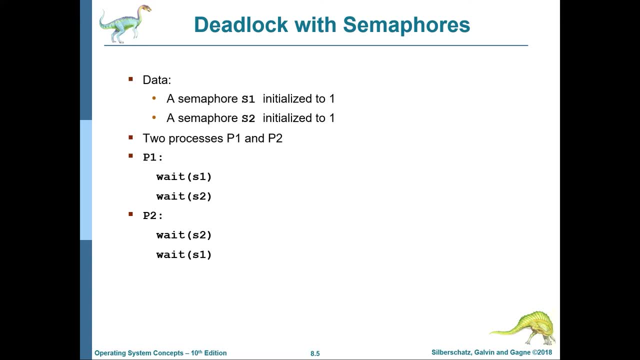 And there are two processes: P1 and P2.. Look at the code for P1. It is first waiting on S1, so it decrements S1 from 1 to 0, and then it is waiting on S2, that is, it will make an attempt. 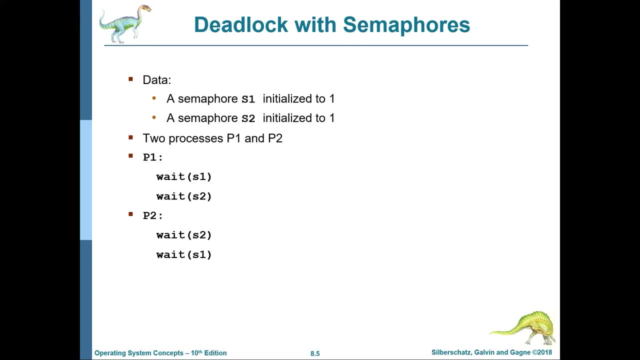 After it gets a hold on S1, it will make an attempt to also decrement S2 from 1 to 0.. Look at what P2 is doing. It is first waiting on S2 and then it is waiting on S1.. Can you pause for a moment and think how a deadlock can happen in this situation? 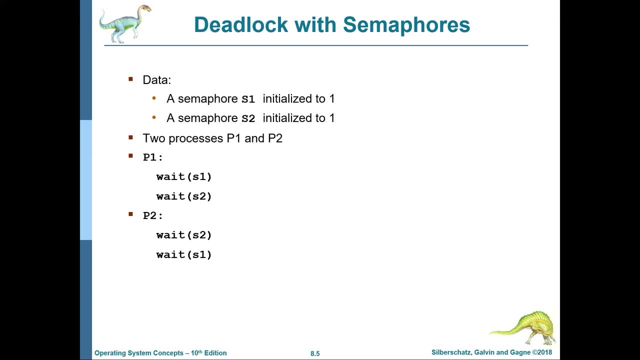 Well, just imagine when P1 executes the first line, that is, it has successfully decremented the semaphore S1, and then it gets context switched out. Or if it is a multiprocessor system, P2 gets scheduled on S1. Another core- and before P1 could decrement S2, P2 decrements S2.. 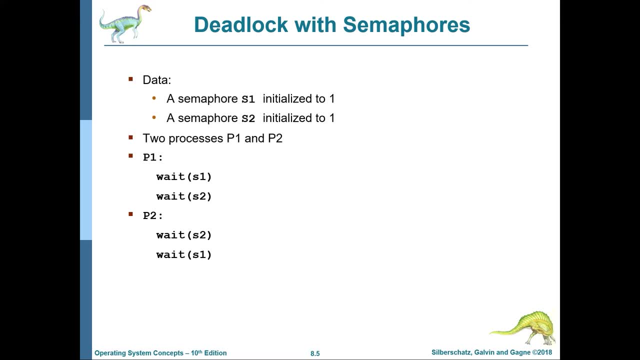 And now it will go on to wait for S1.. Now that is a deadlock situation, because P1 is now waiting on S2, which P2 has already grabbed, and P2 is waiting on S1, which P1 has already grabbed. Now both the processes- P1 and P2, cannot proceed any further. 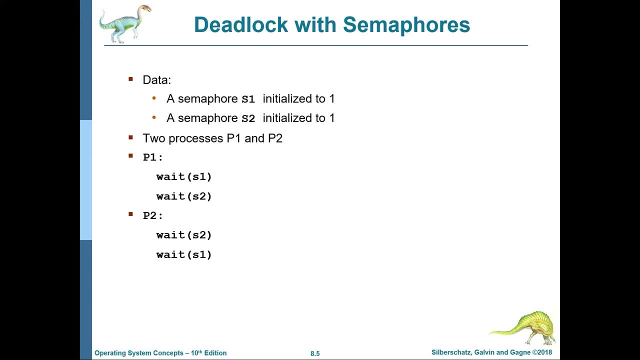 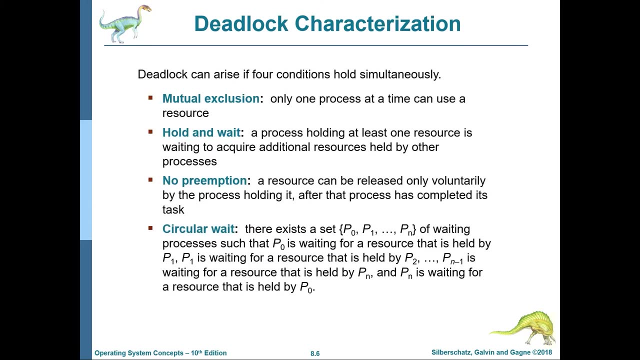 And that is a coincidence. This is a classic example of a deadlock that can happen with just two semaphores. As I said before, for a deadlock to happen, four conditions have to hold simultaneously. Now let's look at those four conditions one by one. 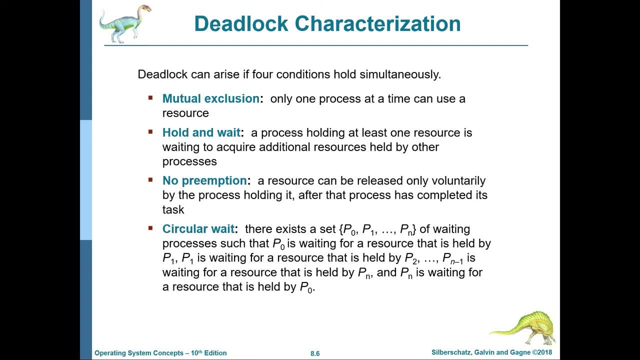 Mutual exclusion: Only one process at a time can use a resource. If this condition holds true, then it is one of the ingredients for a deadlock. Now there are many resources which can be shared, right? So if there is a read-only file whose contents are not being changed actively, 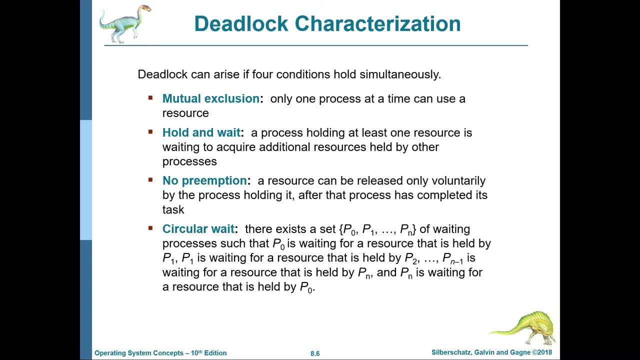 then many processes can read from that file at the same time. So that is an example of a shareable resource. There there is no need for mutual exclusion to happen. But think about a printer. Can two processes print at the same time on a same page? 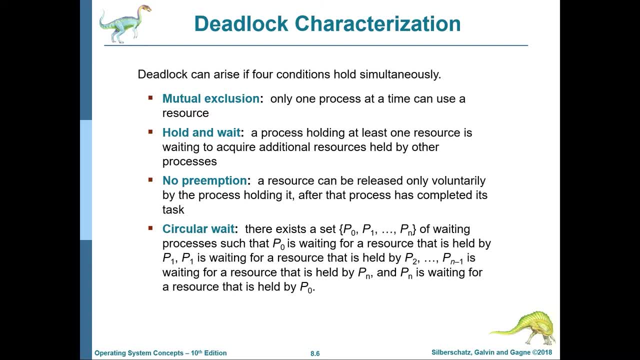 Print at the same time on a single printer, You will see one line from one process. You will then see another line from another process. That is not useful work. So most resources on a system are non-shareable And that is a perfect ingredient for a deadlock to happen. 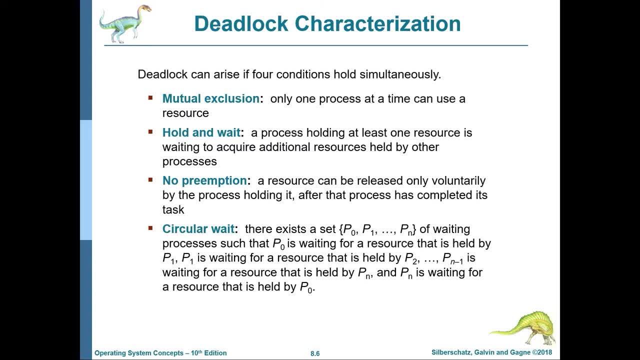 Then we will move on to hold and wait. So processes usually need more than one resource, More than one resource for them to work. For example, if there is one process that needs three resources, It needs the CD-ROM drive, the hard drive and then the printer. 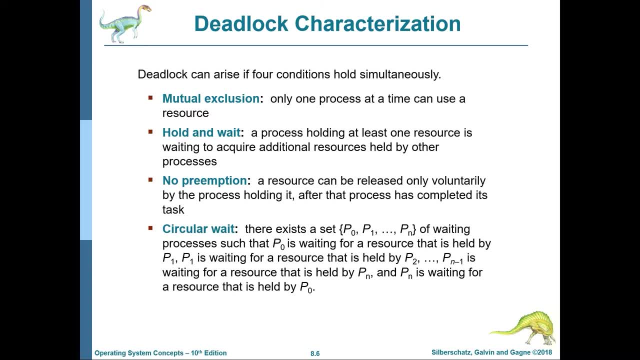 And its job is to fetch something from the CD-ROM drive, copy it to the hard drive and then read from the hard drive and then print whatever is the content of a document. So it needs the CD-ROM drive, the hard drive and the printer. 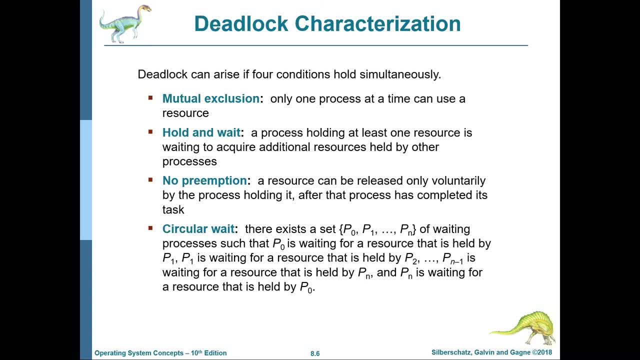 What if it can only get access to the CD-ROM drive and the hard drive and not the printer? So what if the process just grabs, hold kind of reserves the CD-ROM drive and the hard drive for itself and then keeps waiting for the printer to be available to it? 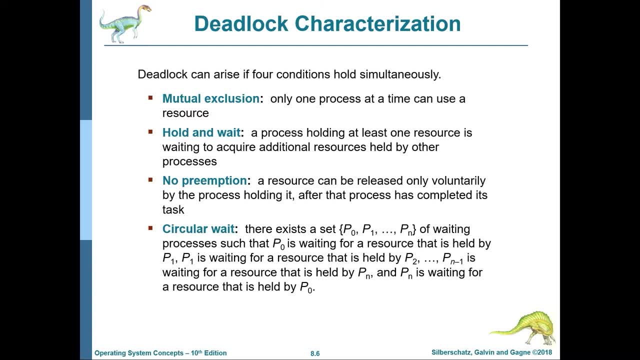 Now that is an example of hold and wait. So you hold on to whatever resources are available, a subset of the exhaustive set of resources that you will need for your job. You hold on to a subset of that. In this example, there is the CD-ROM drive and the hard drive. 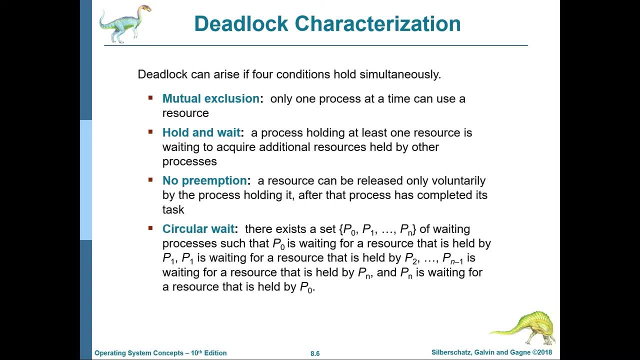 And you keep waiting for the rest of the resources to be available for you. So that is hold and wait, And if that happens, then deadlocks can happen. That is one of the other ingredients for deadlock to happen, And you can see why. 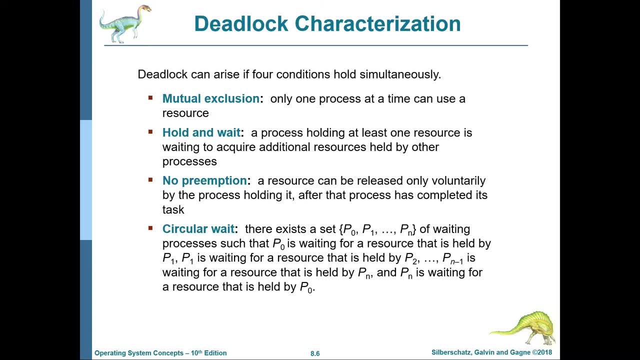 Because if it has access to the CD-ROM drive and the hard drive and it reserves it, and if it keeps waiting for the printer and the printer is with someone who needs access to the CD-ROM drive now, that process cannot get the CD-ROM drive. 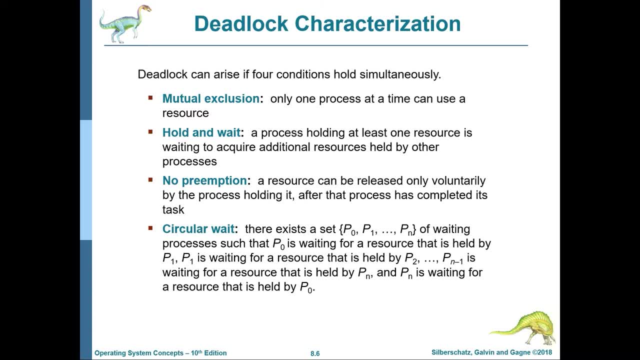 but that process is holding on to the printer And this process is holding on to the CD-ROM drive and the hard drive, but it will never get the printer because the other process has held the printer with it. We will move on to the next condition. 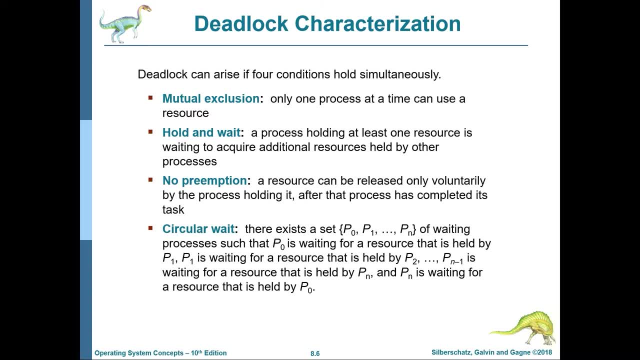 That is no preemption. Now you have probably heard of it. We have heard about the term preemptive scheduling. What is preemptive scheduling? A process is very healthy to keep continuing to execute on a CPU, but the scheduler preempts it. 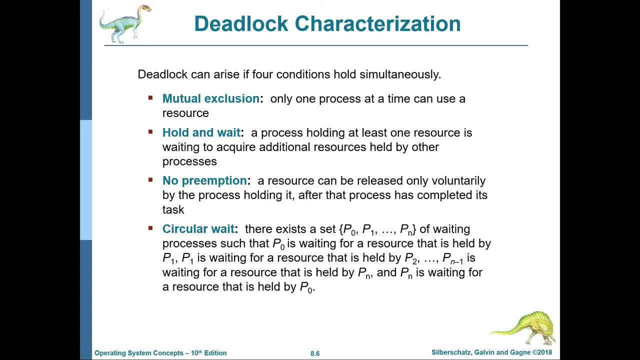 It removes it from the CPU and then it schedules another process in its place. That is preemption. Now, on a computer many things cannot be preempted. If a process is printing something, the operating system just cannot preempt the printer and say: 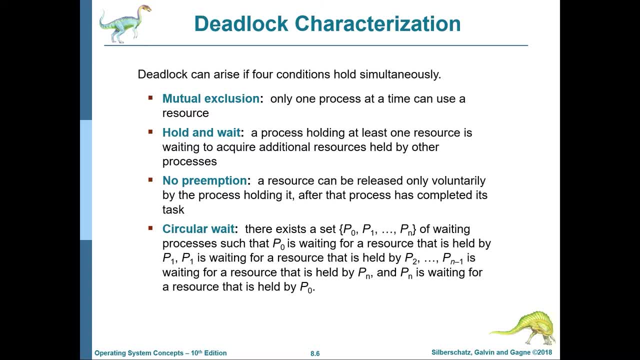 okay, you are done half printing. I am going to steal the printer from you and give it to another process. Now that cannot happen, right? So that cannot happen. That can be another ingredient for a deadlock to happen. So if no preemption can happen, then deadlocks can happen. 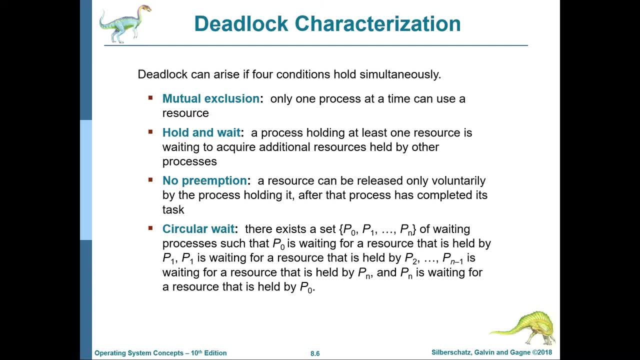 The last one is very interesting. It is called circular wait. So if P0 till Pn, they are all the processes in your system and if you can arrange them in this order- P0,, P1 and Pn- and if P0 is waiting for a resource that is held by P1,, 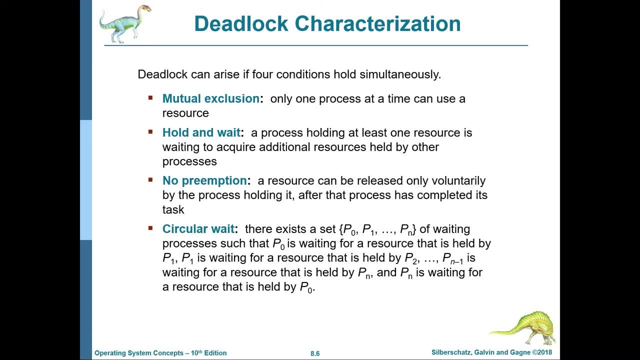 P1 is waiting for a resource that is held by P2, and so on. Pn is waiting for a resource that is held by P0. So you can kind of see a circle happening. It is kind of a linked list whose tail is connected back to the head. 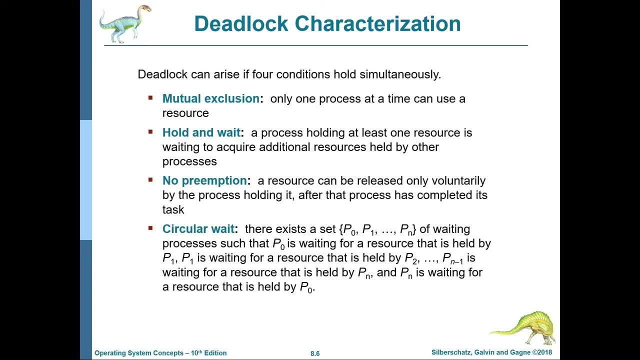 Tail is Pn and head is P0. So if you can arrange the processes in that order, then a deadlock can happen. So that is the fourth ingredient for deadlocks to happen. So P0 is waiting on P1 to release a resource. 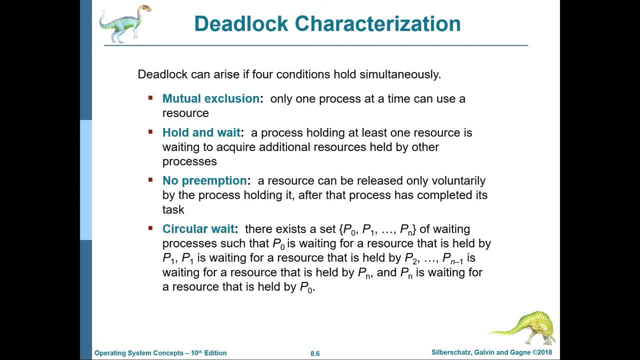 P1 is waiting on P2 to release a resource, and so on and so forth. So if that is happening, then a deadlock can happen. Now, if mutual exclusion hold and wait, no preemption circular, wait. all of these things are happening at the same time. 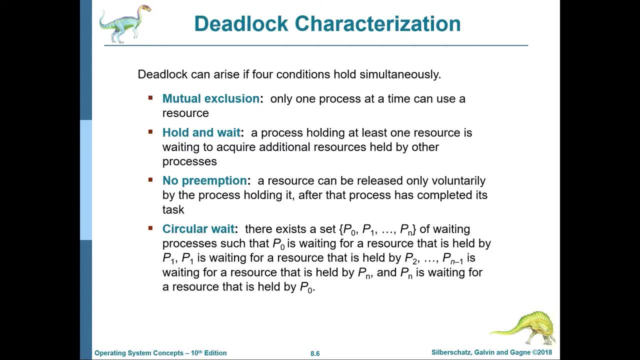 then deadlocks can arise. I am not saying that they will always happen. So by mutual exclusion we mean if there exists at least one resource which is non-shareable. by hold and wait we mean it is usual for processes to grab on to something. 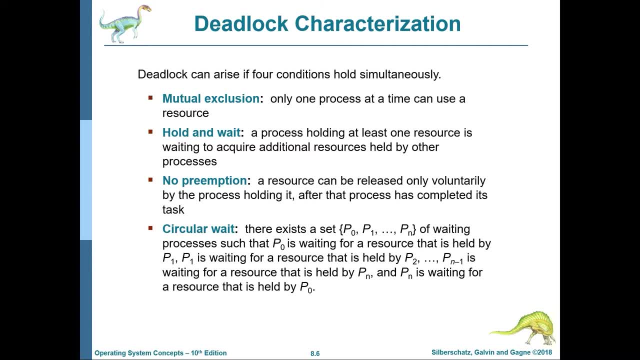 and then keep waiting for the rest of the resources to come. By no preemption I mean there exists a resource which cannot be preempted. if it is being held by one process, then the OS cannot take it midway, and there a circular wait condition is existing in the system at one point of time. 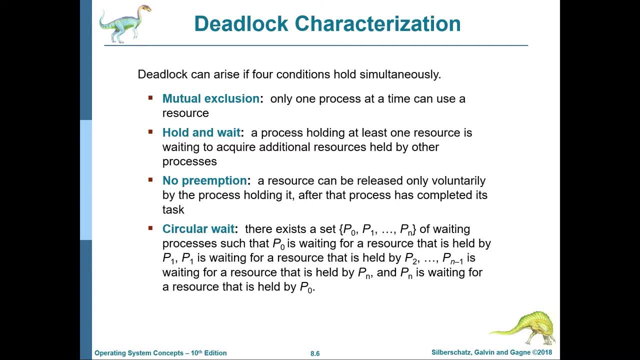 If all of these four situations are true at any one point of time, then that is a perfect recipe For a deadlock to happen. it does not mean that a deadlock has already happened, but if these four conditions are true, then a deadlock might happen. 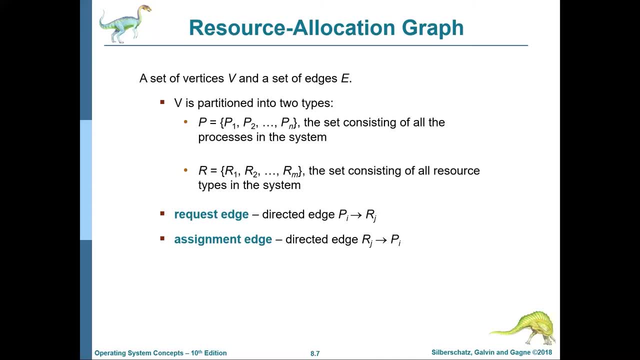 Let's look at the concept of a resource allocation graph Now. since it is a graph, it has got a set of vertices and a set of edges. Now the set of vertices can be divided into the set of processes from P1 to Pn. 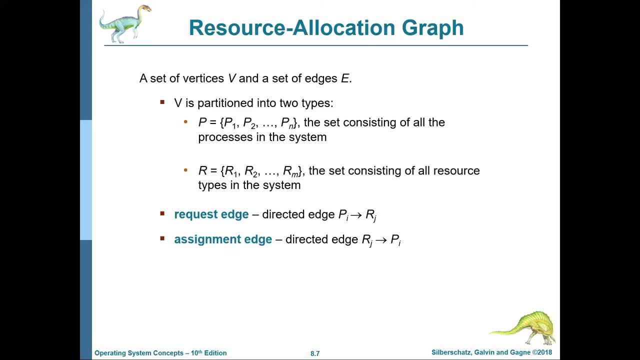 and the set of resources from R1 to Rm. For the purposes of this lecture, we will denote the nodes that signify processes in circles and the nodes that signify resources in rectangles. Now the edges can be of two types. There can be request edges. 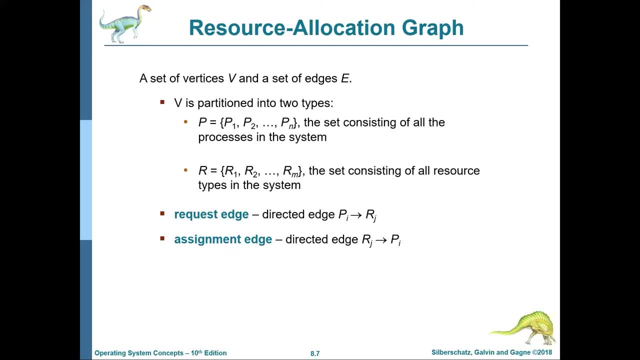 which are directed edges, and they always go from one process to a resource. And this edge means that the process from which the directed edges emanating starting from has a wish to acquire the resource towards which the edge is pointing. So here there is an edge from Pi to Rj. 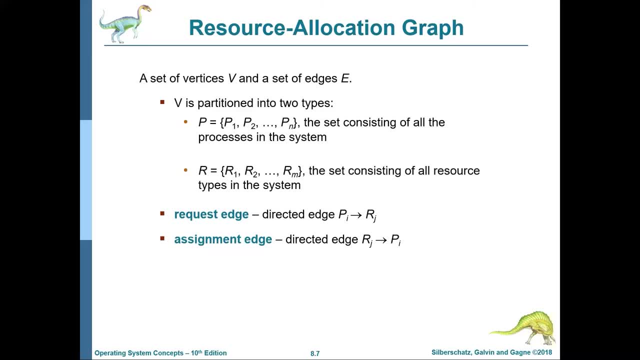 That means Pi has a wish that if Rj is available, then Rj should be given to Pi because it needs that resource for its work. And there can be assignment edges, Which are basically request edges, and when they get granted, the direction changes from Rj to Pi. 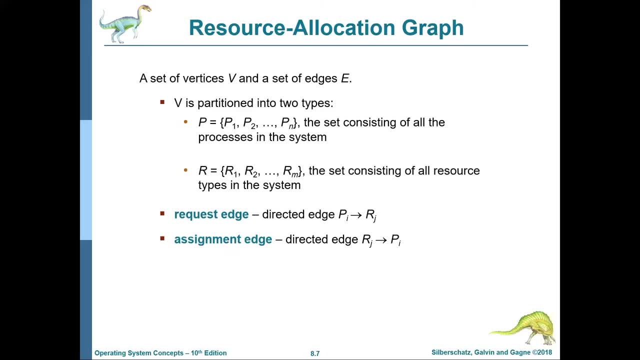 That means if Pi had at one point made a wish to acquire Rj and that the OS was able to give it to that process at one point of time, then the direction of the edge will change and it will now become an assignment. That means the resource has already been given to the process. 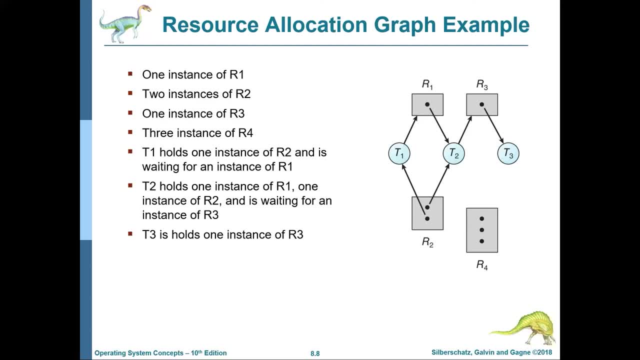 This is an example of a resource allocation graph. Here you can see there are three processes- T1, T2 and T3, which are inside circles, And there are four resources: R1, R2, R3 and R4.. And the dots that you see. 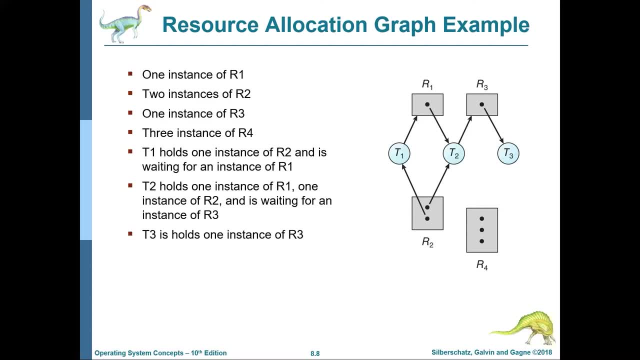 in those rectangles which denote the resources are the number of instances of that resource type that is present. So if R4 is the set of CD ROMs, then there are three dots inside that rectangle. That means there are three CD ROM drives in the system. 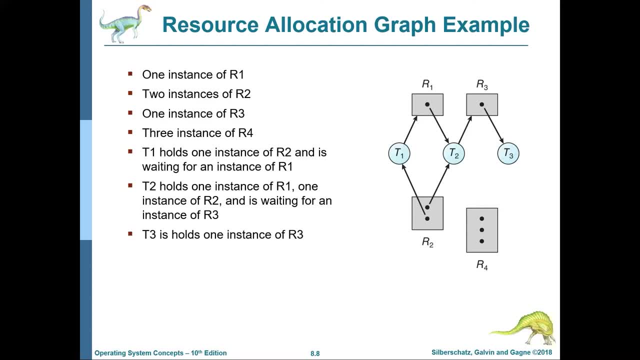 If R2 is the set of hard drives, then the node for R2 has two dots and that means there are two hard drives in the system. R1 and R3 each have just one instance of that type. Now let's look at the arrow from T1 to R1.. 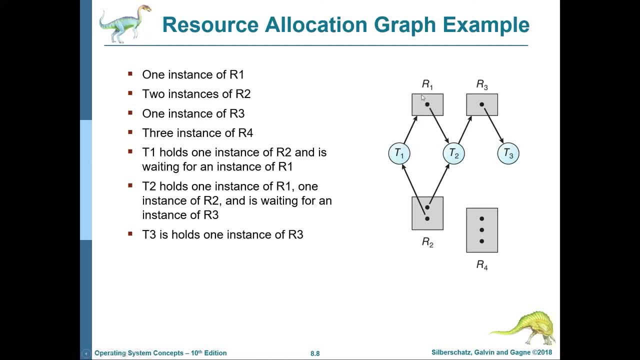 What does that mean? It is a request edge. That means that T1 has a wish that it needs one instance of R1 and whenever it is available, it should be given to T1.. Now, similarly, there is a request for R3 by T2.. 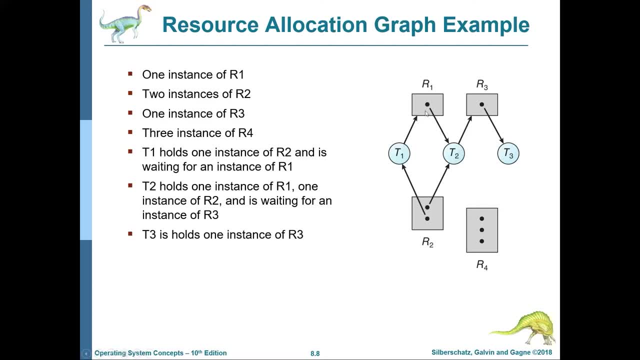 Now let's look at the assignment edges. Now there is an assignment of R1 to T2.. What does that mean? At this point of time, T2 is using one instance of R1.. T3 is using one instance of R3. 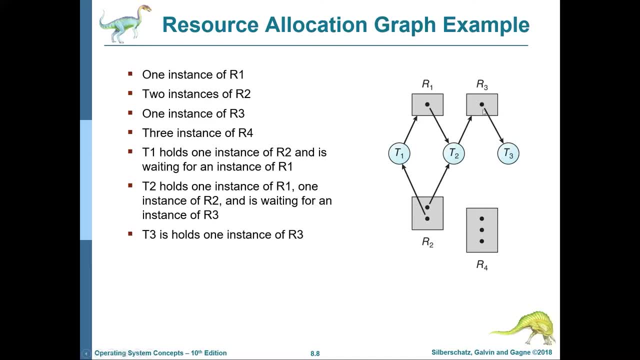 because it is an arrow. it is an edge that points from the resource to the process. Assignment edges always go from a resource to a process. Request edges always go from a process to a resource. And there are two other assignments here. One instance of R2 has gone to T1. 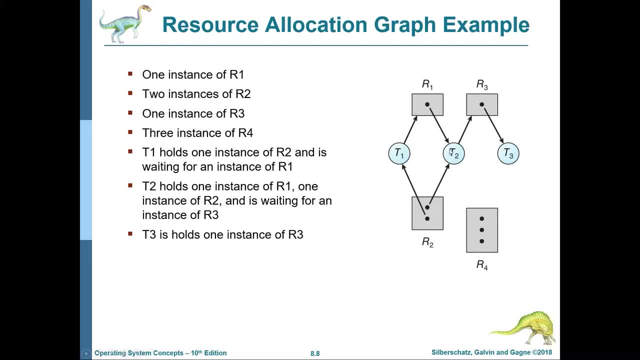 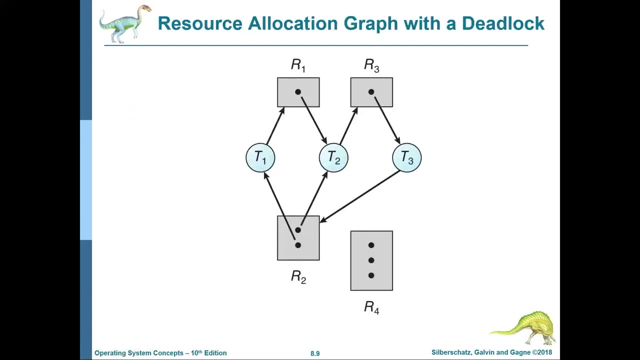 and another instance of R2 has gone to T2.. All the instances of R1 to T2 are free and no process is using them or no process is even requesting them at this point of time. Now, this is a resource allocation graph that has a deadlock. 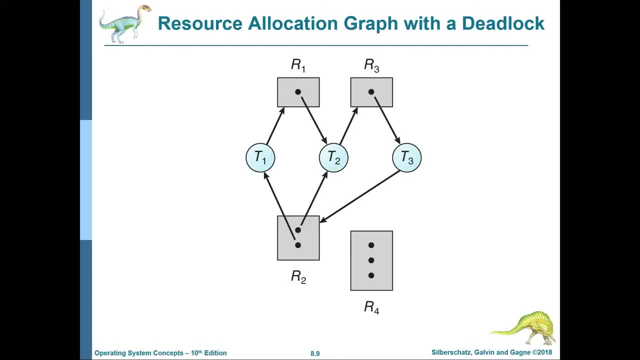 Please pause for a moment and look at the screen to figure out why there is a deadlock. There is a deadlock because T1 wants one instance of R1 and it has not been granted that instance because that instance is currently being held by T2.. 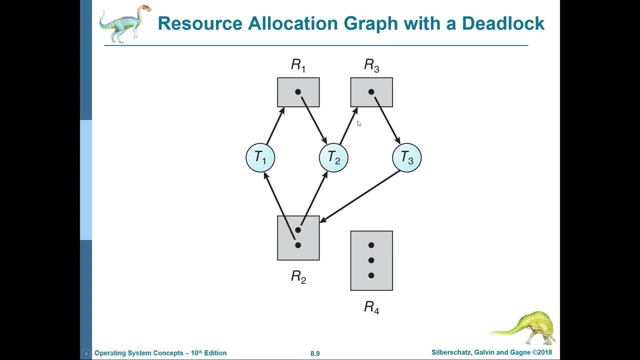 T2 is not able to proceed any further because it needs one instance of R3 before proceeding. but that single instance of R3 has already been reserved by T3 and it is currently using that single instance of R3.. T3 is not able to move any further. 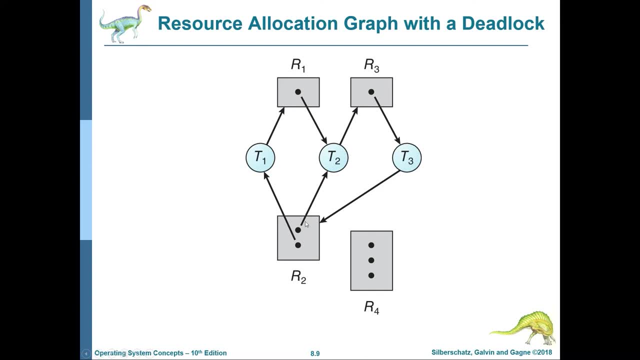 because it needs one instance of R2, but both the instances of R2 have gone one each, to T1 and T2.. Now you can see why there is a deadlock: T1 is waiting on that one resource which T2 has, and T2 is waiting on that one resource. 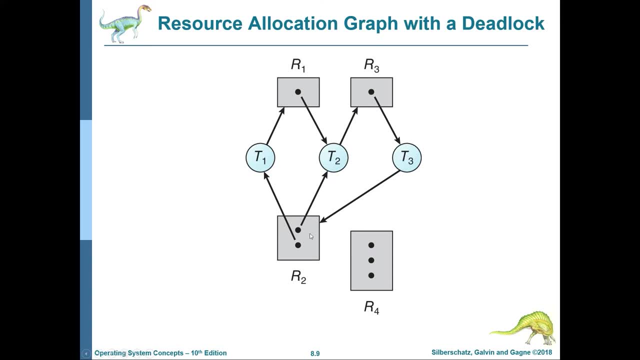 that T3 has, and T3 is waiting on one resource that T1 and T2 have. So they are in a deadlock and they are not able to proceed any further. You should also note that this graph has a cycle. Now this is one cycle over here. 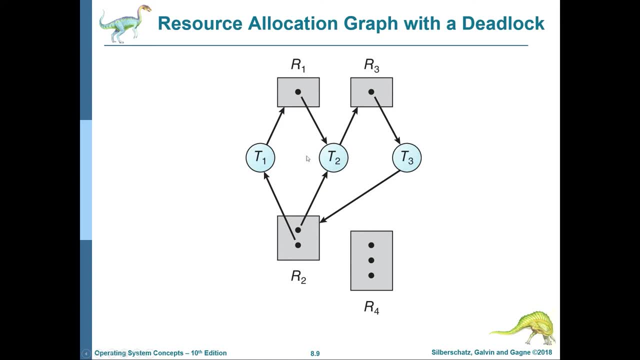 and this is another cycle over here- And we will see that if there is a cycle in a resource allocation graph, then there is a possibility of a deadlock. It is not always guaranteed that there is a deadlock, as we will see in the next slide. 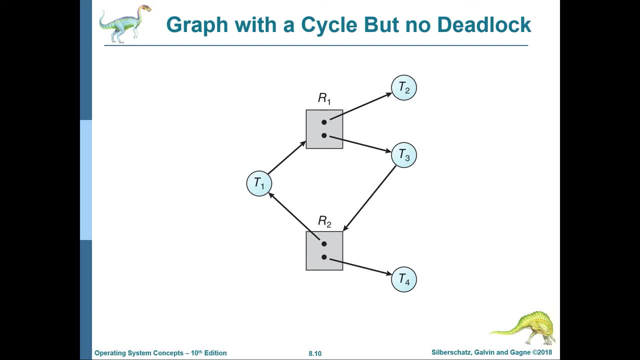 Now this graph has a cycle, but there is no deadlock. Now you should again pause and see why there is no deadlock in this situation. There is no deadlock in this situation because T4 has one instance of R2.. But when T4 is done with that, 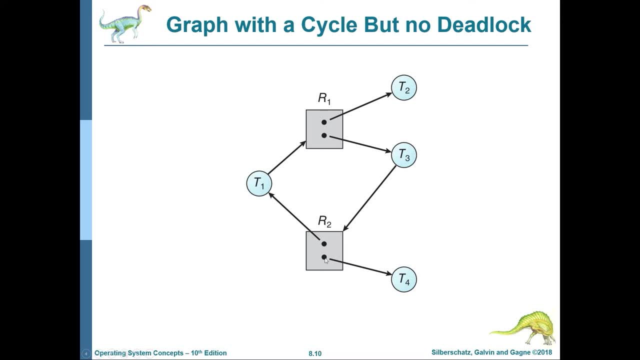 it is going to give it back And once it gives it back, T3 is going to grab it. T3 will be done with its job Now. T3 will release R2 back and it is also going to release that single instance of R1 it has. 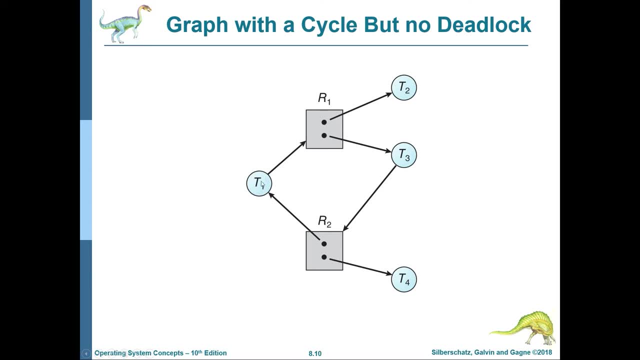 That one instance of R1 will be given to T1 and T1 will also be able to complete. T2 always had whatever it needed and T2 will independently proceed anyway. So this graph, although it has a cycle, but there is no deadlock in this situation. 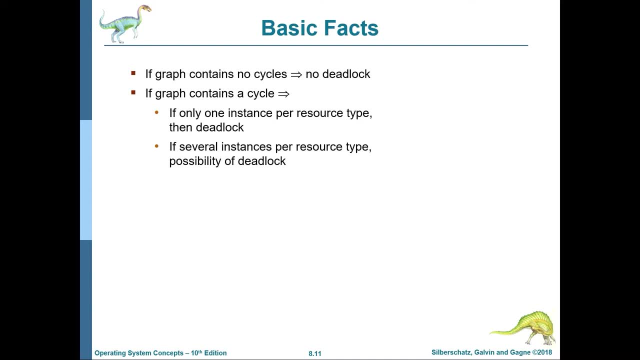 So let's summarize the basic facts here: if a resource allocation graph contains no cycles, then there is no deadlock. If the graph contains a cycle, but if only one instance per resource type is there, then there is a deadlock. If several instances per resource type are there, 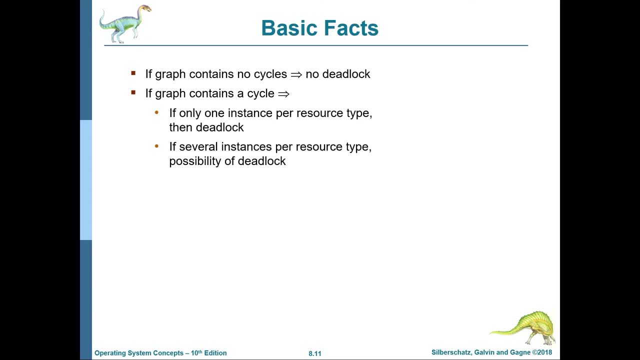 then there is a possibility of deadlock. So what do I mean by saying that if only one instance per resource type is there? I mean to say, if only one instance per resource type is there, then inside these rectangles only one dot will be there for all. 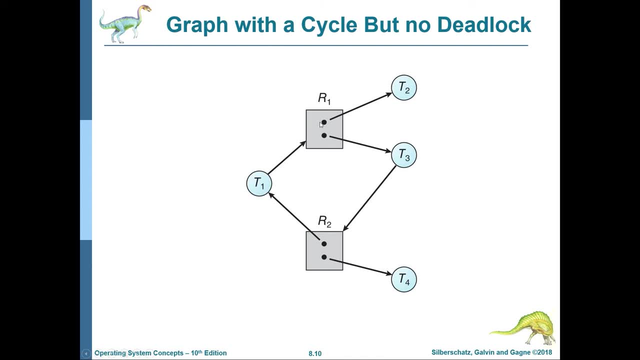 kinds of resource. So R1 is a kind of resource. only one dot should be there. R2 is a kind of resource, it is a resource type. only one dot should be there If all the resources only have one dot and after that also there. 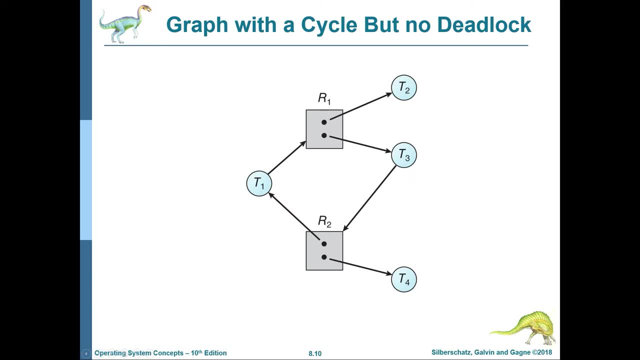 is a cycle, that means there is a deadlock in the system. But if there is at least one resource type that has more than one- so there are two dots inside that rectangle and the graph also has a cycle- then there is no guarantee that that represents a deadlock. We have to see 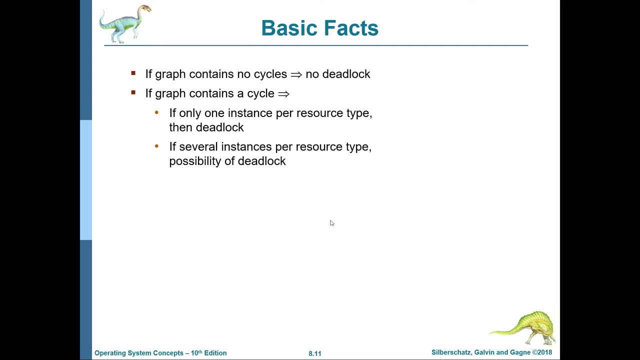 on a case by case basis. if that is the situation, whether it is a deadlock or not. So if there is no cycle, there is no deadlock. If only one instance per resource type for all resource types and there is a cycle, then there is a deadlock. But if there is, 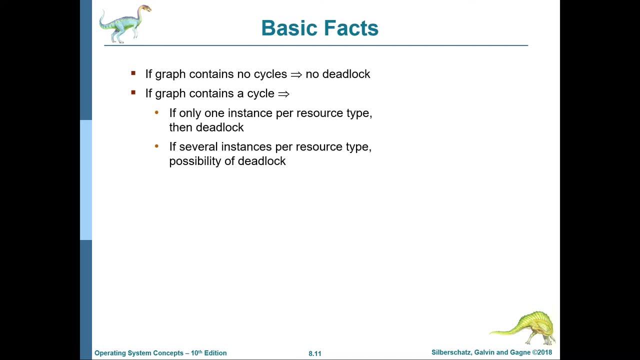 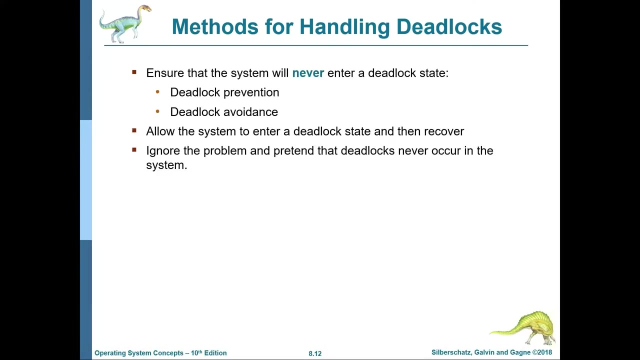 more than one instances for one or more resource types in a graph and there is a cycle, then there is a possibility of a deadlock, but it is not guaranteed that it must be a deadlock. So now we will look at methods for handling deadlocks So we can ensure that the system 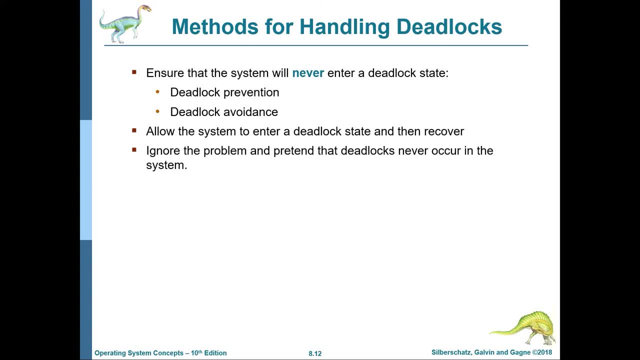 will never enter a deadlock. So we can do it using two ways. We can try to prevent deadlocks and we can try to avoid deadlocks. Prevention is the stronger case, but it is not easy to always prevent deadlocks. You can avoid deadlocks, but you need. 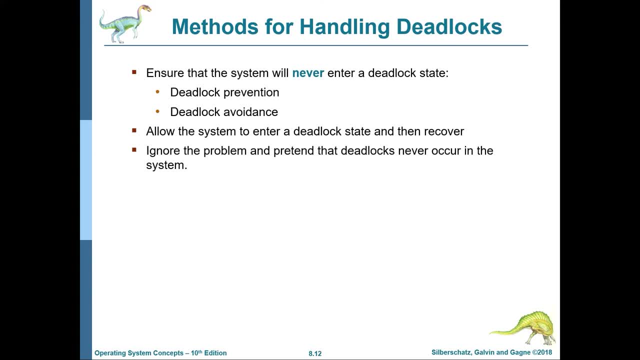 more information about the system to be able to avoid deadlocks well in advance. We will look at both the situations in a great amount of detail in the next few slides. We can also allow the system to enter a deadlocked state and then learn to recover from. 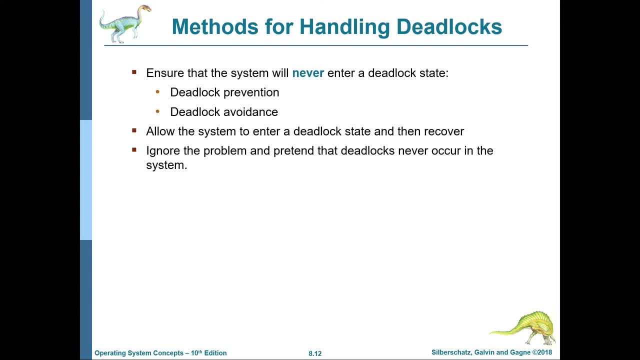 it. So even if we don't prevent or avoid deadlocks, we can let the system enter a deadlocked state and then we can recover from it gracefully, Or we can just ignore the problem and always pretend that deadlocks never happen in the system. 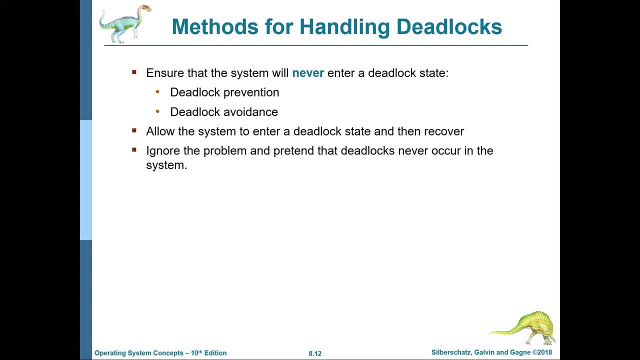 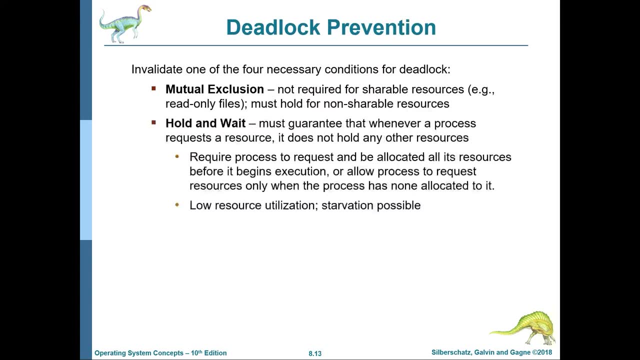 so that we don't have to prevent, avoid or recover from deadlocks. That is the worst idea, but some operating systems do that. So, as I said before, there are four necessary conditions for a deadlock to happen, and we learned they were: mutual exclusion, hold and wait. 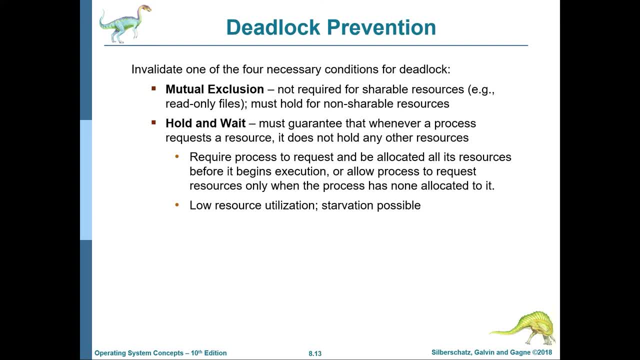 no preemption and circular wait And, as I said, when all four of these conditions are true simultaneously at the same time, then deadlocks are possible. It does not mean that deadlocks have happened. That means that deadlocks might happen. It is a perfect recipe for deadlocks. 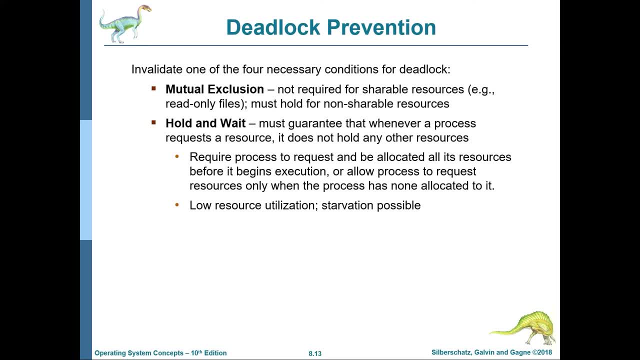 to happen. So that means, by logic, if one or more than one of these four things don't happen, then a deadlock can always be prevented. So let's look at the first one: Mutual exclusion. This relates to the shareability of a resource. 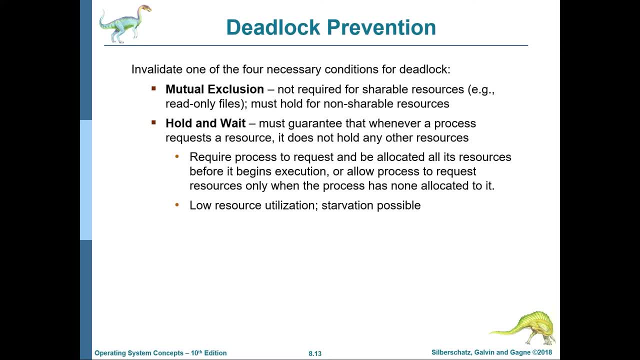 If a resource is not shareable, then it is a mutually exclusive resource. That means only one process can be using it at any one point of time. So if we make sure this never happens, that means all resources in the system are shareable. then deadlocks will never. 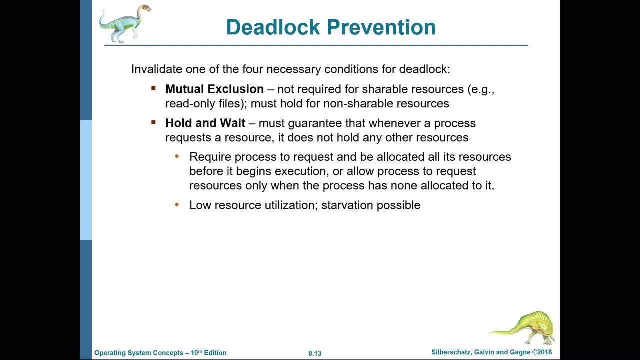 happen because processes will never have to wait for resources. Whenever they want a resource, they can always go and get a hold of it. One example might be: read only files because nobody is actively changing that is writing to such files. processes who want to read from it can do that. 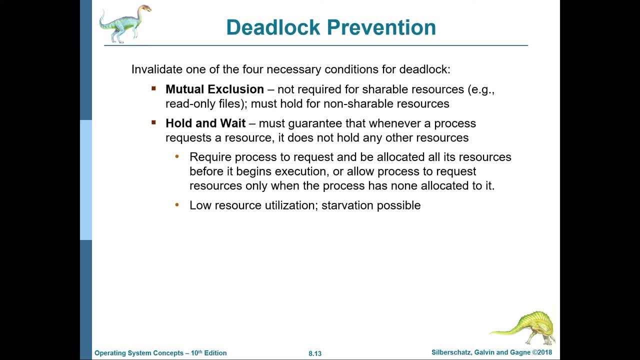 concurrently at the same time and that will not cause any problems. But like read only files, other resources cannot be shareable and, as I said before, for example, a printer cannot be shareable. you have to serialize access to a printer, as in let processes use the printer serially. 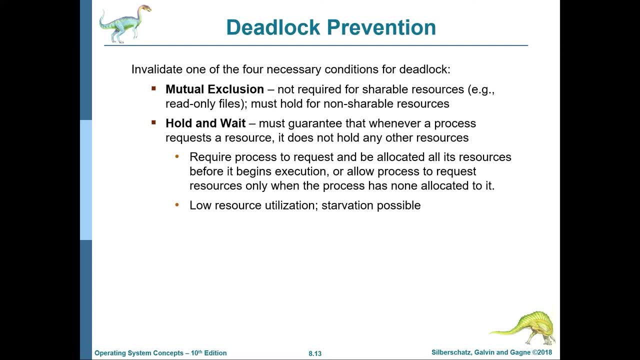 one after the other, not at the same time. Let's move on to hold and wait. If you remember, hold and wait was about holding a few resources and then waiting for the rest of the resources to arrive. Now, how to make sure this does not happen? There are two. 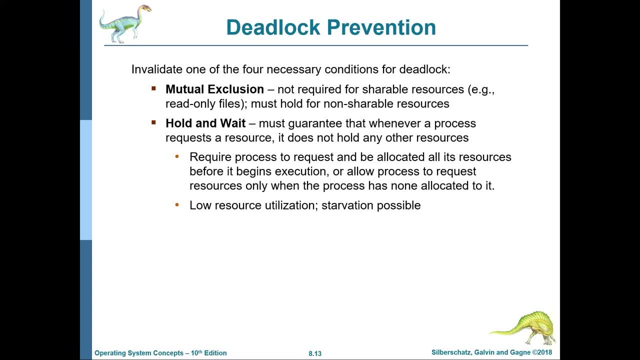 ways. First of all, a process has to request all the resources it needs at the beginning, and then it needs to make sure that it gets all of them at the beginning. If it does not get any one or more than one of them, it cannot begin. It has. 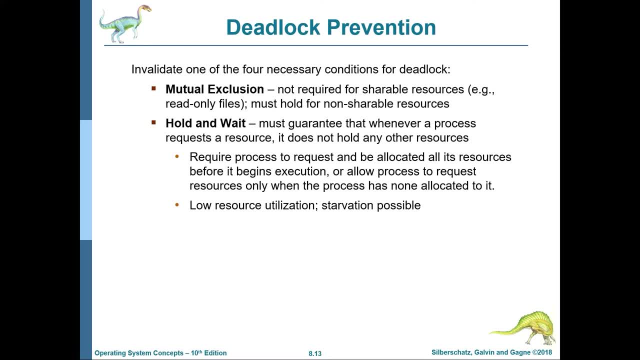 to make sure it gets everything at get go. There is another way to do it. let's just say a process needs three resources: A CD-ROM drive, a hard drive and a printer. If it can only get the CD-ROM drive and the hard drive and not the printer. 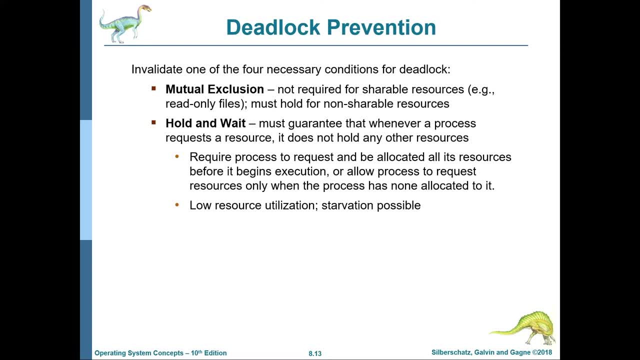 then it has to do some partial work with just the two of them, So it can, for example, copy the files from the CD-ROM drive to the hard drive and then, once it is done, it has to return the CD-ROM drive and the hard drive back to the system and 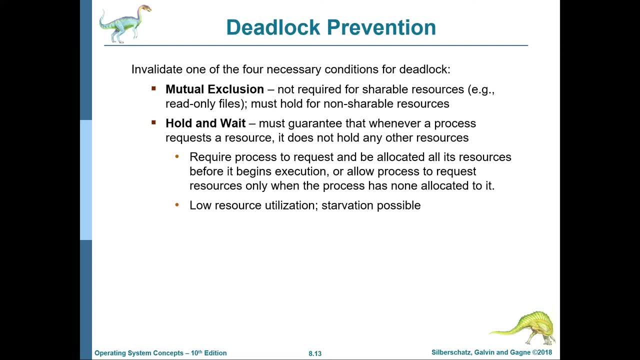 then it has to request for the hard drive and the printer. When the hard drive and the printer are given to it, it is going to read the file from the hard drive and print the document and then give the hard drive and the printer back to the system. 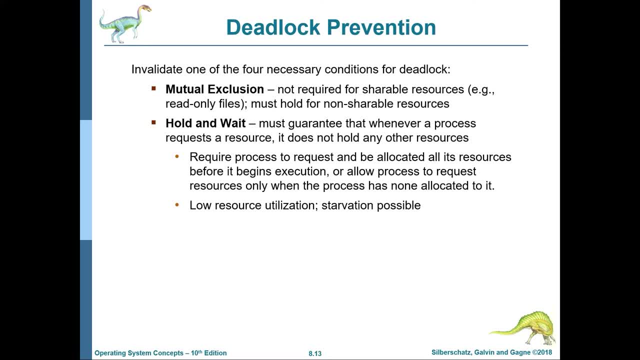 So it has to, at the midpoint, give the CD-ROM and the hard drive back to the system. It cannot just keep holding on to them and then say, okay, I am done with the CD-ROM and the hard drive. now you give me the printer also. No, You take whatever. 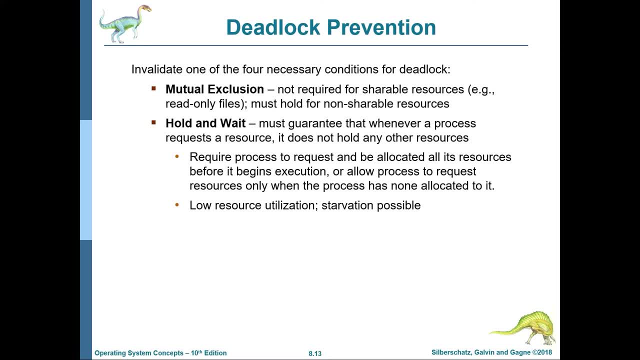 you want, give it back, and then you ask for a fresh set of resources. If we ensure this happens, then hold and wait will never happen and deadlocks can be prevented. The problems of this approach is low resource utilization. For example, if it grabs. 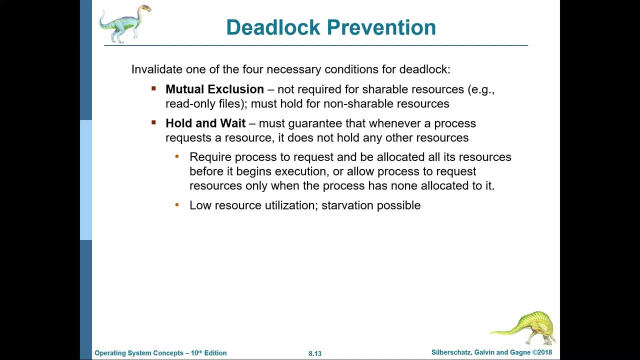 the CD-ROM drive, the hard disk drive and the printer at the beginning, even if it is not using the printer in the first few minutes of the operation where it is copying the data from the CD-ROM drive to the hard drive, the printer is just lying idle. 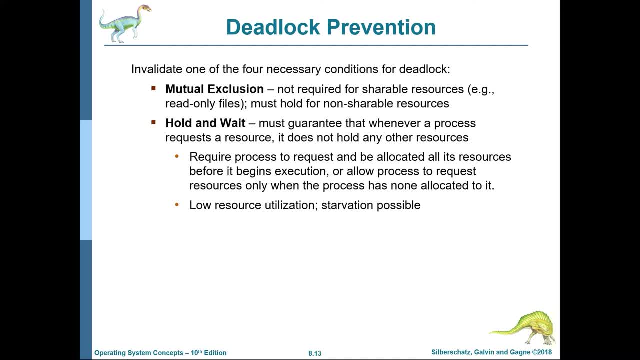 Now, that is a classic example of low resource utilization. Also, starvation is possible. Let us just say it takes hours for it to copy data from the CD-ROM drive to the hard disk, and then the printer is just sitting idle with the process. Now that can starve. 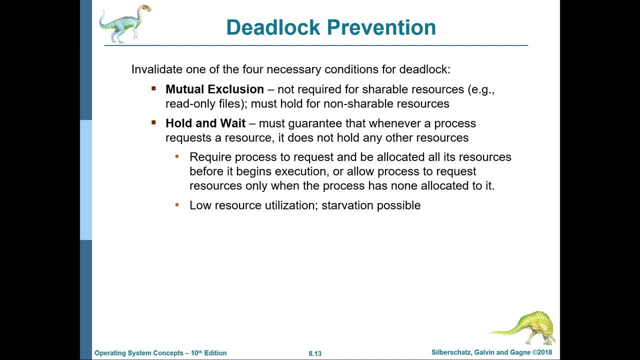 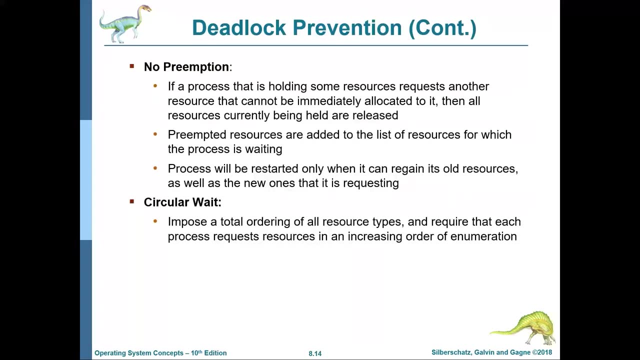 other processes, though at some point it will return it back, but it can starve other processes. So low resource utilization and starvation are the two problems of not doing hold and wait. Then we can make sure that preemption can happen, because no preemption is one of the conditions. 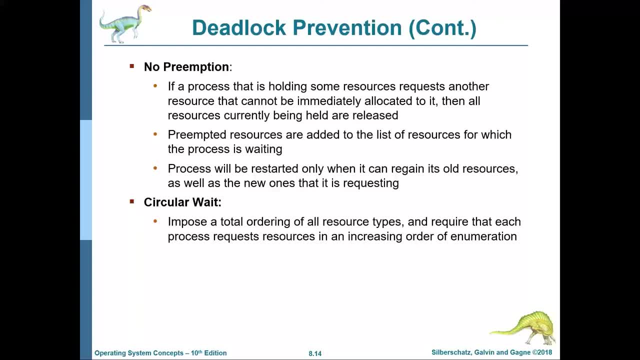 for deadlock If you double negate it, then if we can let preemption to happen, then deadlocks can be prevented. Now, if a process that is holding some resources requests another resource that cannot be given to it, then everything that it has can be taken away from it by the 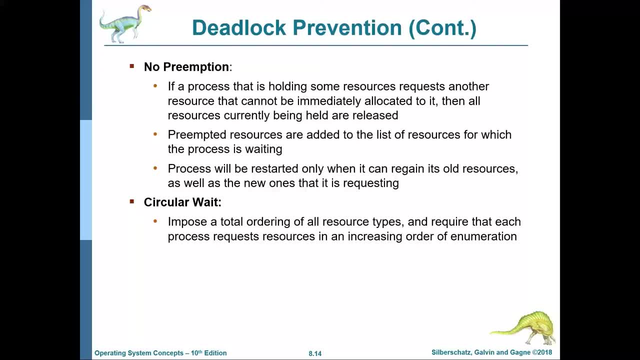 operating system. Again, we will use the same example. The process had the CD-ROM drive and the hard drive, but the printer was not there with it. So when it was requesting for the printer, the operating system can come back and tell it that look, I cannot give you the printer. 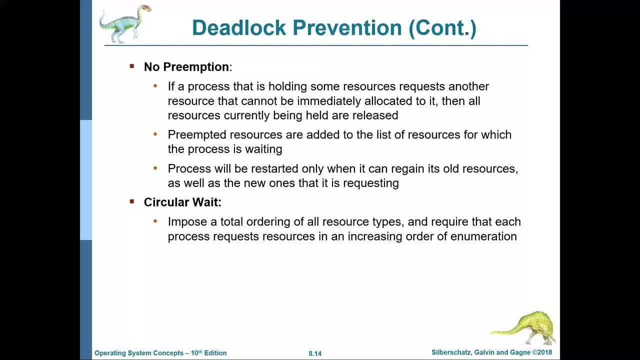 so you have to give the CD-ROM drive and the hard disk back to me, And whenever these things are all available at the same time, I will give it to you. But for now I am going to preempt the CD-ROM and hard drive, Even if you have them. 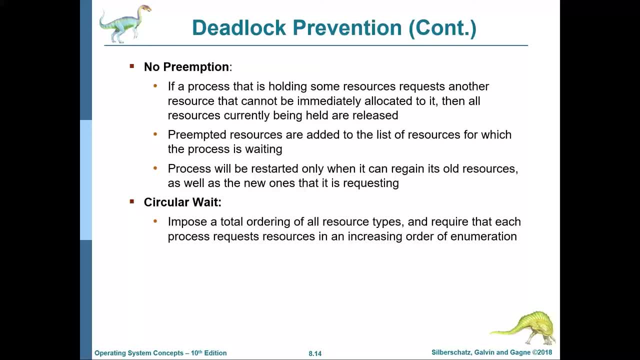 with you. you are going to give it back to me. Another approach could be: now the process has the CD-ROM and the hard drive, but not the printer. but if the printer is with some process, that is again waiting on something else, So it is not able to. 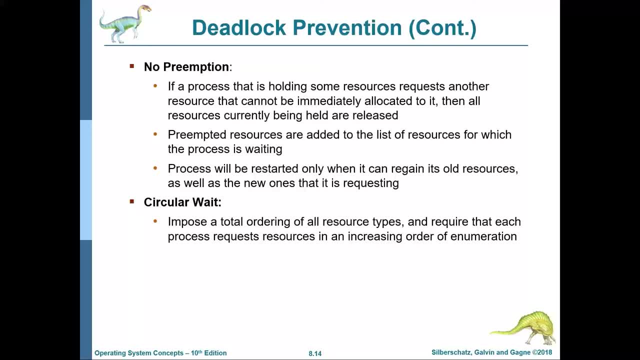 use the printer right now, but it is also waiting for some other resources. then the operating system can go and steal the printer from that second process and say: okay, I am going to take the printer from you because you are anyway waiting for something else which you don't have. 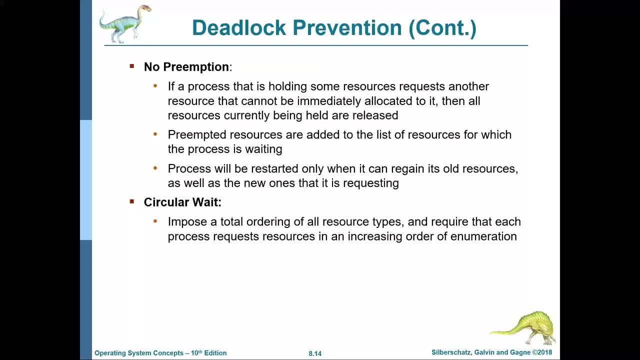 in the meantime, I can assign the printer to another process which really needs it, and whenever the other resource that you are waiting for is available and the first process has given the printer back, I am going to assign it to you. till then, you can wait. So that is. 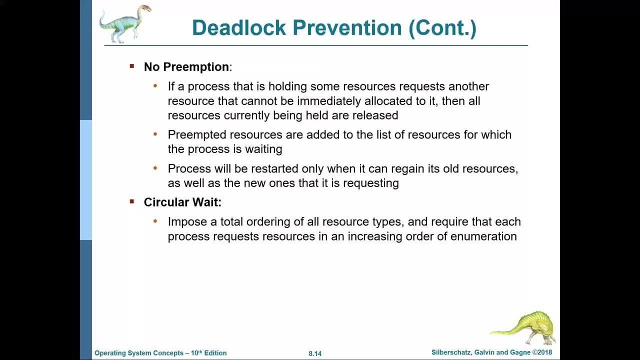 also another kind of preemption. If preemption can be done, then deadlocks can be prevented. Circular wait was another condition for deadlocks to happen, and if we not let circular wait ever happen, then deadlocks can be prevented. So what was circular wait again, 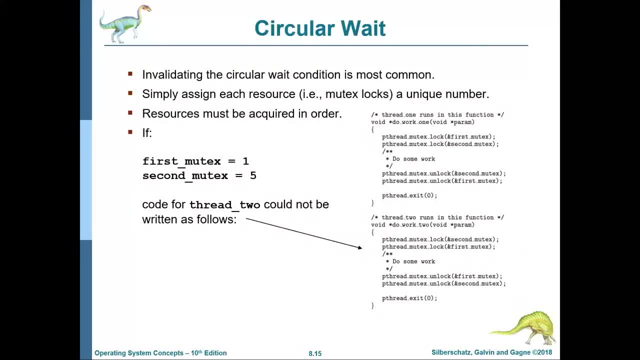 Circular wait was about if we could number or order the processes in such a way that a process earlier in the list depends on something that someone just after that process is holding on to, like P0 is waiting on something that P1 has, P1 is waiting on something that P2 has. 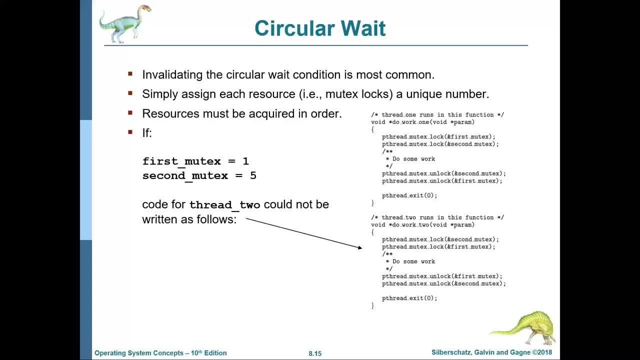 so on and so forth. then circular wait can happen, Right, But it can be prevented by numbering the resources in a certain order. So we can say R1 is the set of all CD ROM drives, R5 is the set of all hard drives and 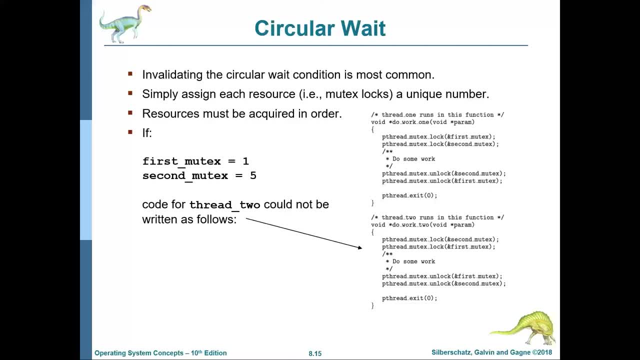 R15 is the set of all printers and we can put a rule on the processes and we can ask them. you can only order the resources in increasing order of their number. so you have to first make sure that you get R1. so you have to first make sure. 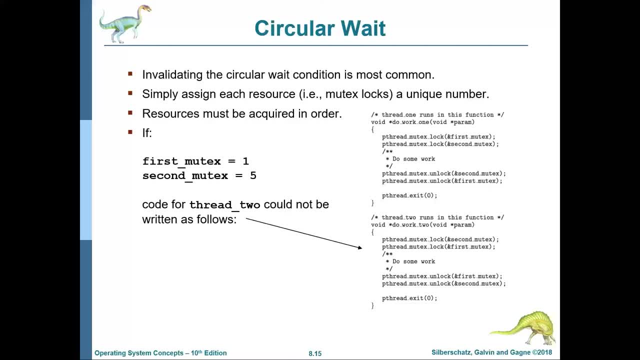 that you get a CD ROM. only after you get a CD ROM can you go ahead and ask for a hard disk. Once you have a hard disk, then you can go ahead and ask for a printer. so you have to request the resources in increasing order of their resource number. 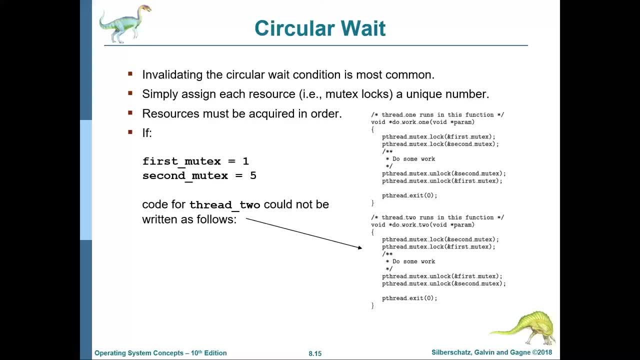 If all the processes in the system do that and the operating system actually ensures that the processes are following this discipline, then deadlocks will not happen, because circular wait is not going to happen. Let's go back to our semaphore example, which is there on the screen right now. 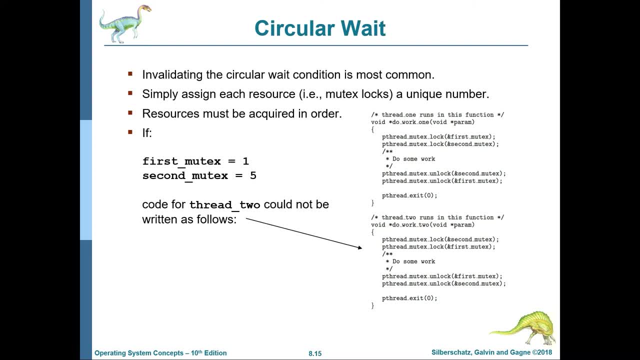 If you remember, P1 used to first wait on S1 and then wait on S2, but P2 was first waiting on S2 and then waiting on S1.. What if we could number S1, the first mutex or the first semaphore, right here: semaphores and mutex. 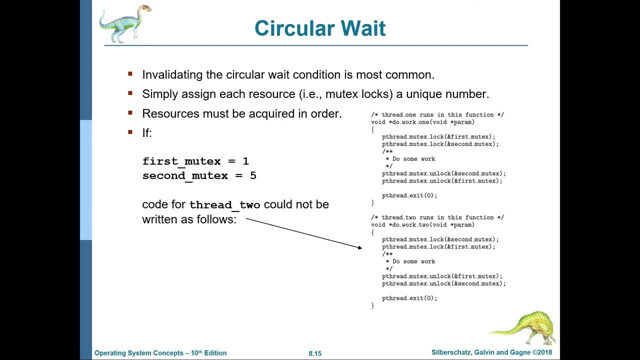 are actually working in the same manner. they basically solve the same problem here as locks. whether it is a mutex or a semaphore does not matter so much in the context of this chapter. So if we can make the first lock the mutex or the semaphore and give it the 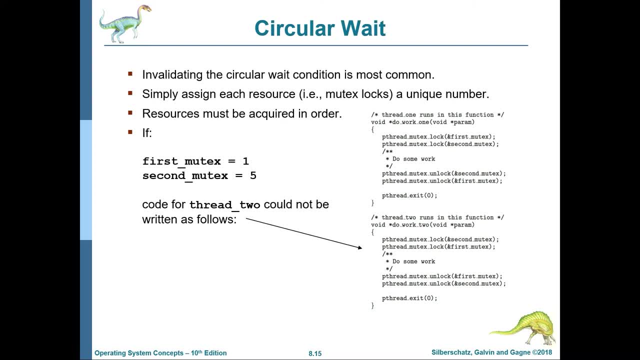 resource number of 1 and the second mutex the resource number of 5, and then make sure that both the threads P1 and P2 access the locks in that order, that is, they go for the first mutex first and then they go for the second mutex later. 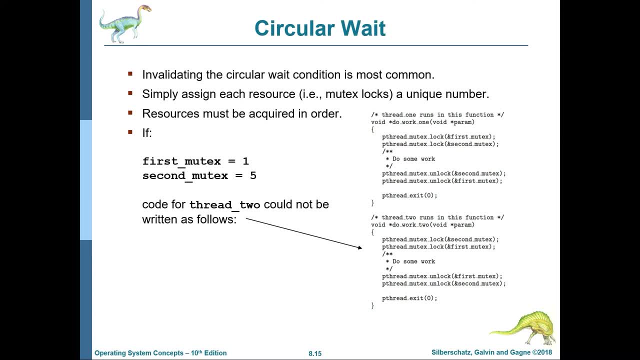 because the first mutex's number is 1 and the second mutex's number is 5.. So the first process was anyway doing the correct thing, because it was asking the lock on the first one and then on the second one, and then it was unlocking the second. 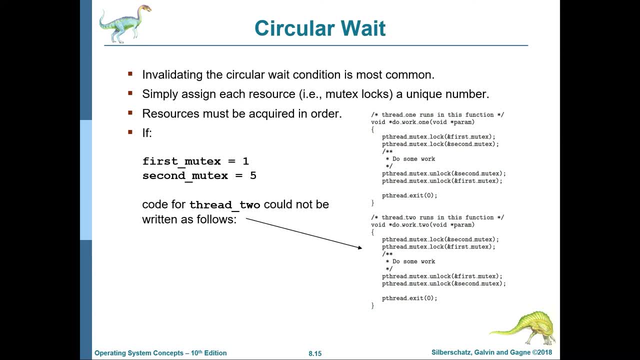 one first and then unlocking the first one second. right. so it was going for the first lock and then the second lock afterwards. but the second process attempts to lock the second mutex first and the first mutex second. now this is where the deadlock was happening, right? but if we put this rule, 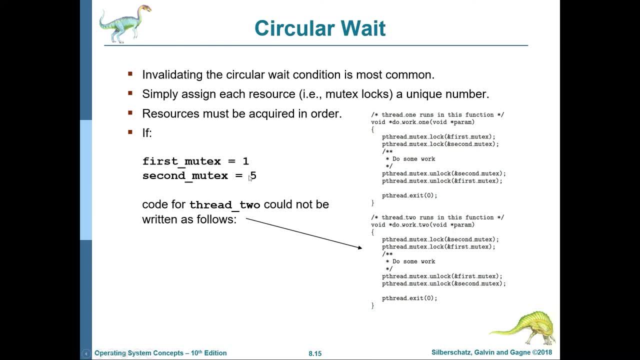 that the second process has to go for the lower numbered mutex first and then the higher numbered mutex second. then a deadlock cannot happen, right? so the code for the second process will kind of look like this: so it will get a lock on the first mutex first and 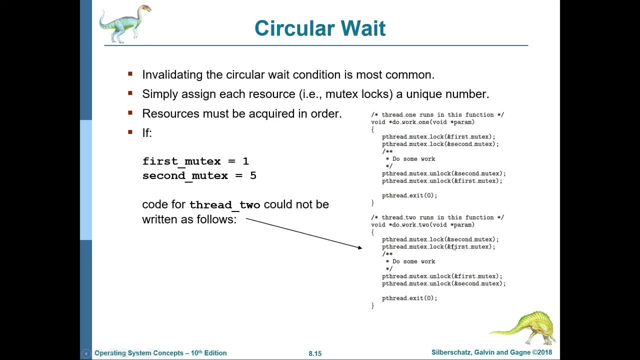 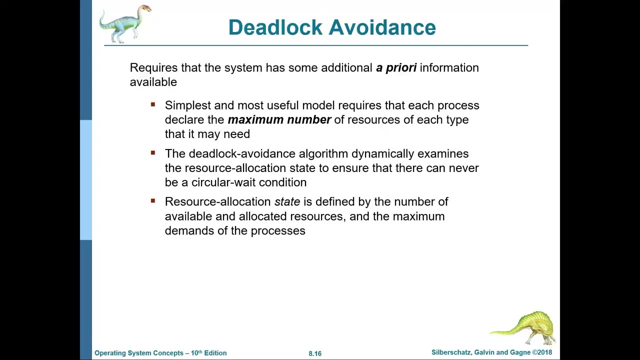 the second, mutex second, and then both the processes will never enter a deadlocked state. can you see why? if you cannot see, why pause the video and think about it now. that was all about deadlock prevention, and deadlock prevention, as you could see, is not very easy to carry out. 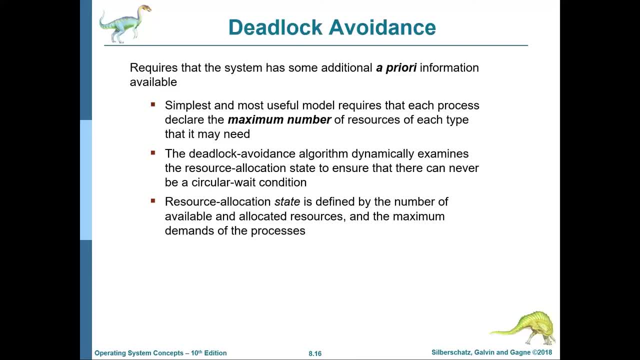 mutual exclusion is very difficult to get rid of because you cannot make all the resources shareable. hold and wait is also very, very tough because you cannot make sure that processes always get all the resources at the beginning. but even if they do, it can result in low. 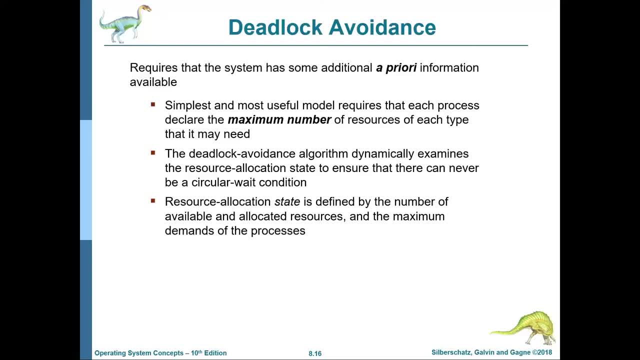 resource utilization and starvation. no, preemption is also difficult to do because you are stealing resources from processes midway- and many things cannot just work that way- and ensuring that the resources are numbered from lower numbers to higher numbers and the processes have to request them in the increasing order of the resource. 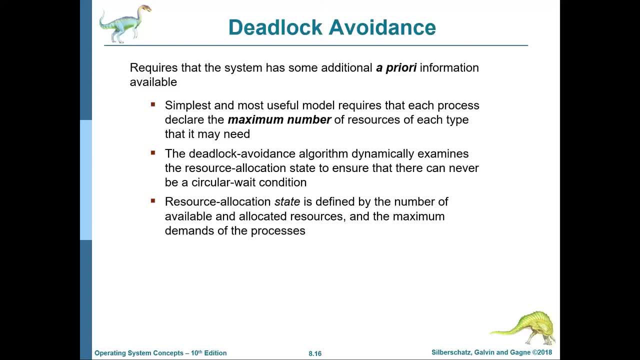 number is also not feasible because it is up to the processes to ensure that they are following that discipline. not all resources are handled by the operating system. if it is resources like cd-rom drives, hard drives and printers, then the operating system can enforce that discipline. but if it is, 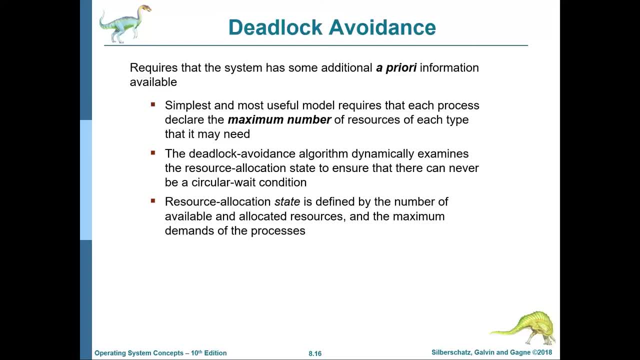 semaphores and mutexes. it is all about how programmers write their code, as we just saw in the case of the two processes that we discussed in the previous slide. if the second process still chooses to use the second mutex first and the first mutex second, deadlocks. 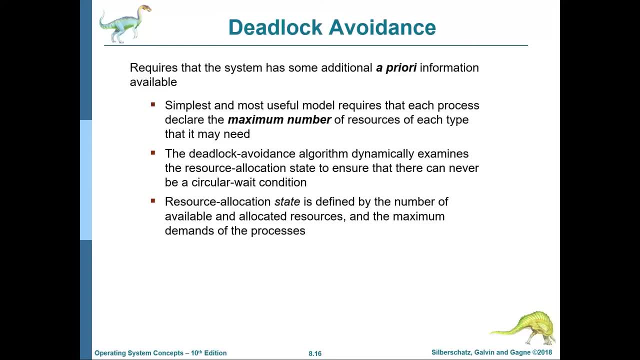 can still happen, and it is very difficult to kind of get that kind of discipline in all the programs that a computer has to run. so deadlock prevention is not always easy, though it is a stronger case of preventing deadlocks, so ensuring that deadlocks never happen, because if you can, 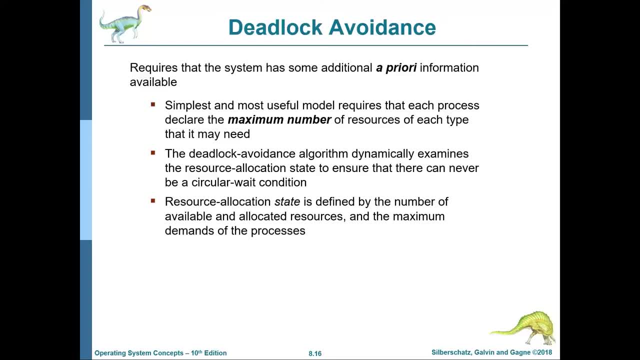 ensure one of them don't happen, then deadlocks can never happen. but it is hard to do that, so we will look at deadlock avoidance. in deadlock avoidance, the operating system needs to have some a priori- that is, prior- information about processes, one of the most important pieces. 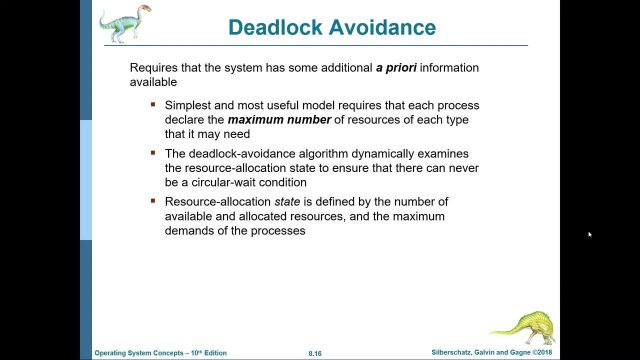 of information that an operating system needs to know about a process is the maximum amount of resources the process might request in the future. I am not trying to say that the processes have already obtained that maximum. they are probably operating at a number that is lower than that. 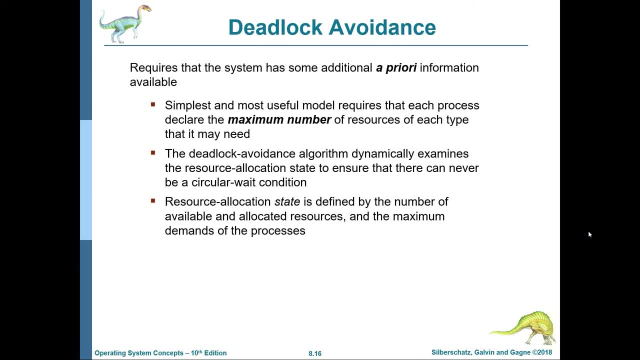 maximum at this point of time, but the operating system must know, in order to avoid deadlocks in the future, what is the maximum amount of resources processes might want to obtain. with that kind of information available, the operating system might employ deadlock avoidance algorithms that will dynamically examine. 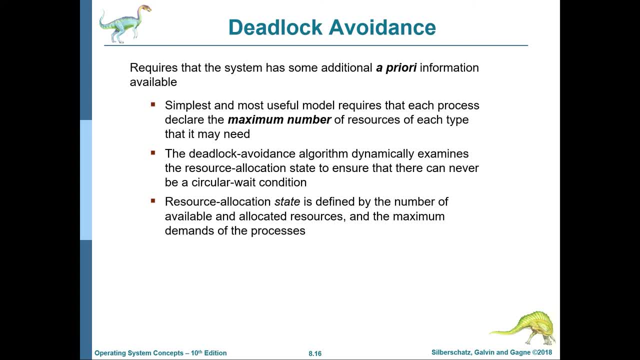 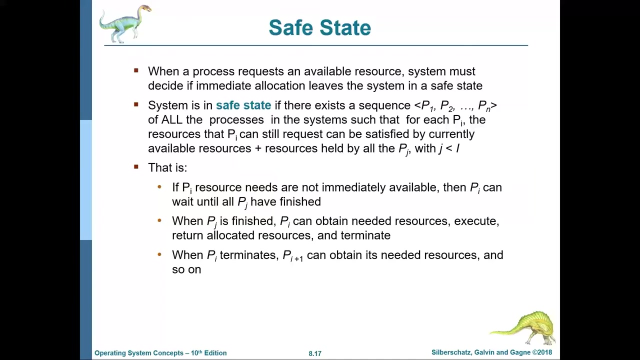 the resource allocation state to ensure that the circular weight condition that we have studied before never happens. the resource allocation state is defined by the number of available and allocated resources and the maximum demands of the processes. so lets study about what is a safe state. lets assume that 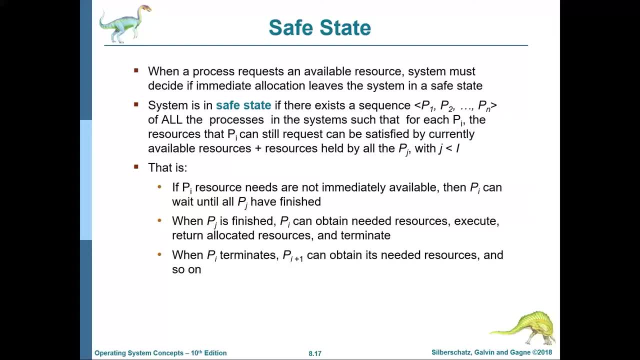 the system is already in a safe state, and when a request for resources comes in, the system must decide if it needs to satisfy the request while making sure that the state remains safe. it should never allocate resources to the request and in turn make the system unsafe. so that is the. 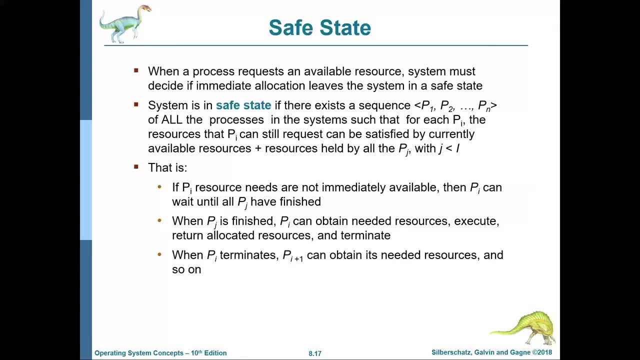 vague idea about a safe state. for a formal definition, safe state is a state in which we can order the processes P1, P2 up to Pn in such a way that a process PI can complete its work by requesting resources and those resources can be satisfied by whatever. 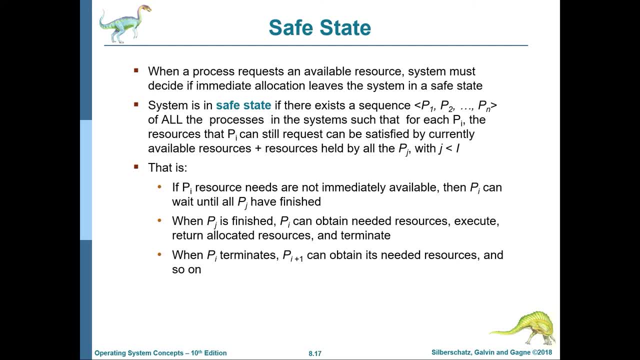 is available in the system, that is, whatever is free and whatever can come back after all the processes whose numbers are less than i and when they finish right. so, for example, if P2 makes a request, then if that request can be satisfied by whatever the operating system already has with it. 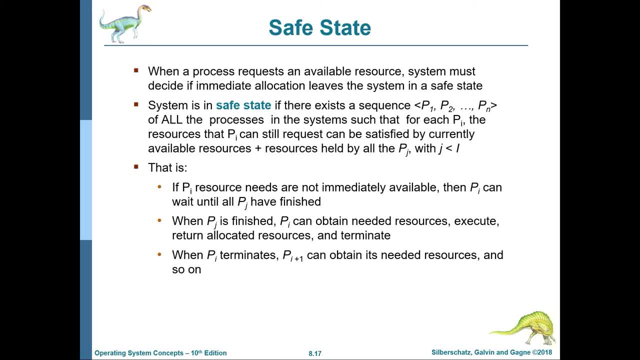 and whatever it can get back after P1 finishes execution. if P3 makes a request, then if that request can be satisfied by whatever free resources the operating system has, plus whatever can come back after both P1 and P2 finish execution, so on and so forth. 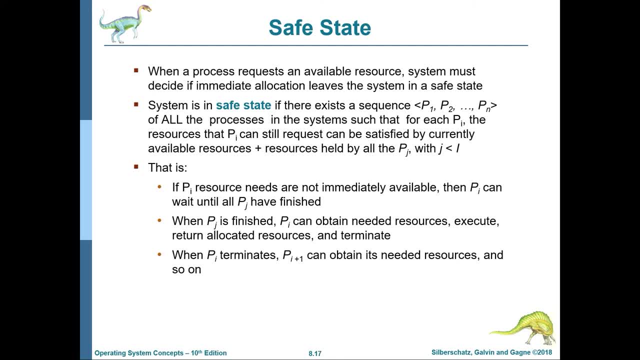 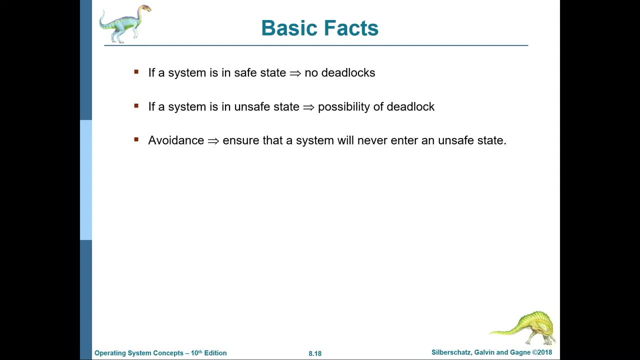 if we can arrange the processes in that way, then the system is said to be in a safe state. again, let's come back to some basic facts. if a system is in a safe state, then no deadlocks can happen. if a system is in an unsafe state, 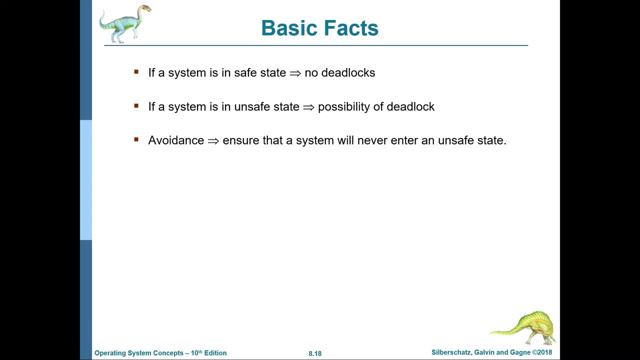 then there is a possibility of deadlock. avoidance means ensure that a system will never enter an unsafe state. if the system always stays in a safe state, then deadlocks will never happen. if the system goes into an unsafe state, then there is a possibility of deadlock. i am not trying to say 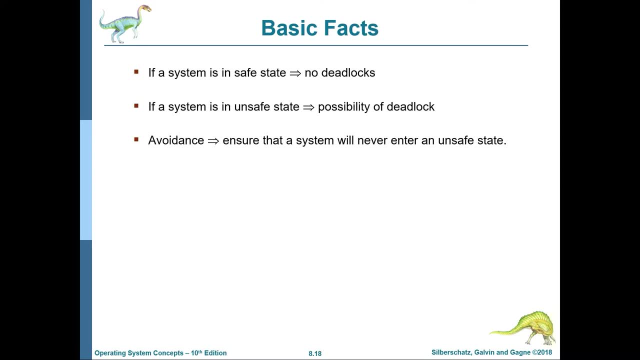 that deadlocks will always happen in an unsafe state. but the possibility is always there in an unsafe state for deadlocks to happen. in a safe state, there is a guarantee that deadlocks will never happen. and what is a safe state, if the processes can be arranged from? 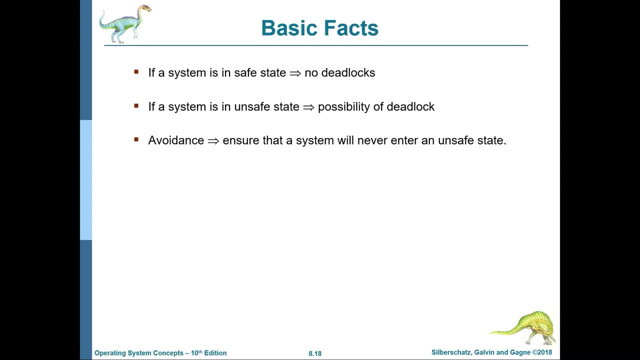 p1 till pn in such a way that pi, the process, pi's request can be satisfied by the operating system with whatever it has and from whatever it can reclaim, whatever it can get back from all the processes less than i. it's the same thing over here. so this is the safe state and this is the 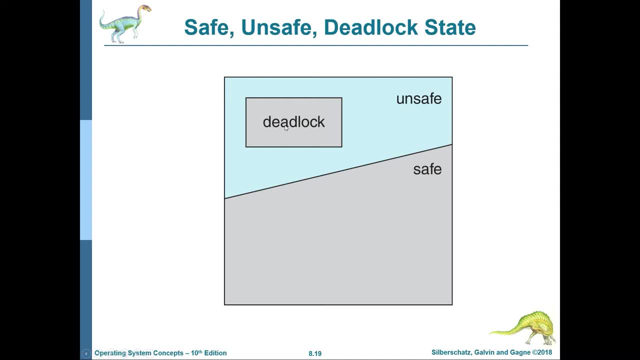 unsafe state and deadlocks can happen in this area and, as you can see, it is not the entirety of the unsafe state. so once you are in the unsafe territory, then deadlocks might happen. there is a possibility of deadlocks from happening, but in the safe state deadlocks can never happen. so it is a job of the 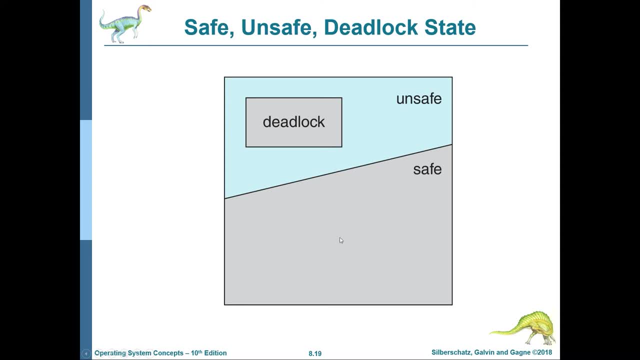 avoidance algorithm to always keep the system in a safe state. now there are two kinds of algorithms. if only single instances are there for resource types- if you remember those rectangle nodes that we used to talk about, and those rectangle nodes used to stand for resources, and if there was only a single dot inside them, that meant that only. 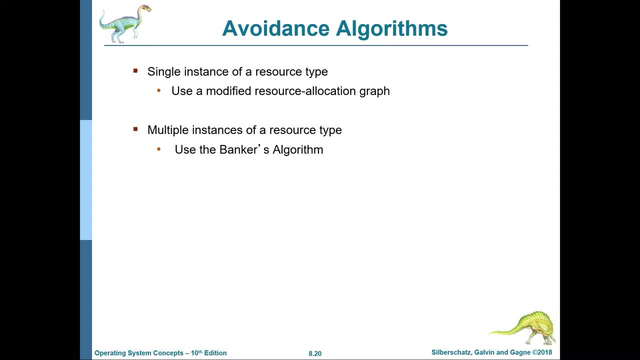 one instance per resource type is present for that resource type, and if there was only one instance for that resource type, if more than one dots were there, that meant more than one instances are there for that resource type. so if only single instances are there, we can use a modified resource allocation. 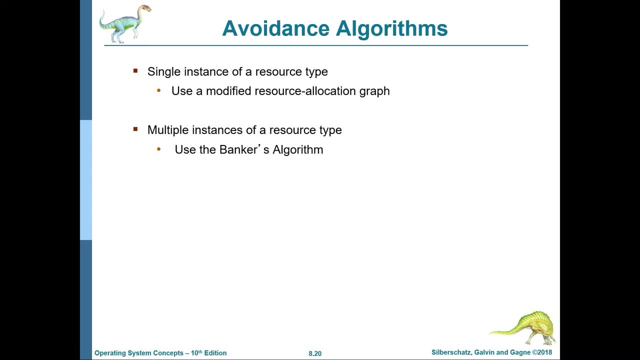 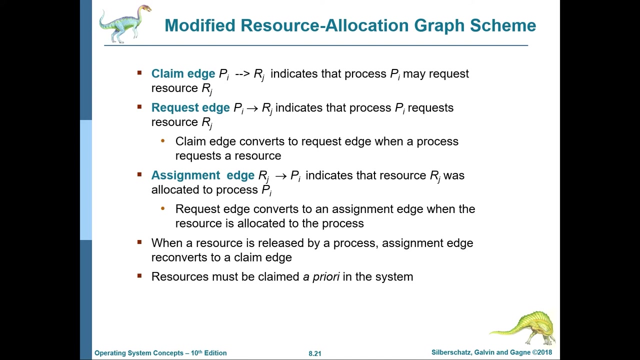 graph, look for cycles and figure out if the system is safe or not. now, if multiple instances of a resource type are there, then we can use the bankers algorithm and we will look at how that works later. now. the modified resource allocation graph scheme is almost similar to our previous original. 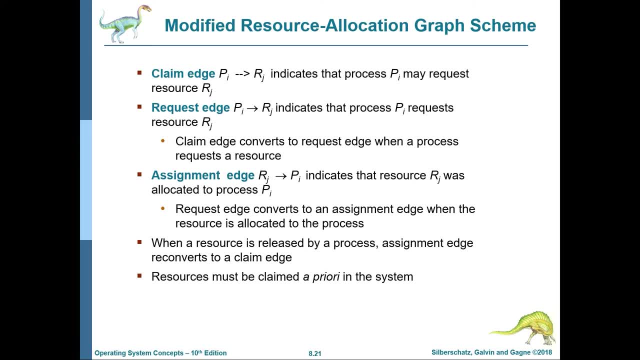 resource allocation graph. the new kind of edge is introduced here. it is a claim edge. it always goes from a process to a resource and it says that that the process may request the resource in the future. right not now, There is a possibility that the process might request that resource and the claim edges. 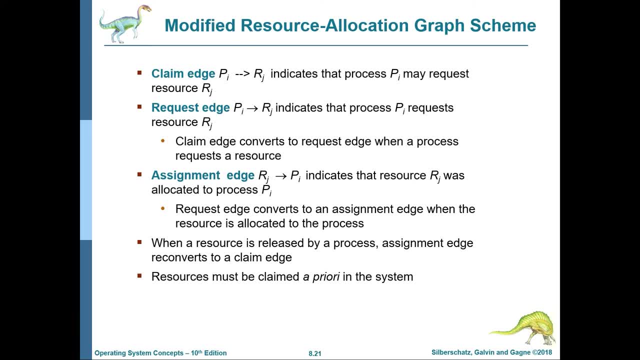 are always dotted. they are not bold lines, the dotted lines. they start on a process. they point towards the resource. Now, the request edge is the same old request edge. it always points from a process to a request and claim edges become request edges when a process is actually making the request. 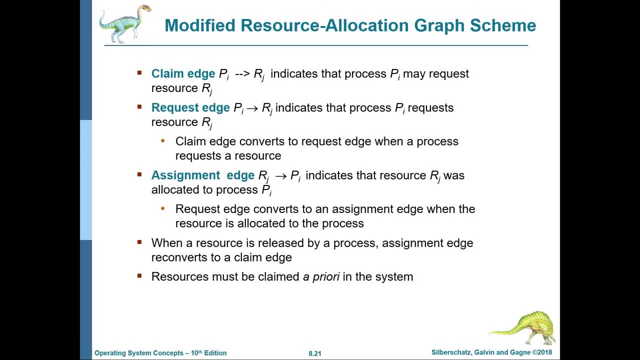 So claim edges can turn into request edges and the direction will remain the same. they will always point from a process to a resource, and assignment edges are again the same thing. They always point from a resource to a process, and request edges will turn into assignment edges when the OS approves the request and says: okay, now you can have the resource and 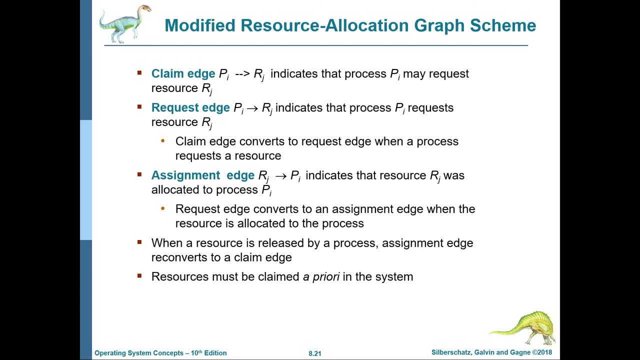 then the request edge will become an assignment edge. A thing about the, The avoidance algorithm that we are studying here, is that resources must be claimed a priori in the system. That means the resources must be claimed by the processes beforehand. The process has to kind of declare to the OS that I might need these many things in. 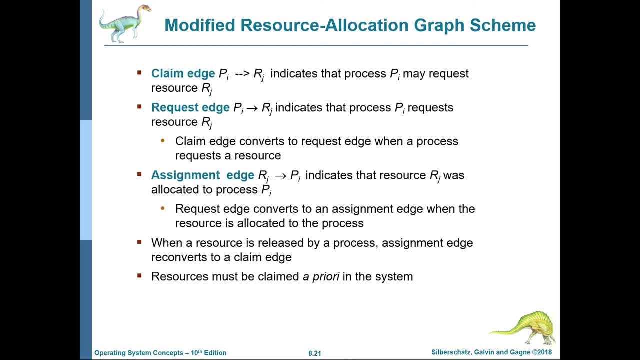 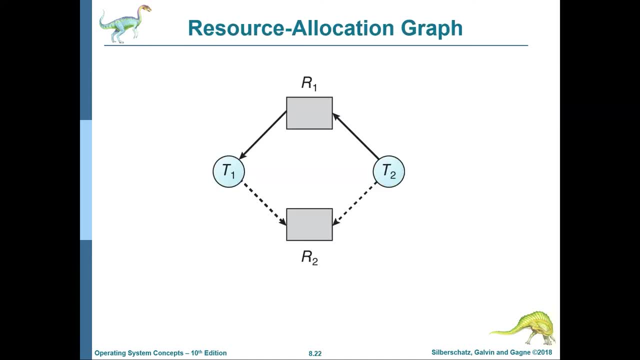 the future, though I am not currently requesting them, but I might need them in the future So that information processes have to inform the operating system. This is an example of it Allocation graph. here you can see that T1 has a claim over R2 and T2 also has a claim. 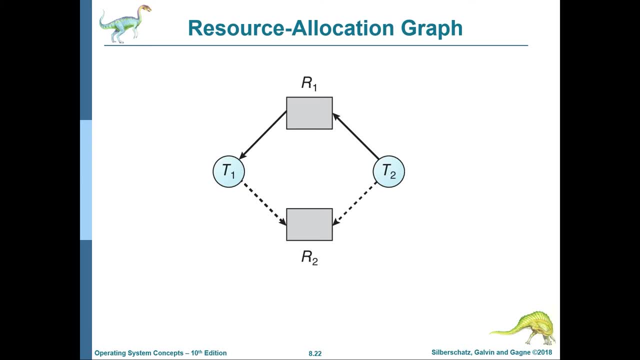 over R2, because we see two dotted arrows, one starting from T1 pointing towards R2, and another also starting from T2 and pointing towards R2.. Now there is a request edge from T2 to R1. that means T2 has made a request to the operating. 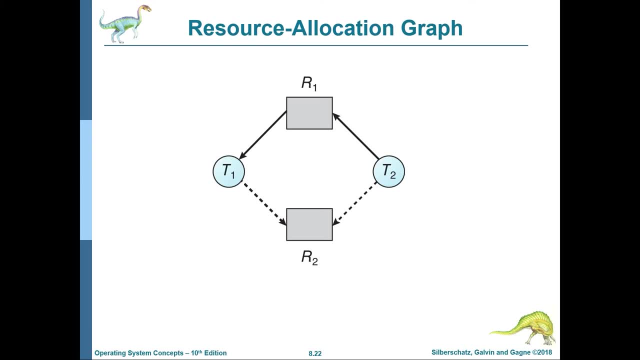 system. to get instance of R1, and there is an assignment edge from R1 to T1. that means R1 is currently assigned to T1.. It is currently allocated to T1.. Now let's just say we satisfy the request of T2 over R2.. 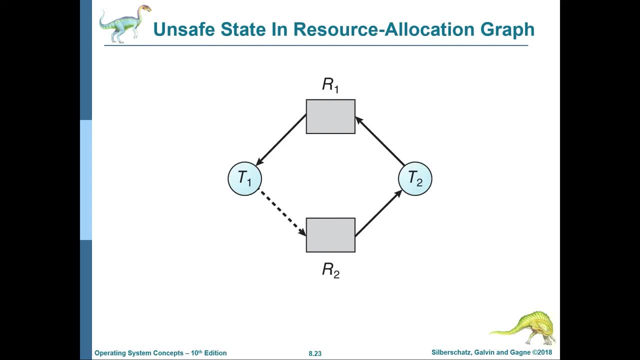 Now, T2 had a claim over R2 previously. Let's just say that turns into a request and the operating system allocates that resource to T2.. Then what happens? there is the dotted line from T2 to R2 becomes a request edge from T2. 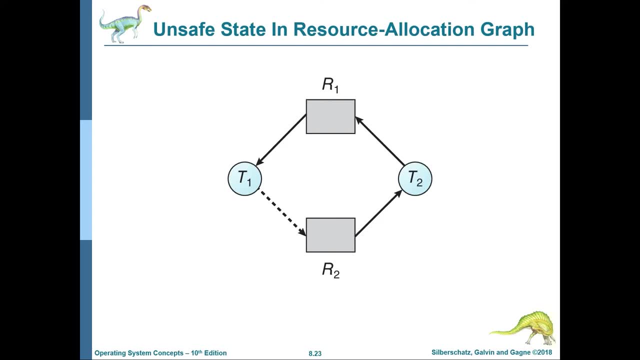 to R2 and the OS grants it and then that becomes an assignment edge from R2 to T2.. So can you see a cycle? Yes, we can see a cycle. that means this is an unsafe state and a deadlock might happen. Can you tell me when a deadlock might happen? 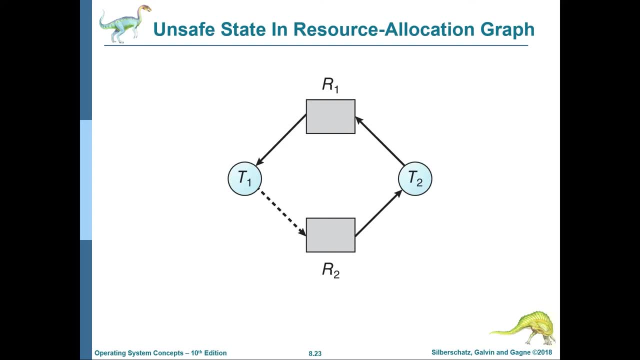 Just imagine T1 makes a request over R2 right now. Then what would happen? The operating system will give that resource, or well, it cannot give that resource. It will just turn the claim edge from T1 to R2 to a request edge from T1 to R2, and then 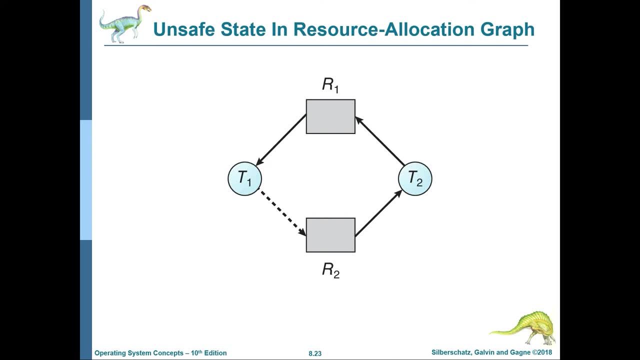 there is a cycle in the graph and then it's a deadlock. It's a clear deadlock because T2 is waiting on R1, that is currently assigned to T1,. T1 is waiting on R2.. Which is currently assigned to T2.. 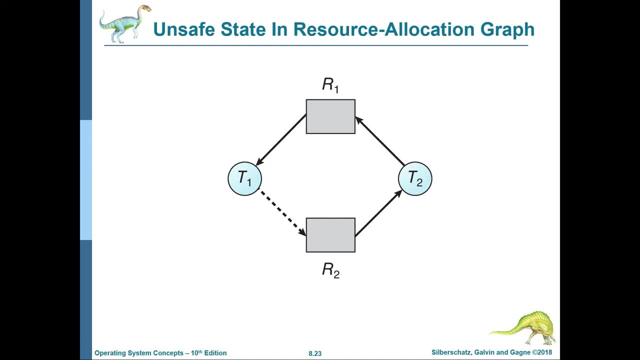 So the fact that we actually allocated R2 to T2 and introduced a cycle in the modified resource allocation graph we made it unsafe. That does not mean that a deadlock has already happened as long as T1 has not made a request on R2 yet. 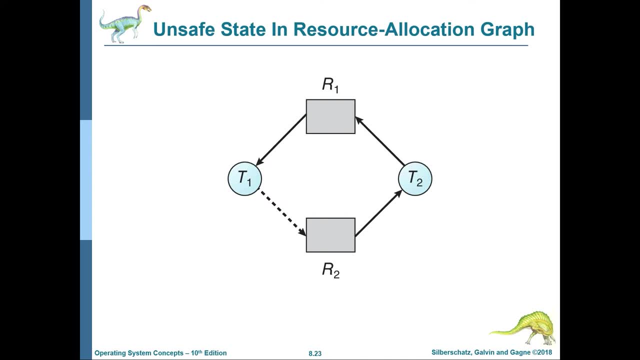 The system is still fine, There is no deadlock, but it has already become unsafe because the moment T1 makes a request on R2. And that cannot be allocated because it has been given to T2, then a deadlock happens And the beginning of all of this is- let's go back to the previous slide- is this graph: 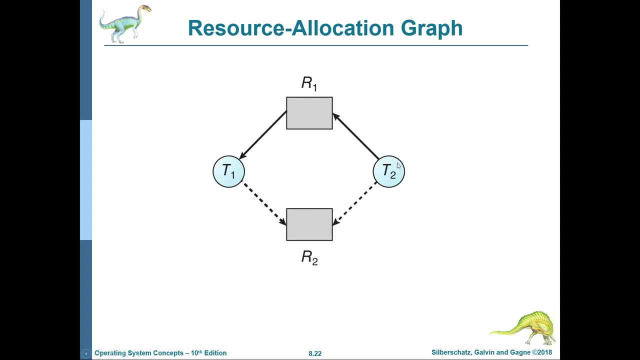 was fine. there were no cycles. The moment T2 made a request for R2. then this arrow kind of turned its direction and this happened, And now you can see a cycle in the modified resource allocation graph and that is where the system went from a safe state to an unsafe state. So you can use this. 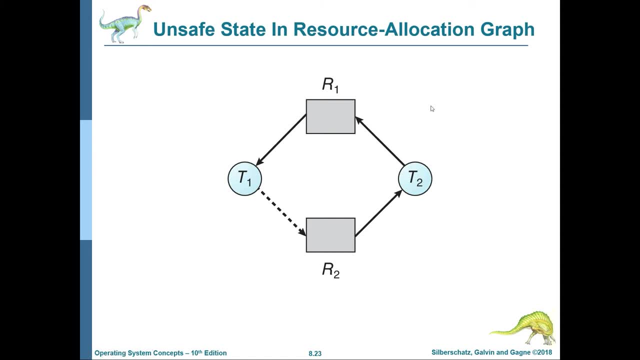 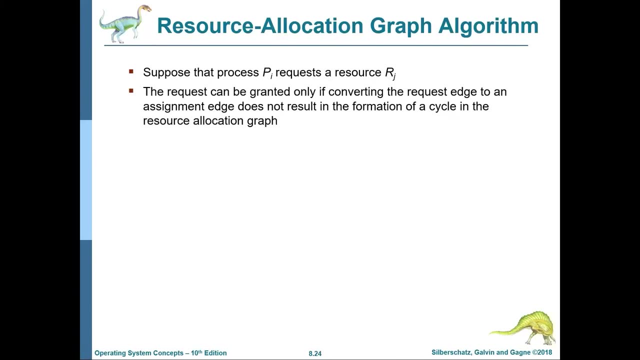 algorithm to figure out if the state of the system is unsafe or not, if only single instances per resource types are there. So this slide kind of talks about the same thing that we already discussed. If you have a modified resource allocation graph and a process, PI requests a. 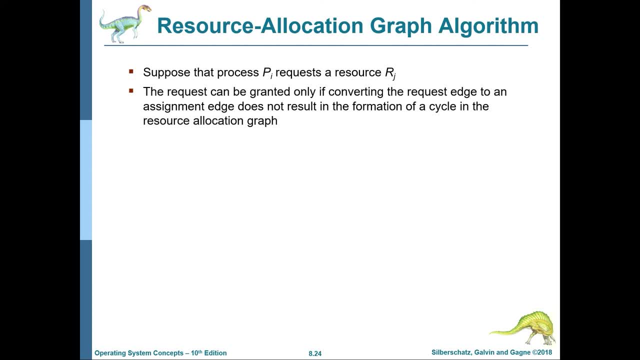 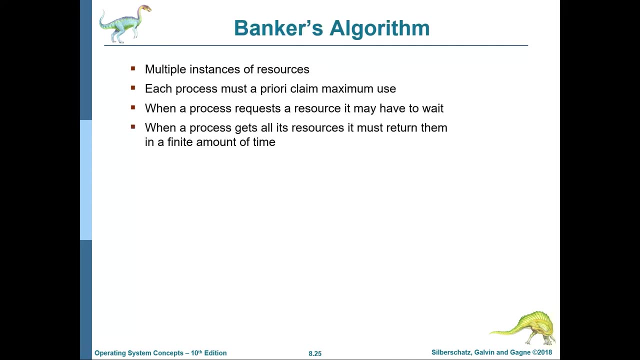 resource RJ. the request should only be granted if a cycle does not get introduced into the graph, because if a cycle gets introduced, then the system will go from a safe state to an unsafe state and possibility of a deadlock will arise. Now let's discuss the banker's algorithm. We will 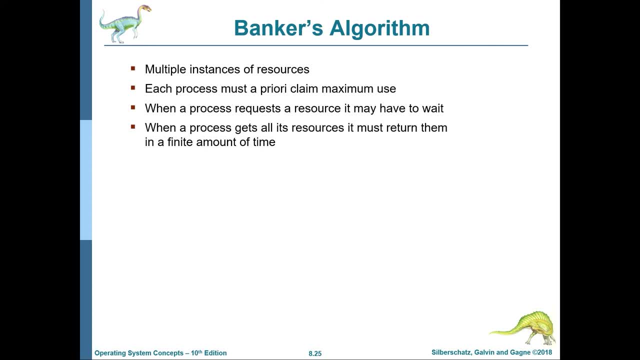 use this algorithm if more than one instance of a resource type is present in the system. As always, each process must kind of declare a resource type Priority: it's maximum use. by that I mean the maximum amount of resources it might need in the future it will request in the future it should declare right at the beginning. 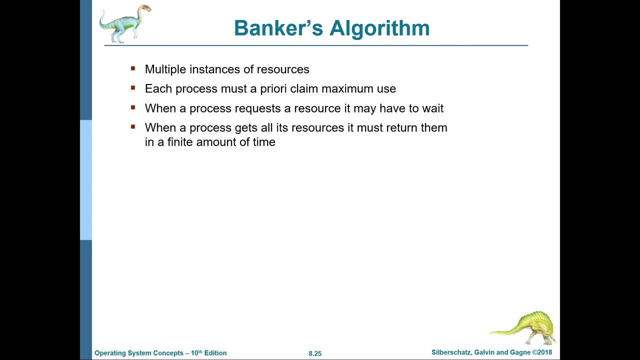 It may so happen that when a process makes a request for a resource, it might have to wait a little bit before the operating system assigns the resources to the process, and when a process gets everything that it needs, it must return them in a finite amount of time. It cannot. 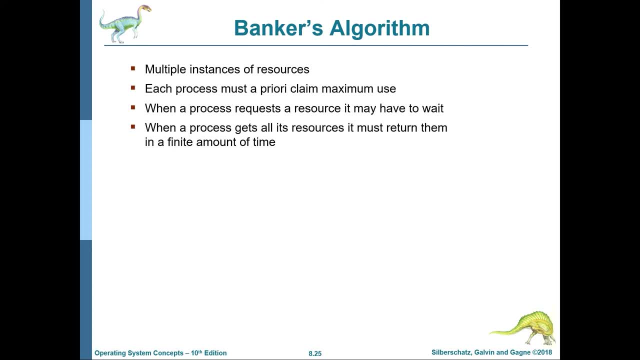 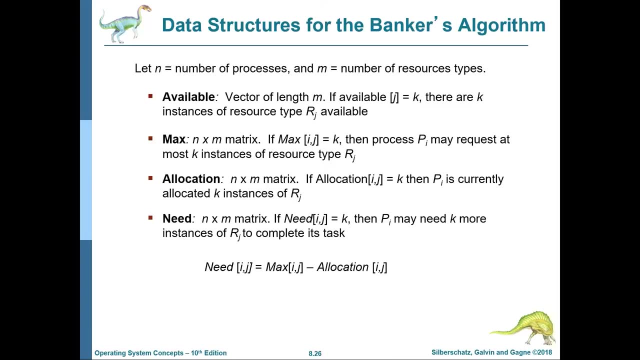 just keep holding to them for a long, long time, because that might result in starvation of other processes. Let's discuss some data structures that we will need for using the bankers algorithm. Let n be the number of processes and m with a number of resource types. Now we will define. 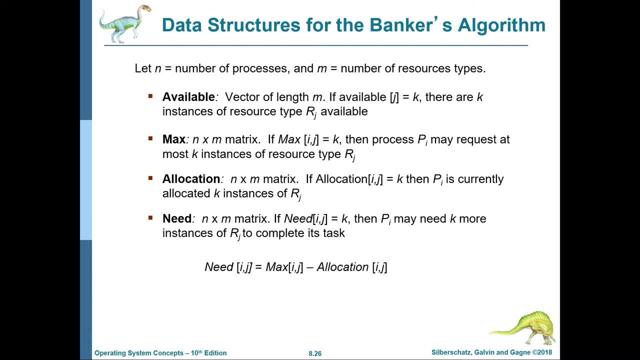 a vector that is called available. It will be a vector of length m, and then this vector- what that means available- is basically going to be a row vector. a row vector, as in. it will be a vector like this, going from left to right, and then it will contain the amounts of resources. 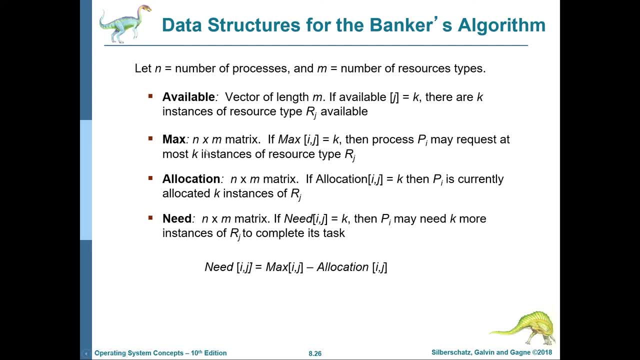 available for each kind. so if the first cell is for cd-rom drives, the second cell is for hard drives, the third cell is for printers. if we have two, one, two that means two cd-rom drives are available at this point of time, one hard drive is available and two printers are available at 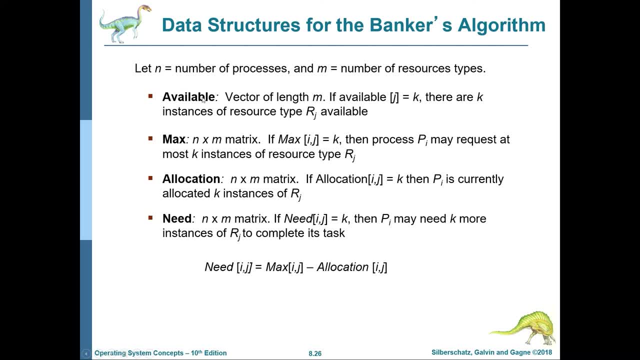 this point of time. so available is basically the availability of resources in the system. it is a vector because different resource types are there and each resource types might have different numbers of instances available. that is why it is a vector. it is basically a row vector that goes from left to right, something kind. that kind of looks like this. then we will define a. 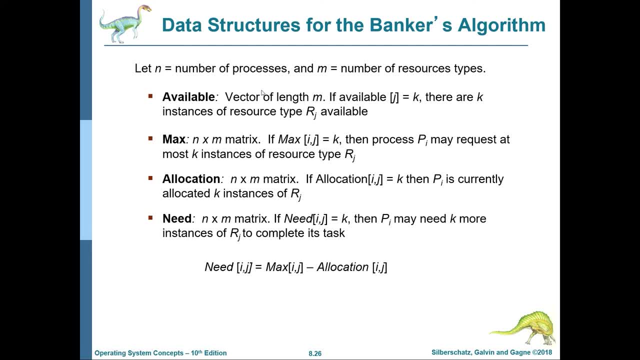 matrix called matrix matrix. it is a n cross m matrix, like a table, and then this table will contain the maximum request that processes can make for certain kinds of resources. so here the rows will represent the processes and the columns will represent the resource types. so if this is a cell which is for 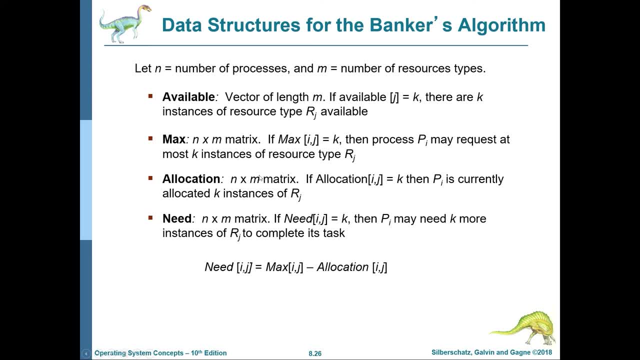 row number two and column number three, and if it has got a value of three, that means process number two can make a row number two and column number three, and if it has got a value of three, that means it can make maximum three requests for resource type three. now we will define another. 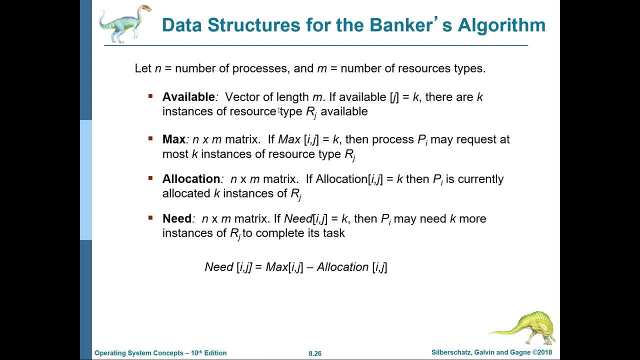 matrix called the allocation matrix. it is a same kind of table, like max as in the same size- n cross m- in which the rows are the process numbers and the columns are the resource numbers. and this matrix, this table, represents the current allocation of resources to the processes. so if a cell has a 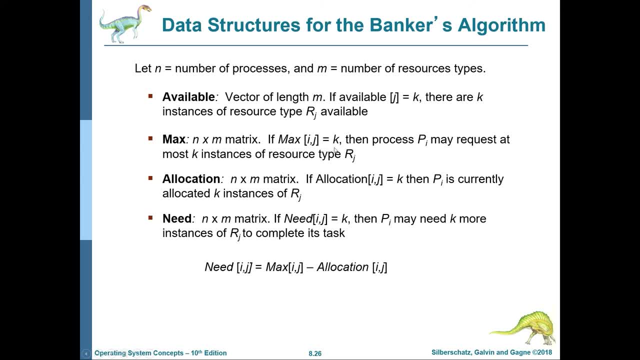 number. that means, whatever the row number it is, that process number has currently those many instances of that resource type at this point of time and there is a need matrix which is of the same size as both max and allocation, and it is basically the future need of the process. and, as you can clearly see it, 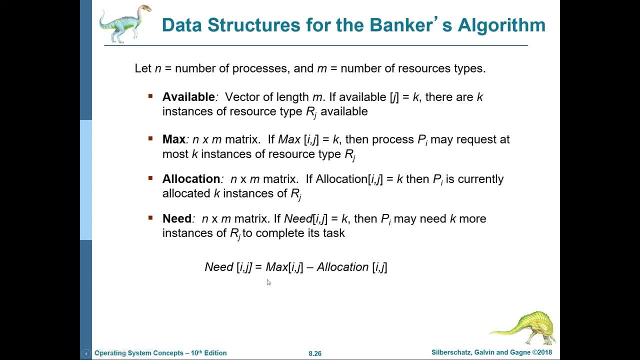 is equal to max minus allocation. so max is basically the maximum number of instances of resources processes might request, and allocation is the current value that has been assigned to them. so the need will be the difference. so if, if the max in a certain cell is 10, that means that 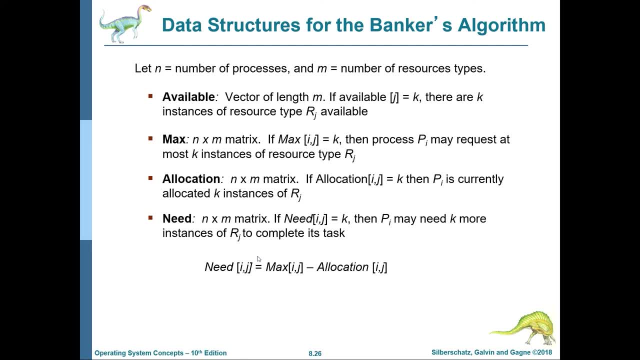 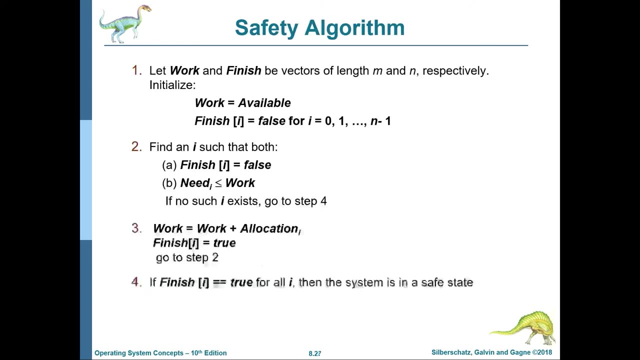 process can maximum request 10 instances of that resource type and if allocation for that corresponding cell is 2, that means need is 8. that means currently that process has 2 of those resources and in future it might need 8 more because max is 10. now let's discuss the safety. 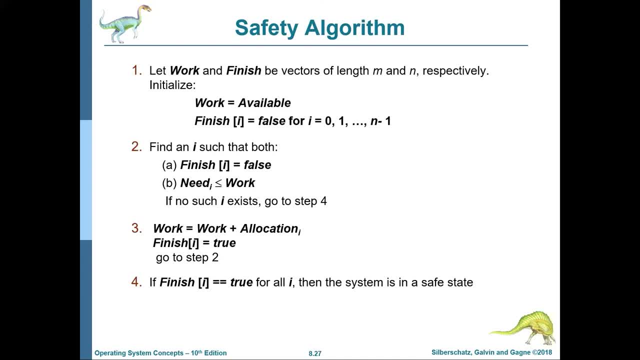 algorithm. now, this is a safety algorithm and it is a safety algorithm and it is a safety algorithm algorithm that you will use to determine if the state of the system is safe. so to do that, let's define two vectors- work and finish, and they will be of length, m and n respectively. work will: 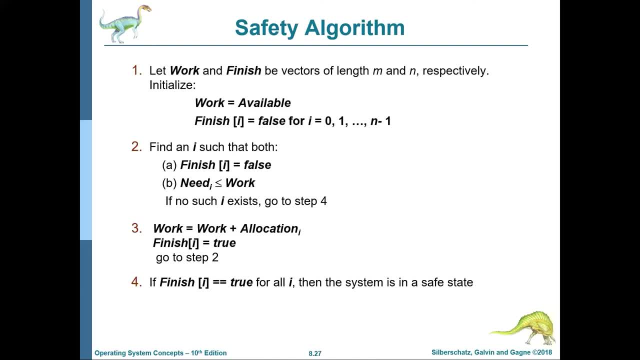 basically hold the availability of resources and finish will hold whether a process has finished or not, since m kinds of resources are there. that is why work has a length of m and because n number of processes are there. that is why the length of finish is n and we will initialize. 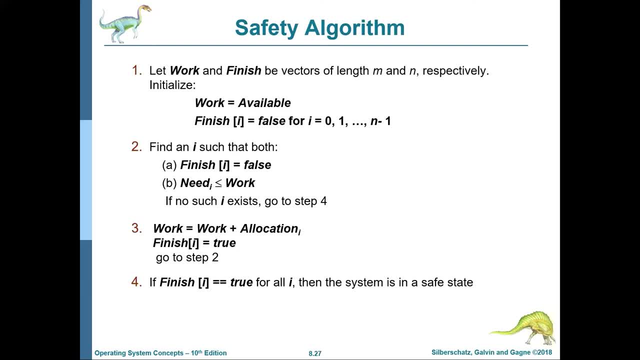 work to available. we will make work equal to the currently available resources and then we will set all the processes finish value to false. that means none of the processes have finished as of yet. we will find an i such that the process has not finished and whose need can be satisfied with. 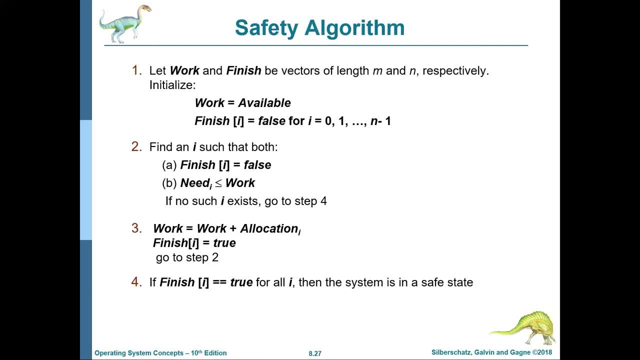 right now. so when we say need i is less than equal to work, we basically mean that. so whatever is available isn't there in work and need i is the need of that process, i which has not finished, because finish of i is false. if no such i is there, then we go to step four. but if we find such an i, 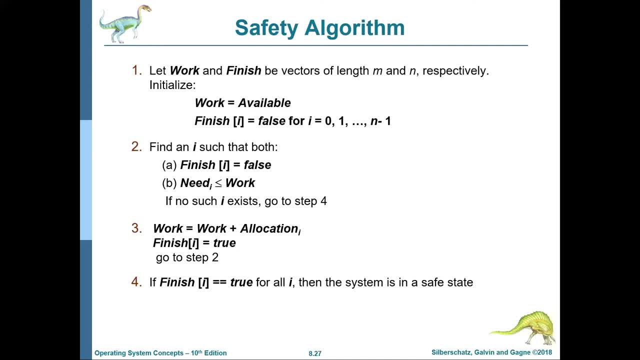 what we do is we will assume that the process will do its job, return its current allocation back to the work pool, and we will mark the process as true in the finish vector. so that is basically what is happening in step three. so let me say that again, we will find a process. 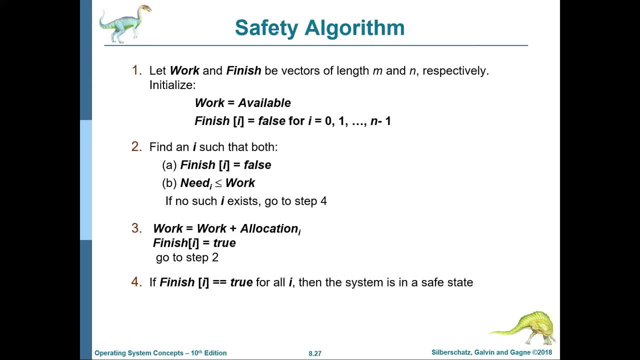 which has not finished and whose need can be satisfied with whatever is available in the work pool. we will assume that the process has finished execution and we will set the finish of i to true. that means the process has finished execution and we will take whatever has been allocated to that process and return it back to the work pool. that 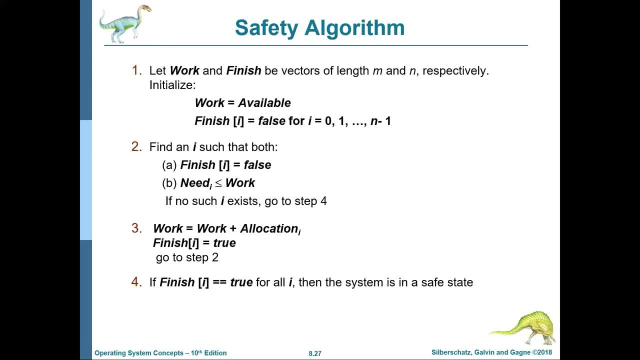 is why we do work equal to work plus allocation, and then we go back to step two. if we keep doing this, at one point no such i will exist. and then we will go to step four, and if finish of i is true for all processes, that means all processes have finished execution, then the system is in a safe 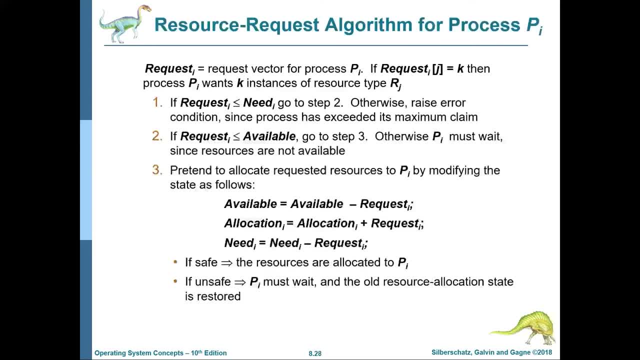 state. now we will study the resource request algorithm for process p i. so a process p i now makes a request and we will assume that the system is already safe. and how will we know that the system is already safe? so we will employ all our data structures and run the algorithm that we discussed. 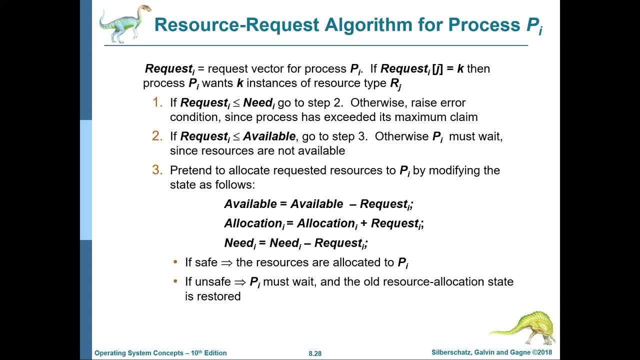 in the previous slide to determine if the system is in a safe state. so let's say that the system is already in a safe state. let's assume the system is already in a safe state and process p i has made a request for certain number of resources. now we will see if we allocate these resources to the 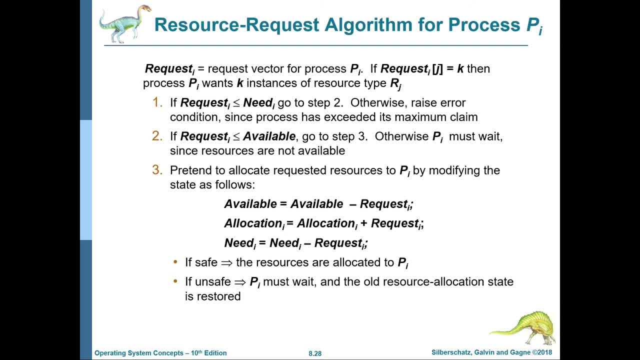 process. will it still leave the system in a safe state? if it still leaves the system in a safe state, then we can assign those resources to that process. if it does not leave the system in a safe state after allocation of the resources that is requested by that process p i, then we will. 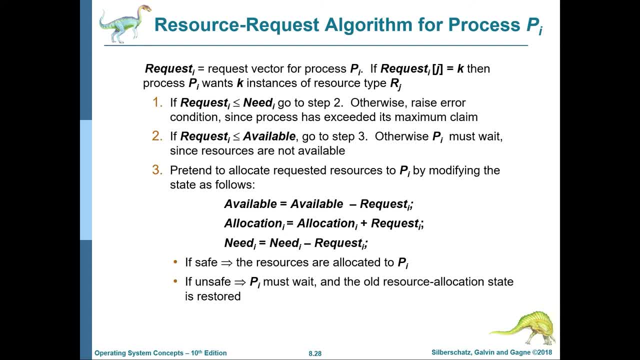 not allocate those resources and we will ask the process pi to wait a little bit. So the request for process pi will come in as a request vector, which is called request i, and its size will be m, because the request vector will basically contain the different number of instances of resource types that this process needs, and there are m different. 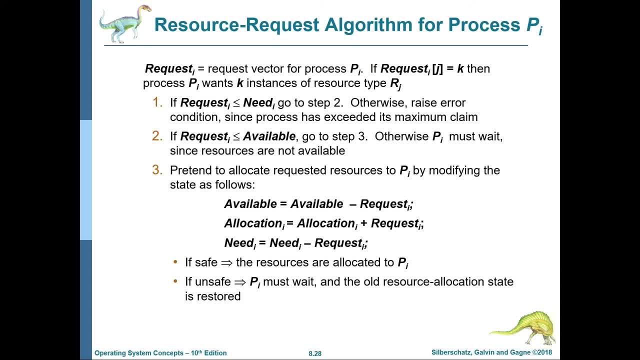 numbers of resource types. so request: i will be a vector whose length is m. Now step one. if request is less than equal to need, then go to step two. otherwise raise error condition, since process has exceeded its maximum claim. So the process initially in the avoidance algorithm that we are trying to study here. 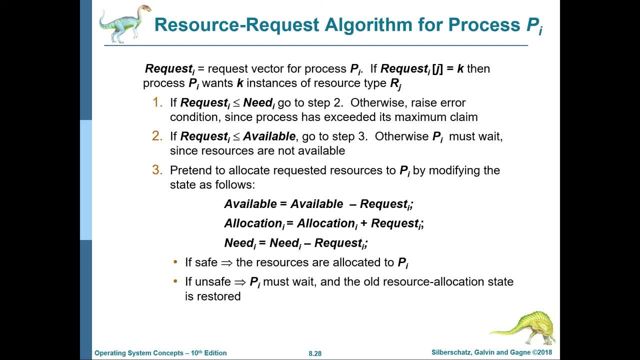 each process has to kind of declare its maximum claim. Now the request is more than the need, that means the process is cheating. It told a lie in the beginning, so we have to raise an error Now in step two. if the request is less than equal to available, then go to step three. otherwise 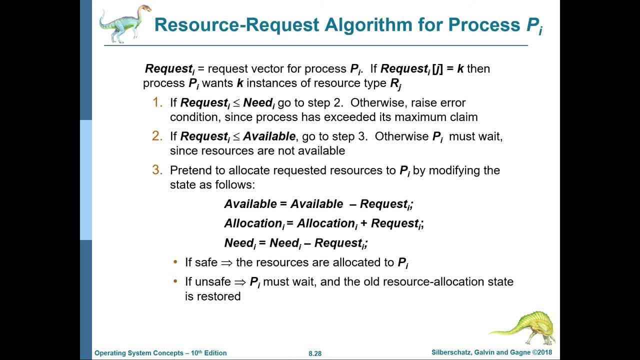 pi must wait since resources are not available, because if the request is more than what is available right now, then certainly the operating system has to ask the process to wait, otherwise we can move on to the next step. In the next step, it is very, very easy to see what is going on over here. 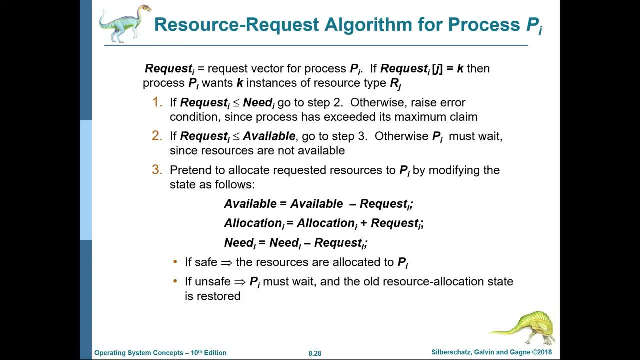 We will pretend that the allocation is being done. We will pretend as if the resource request of pi has been granted. So what will happen? the available pool will reduce by how much? by the request amount that pi has done. So we will do: available equals available minus request. so available quantity of the resources. 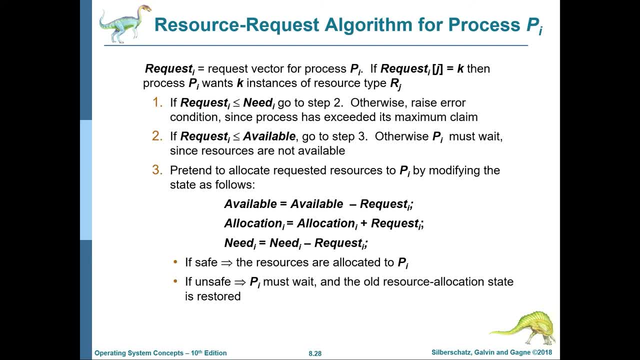 will go down And allocation for that process will go up by how much, How much we have allocated, and that is equal to request. So allocation- i now keep in mind allocation. i is a vector, though allocation was a table before. if i put a i, then it is just that row, the row for that process, right? so that is. 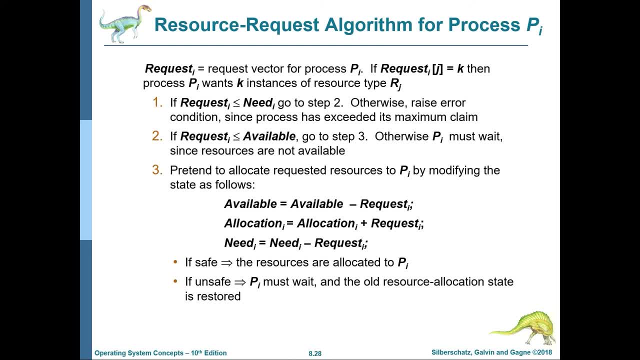 also a vector of size m, and that allocation will go up and the need will go down, because now the process already has those many requests, So the need also goes down. Now we will run the safety algorithm that we discussed in the previous slide and after 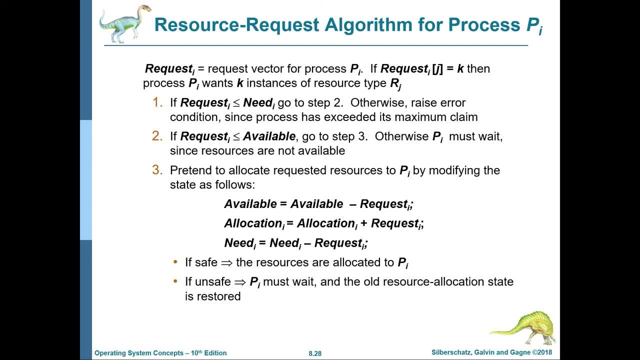 running that algorithm. if the state is still safe, then it is okay to allocate the resources that has been requested by the process pi to the process. otherwise pi must wait, because if it does not wait and the operating system gives the resources to the process pi, then the system will become unsafe and we don't want that because once the system becomes, 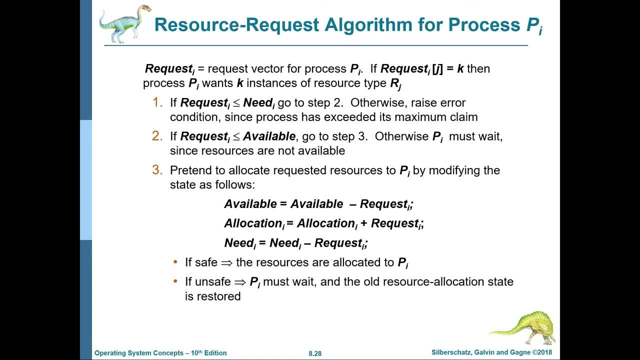 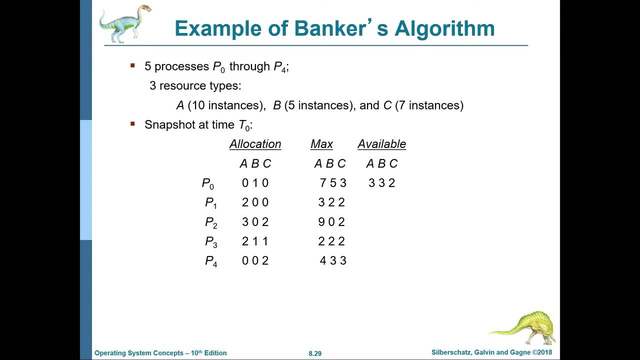 unsafe. a possibility of deadlock will arise, and we don't want that. Now let's look at an example of the banker's algorithm. there are five processes, p0 through p4, so that is p0, p1, p2, p3 and p4, and there are three resource types: a, which has ten instances. 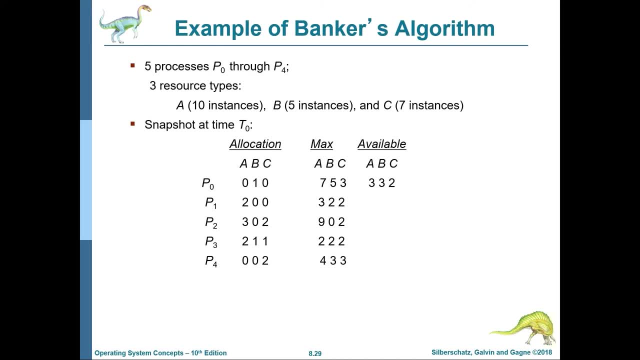 b, which has five instances, and c, which has seven instances. So we have taken a snapshot, at time t0, of the resource allocation state, And so I hope you can understand the table. but let me quickly go over the table in case you are not clear about the allocation max and the available matrices. 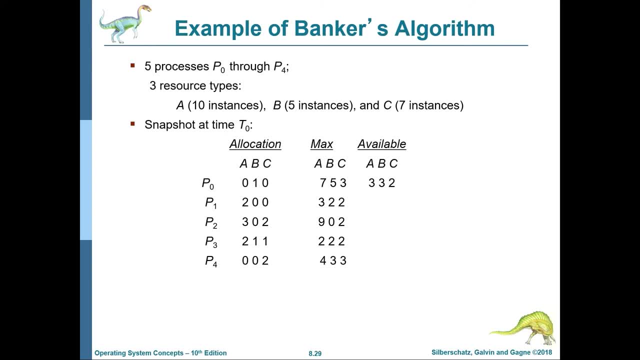 At this point of time the available vector has 3, 3, 2. that means there are three free instances of a available, three free instances of b available and two free instances of c available. The allocation matrix of the processes and the resources is kind of given on the left. 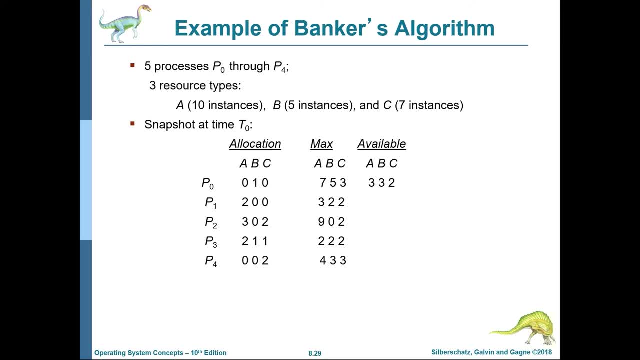 In the first row you see 0, 1, 0. what does that mean? that means zero instances of a have been allocated to p0 at this point of time, one instance of b has been allocated to p0 at this point of time and zero instances of c have been allocated to p0 at this point. 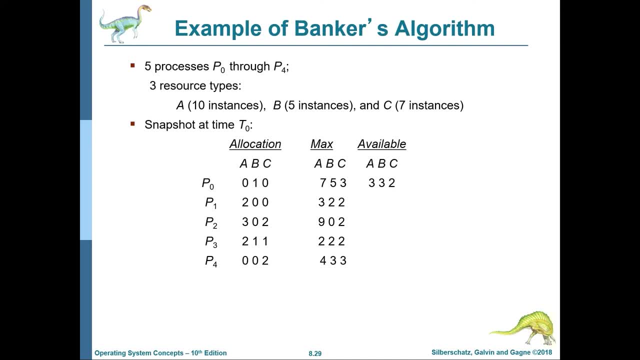 of time I will just try to explain one more row from that table. let's look at the row for p3. we see 2 1, 1.. That means Three instances of a have been allocated to p3, one instance of b has been allocated to. 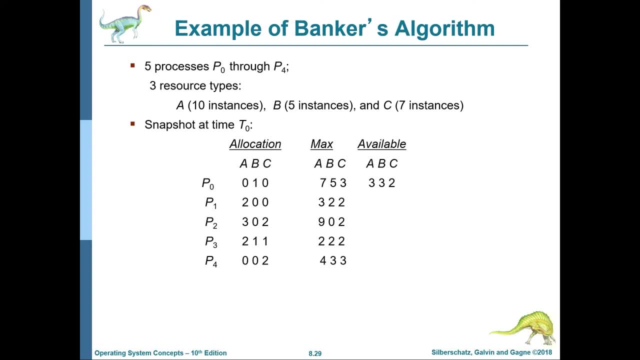 p3 and one instance of c has been allocated to p3. to the right of the allocation matrix is the max matrix, And what does that mean? So I'll just explain the first row, that is 7 5: 3.. That means p0 can maximum request seven instances of a, five instances of b and three instances. 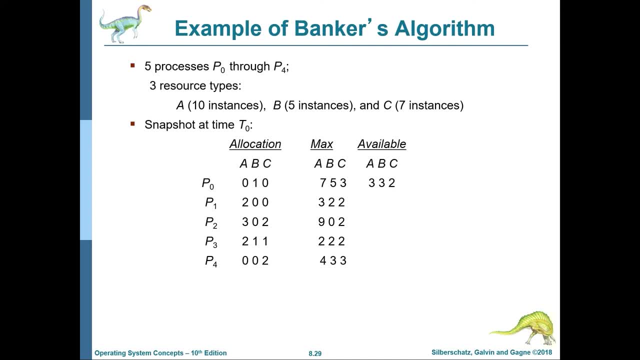 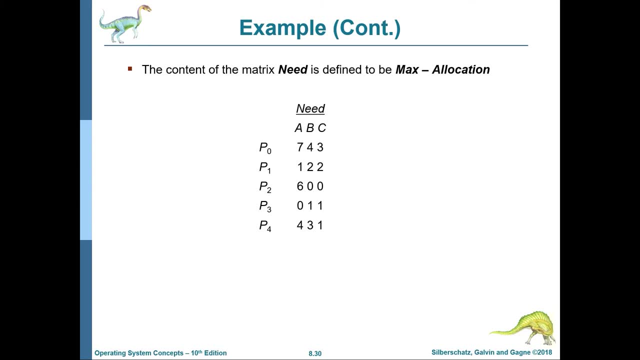 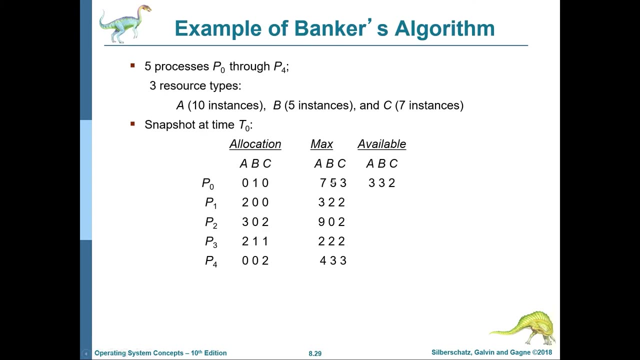 of c, And if we do max minus allocation we will get the need Matrix. so let's see how the seven 4: 3 came. so I'll just go to the previous slide. So the max was 753 and the allocation was zero, one zero. 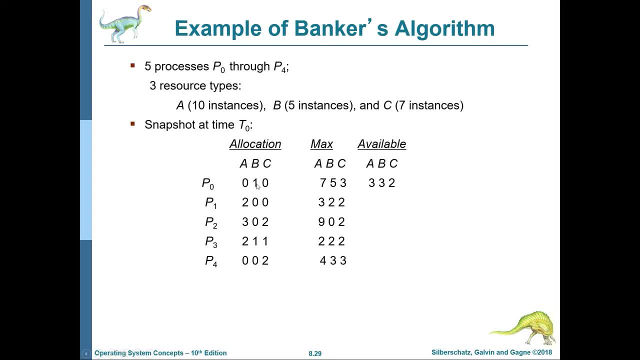 So since we 0 already has one instance of b, so it will request only four more, And it has 0 and zero of a and c, So it can still Request 7.. … And…… 3.………, 3.…………, 3.………. 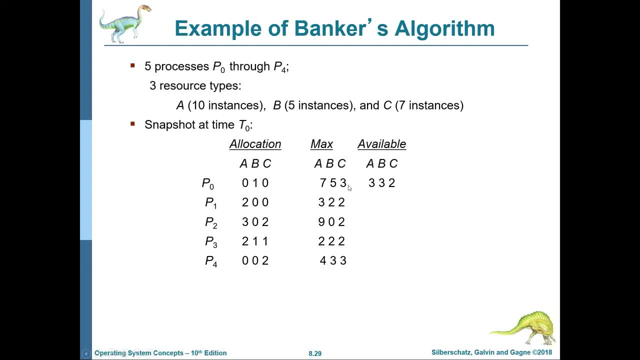 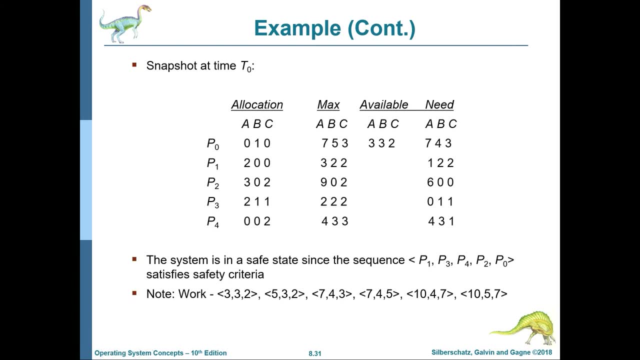 a and c, so we will have 7, 4, 3 and the first row, and that is what is there over here. now let's see if this is a safe state. now for a safe state. we saw the algorithm that we need to mark all the processes finish as false, so we'll assume that none of the processes have finished. 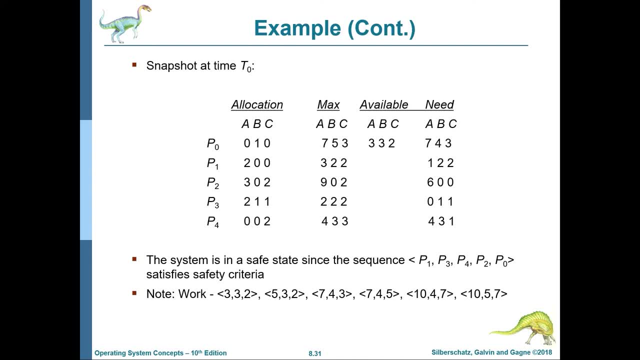 and we will take the work vector as the available vector to begin with. so since available was 3, 3, 2, i have taken the work vector, the initial work vector, to be 3, 3, 2 and we will look for a process which has not yet finished and whose need can be satisfied by whatever is available in the work. 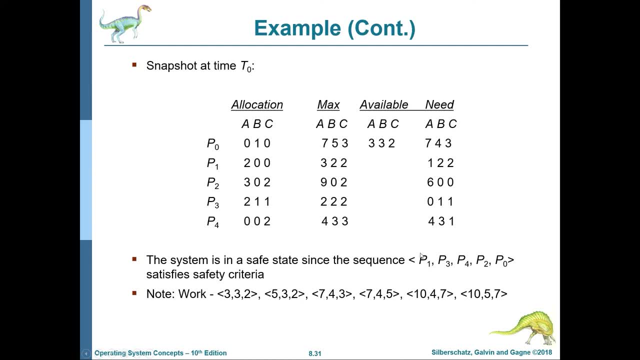 so let's see if we take p1. well, of course it has not been finished because initially we have marked all the processes as not finished finished in the finish vector. its finish i is false for all of them and for p1 the need is 1, 2, 2. 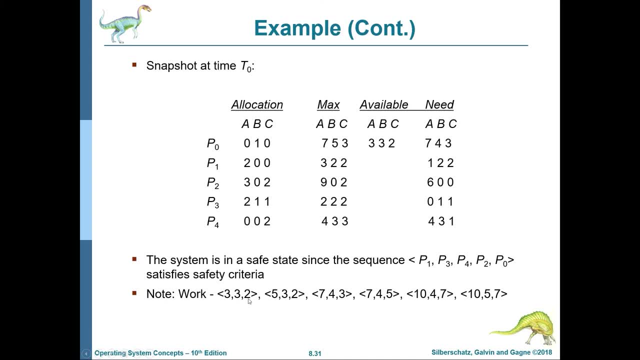 can that be satisfied by work? yes, 1, 2, 2 is- is smaller than or equal to work. well, 1 is less than 3, 1 is less than 3 and 2 is less than equal to 2, so it can be satisfied. so what we will do, we will. 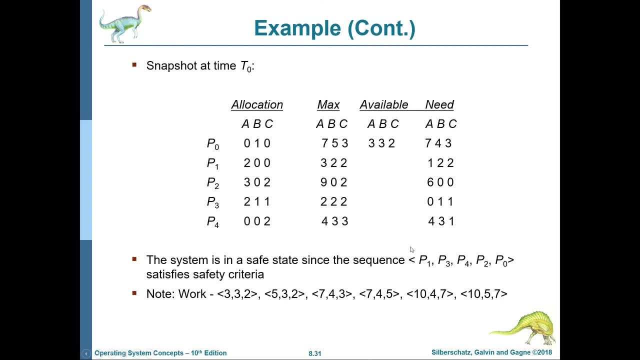 mark p1 as done. that is, we will say finish of 1 as true and we will return whatever has been allocated to p1 back to the work pool. so what was the allocation of p1? it was 2 0 0. so we take 2 0 0. 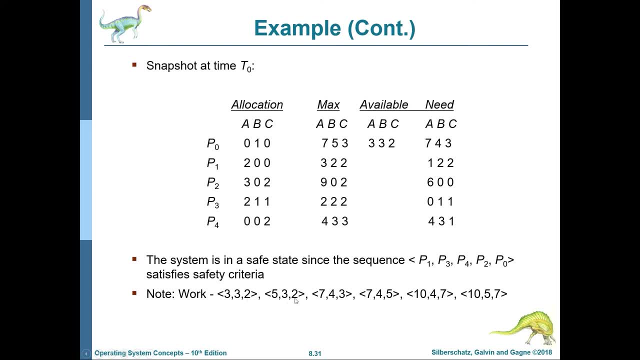 and we add it to 3 3 2. so we have 5 3 2 over here now. next we will go to p3. so you might ask: why did we go to p3, why didn't we go to p2? so if you look at the need of p2, it has got 6 0 0. but with whatever we 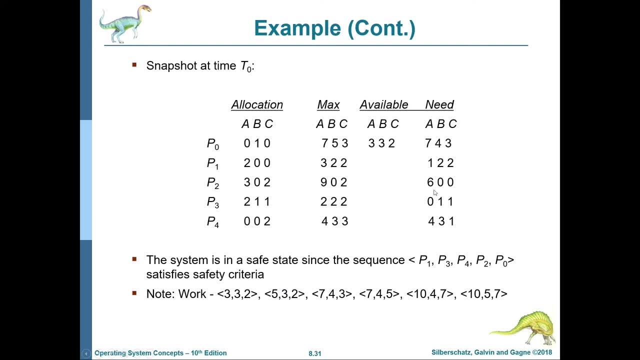 have in the work pool. can that be satisfied? well, the ones for b and c can be satisfied, but the one for a, which is 6, cannot be satisfied by 5. so we choose to go to p3 and whose need is 0, 1, 1 that. 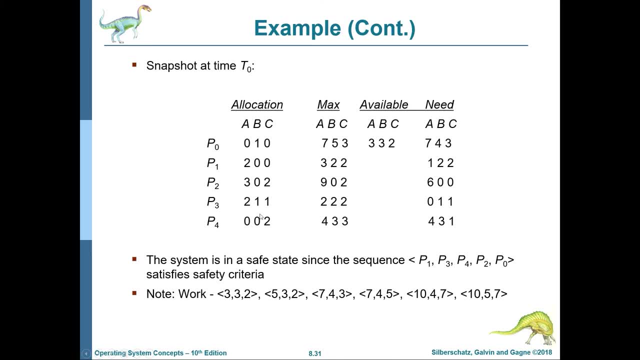 can be satisfied. so we will just assume that this has finished. we will set its finish to true and we will return its allocation back to p2. so we will just assume that this has finished. we will return its allocation back to work. so we will add 2- 1, 1 to 5, 3, 2 and we have 7, 4- 3. we keep doing. 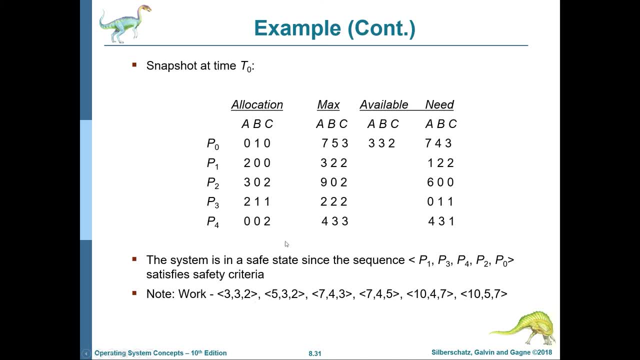 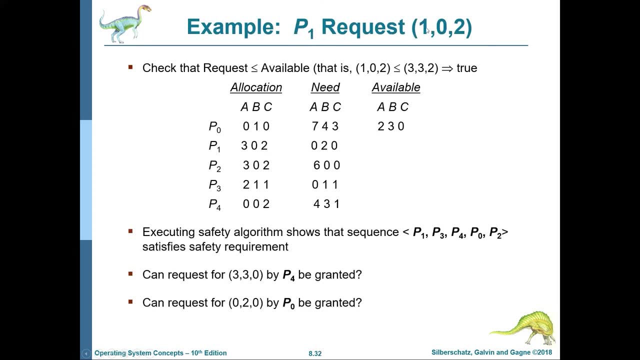 this and in the end, we see that all the processes are able to finish. so this is a safe state. now p1 makes a request of 1, 0, 2, and what does this mean? it means it made a request for one instance of a, no instances of b and two instances of c. now let's use the banker's. 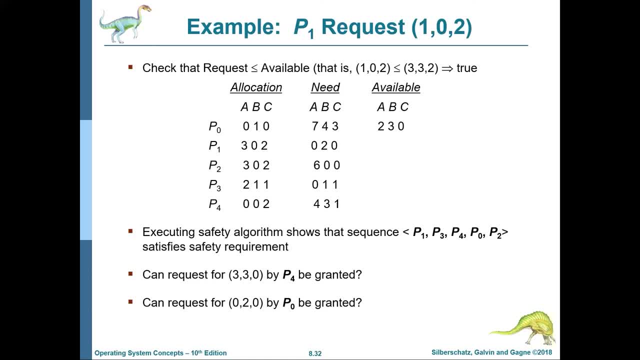 algorithm to make a request for 1, 0, 2. and what does this mean? it means it made a request for one instance of b and two instances of c. now let's use the banker's algorithm to see if we should be entertaining this request, if satisfying this request will take our state from a safe state. 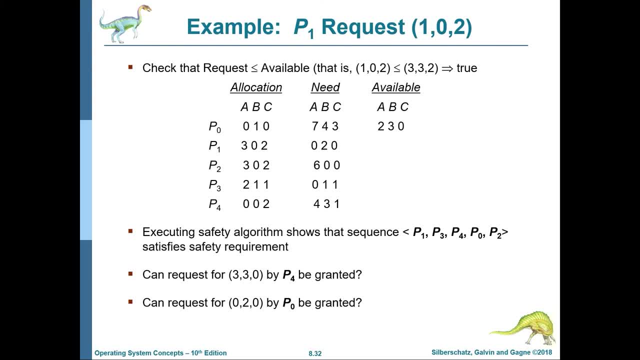 to one unsafe state, because from the previous slide we already calculated that the state was a safe state. but we should not just grant the request of p1 if it will take our state to an unsafe state. so let's see if that is the situation. so we will see if the request is less than equal. 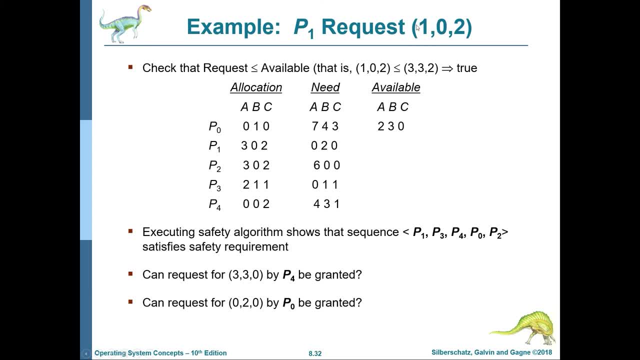 to available, because if it is not available, whatever the request is, it will not be available. then we cannot satisfy the request. we see that 1, 0, 2 is less than equal to 3, 3, 2. well, 1 is less than 3, 0 is less than 3 and 2 is less than equal to 2. so that is true. so we can proceed further. 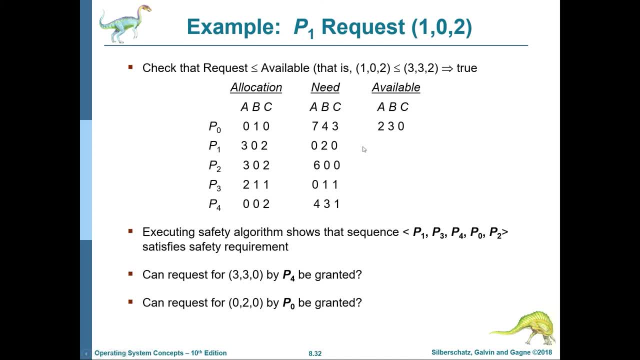 now what will happen? available will go down. by what amount? by 1 0, 2, so that has gone down, it has become 2, 3, 0. what was it before? it was 3, 3 and 2, and we have subtracted 1, 0, 2, so it has become. 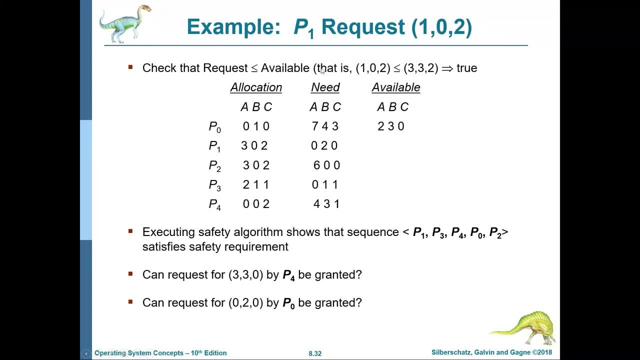 has the need gone down? yes, the need for p1 has gone down and has the allocation gone up? yes, the allocation of p1 has gone up. so this is the new state and we have to evaluate if this state is safe. now it is an exercise for you and you will come up with this sequence. so if this is, 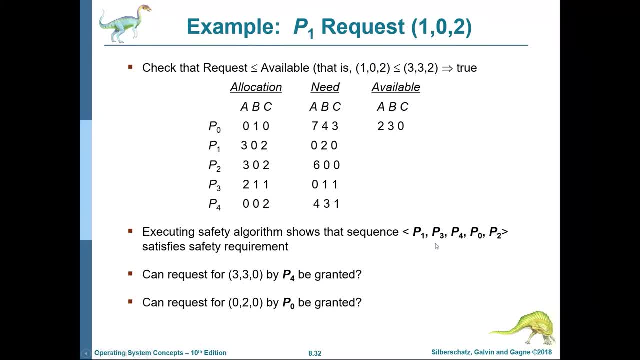 the sequence in which we go on marking the finish to true and returning the allocation of p1 to true, we will come back with this sequence. so if this is the sequence in which we go on back to the work pool, you will see that at the end all the processes will finish successfully. 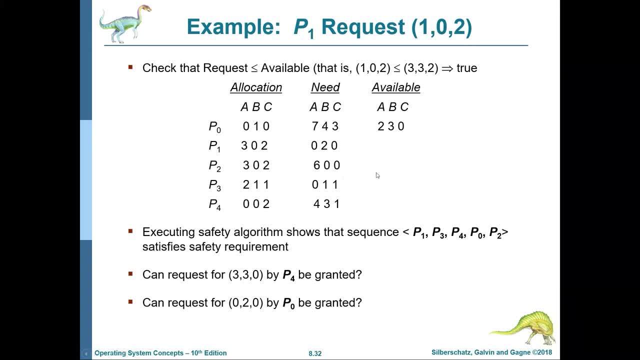 So this is a save state and it is also an exercise for you to figure out if the request for P4, that is 330, can be granted and the request for P0, that is, 020, can be granted. And while you are solving the question, assume the state on the previous slide to be the. 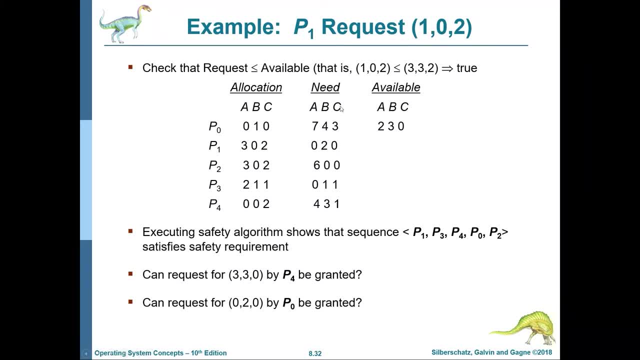 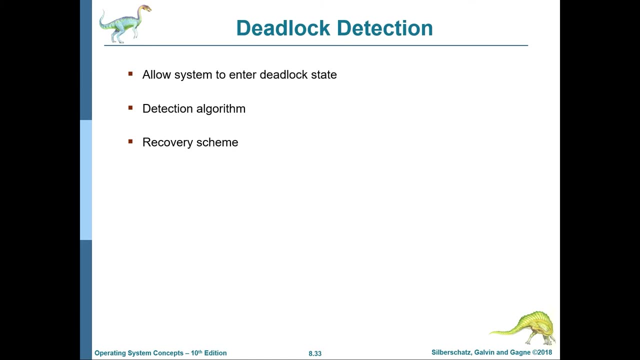 starting state. You should not assume this as the starting state, because this is just the specific examination of the request for P1.. So, now that we have studied deadlock prevention and deadlock avoidance, let's see. if a system chooses not to prevent or avoid deadlocks, what can it do? 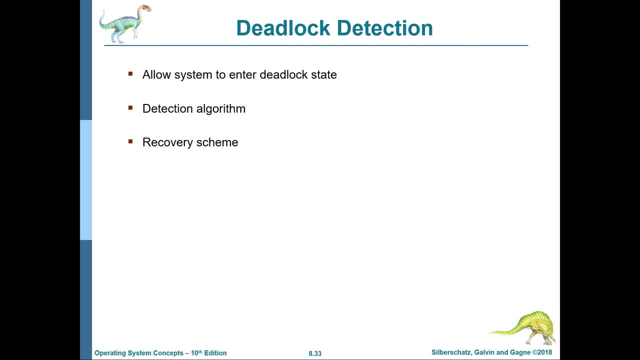 Well, it can choose to detect deadlocks because deadlocks will happen. it is not trying to prevent or avoid deadlocks- deadlocks. so when deadlocks happen, it has to come up with algorithms to detect that a deadlock has happened and then it may choose to deal with that situation. so the system has clearly allowed. 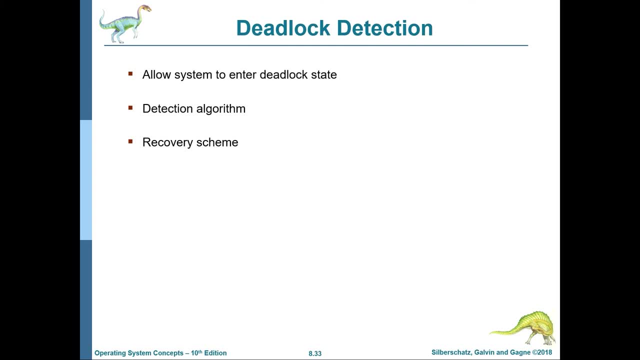 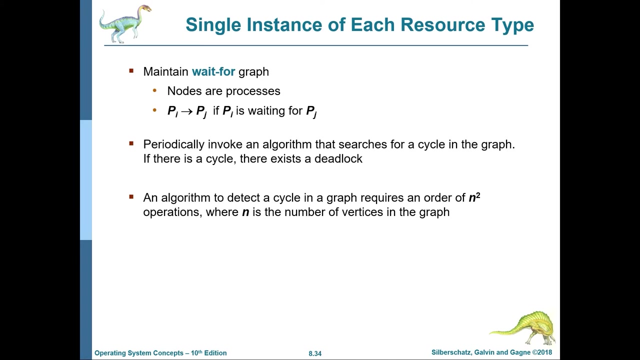 processes to get into a deadlock. now we will discuss some algorithms to detect the deadlocks and then we will go on to see some recovery schemes which the system might employ to recover from a deadlock. so, as we discussed before, so there are two situations here, if a single instance. 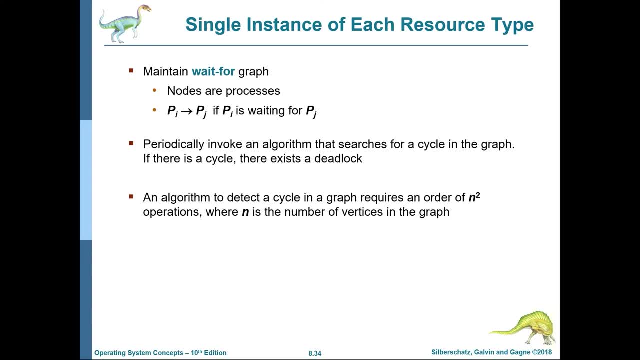 of each resource type is there, then we can use graph methods to detect deadlocks. if multiple instances of each resource type is there, then we have to use a little bit slightly different version of the banker's algorithm. you will see, it is kind of very, very similar to that. 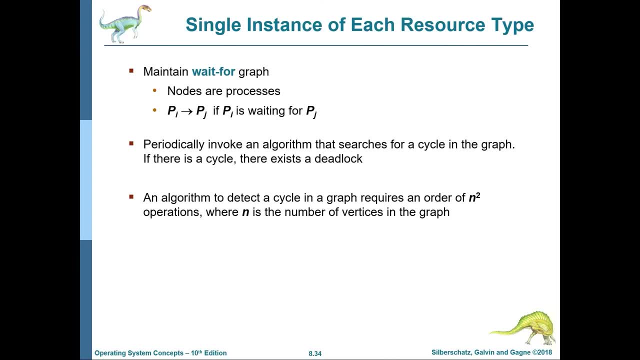 to detect if a deadlock is there. so let's focus on the simpler one, in which only single instances of each resource type is there. so we will have to maintain a wait for graph. now, what is a wait for graph? a wait for graph is another modification of the resource allocation graph. here there are no resources. 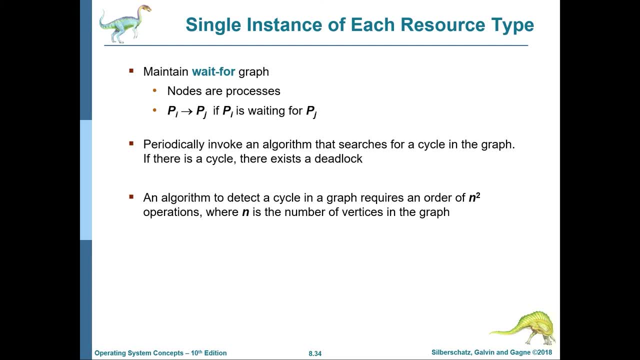 anymore. so we get rid of the resources and we only have processes in this graph. now, an edge from one process to another is called an edge from one process, and this is what we are trying to do here. so we are taking an edge from one process and again we are taking an edge from one process. 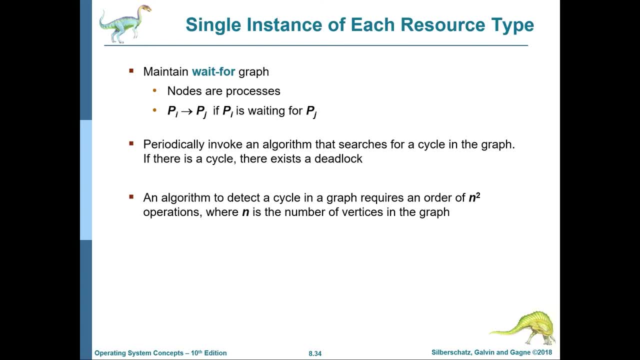 to another process will only be there if the first process depends on resources which the second process is currently allocated. So if there is one process process one, there is another process, process two. there will be an edge starting from one to two if P1 is currently requesting a resource. 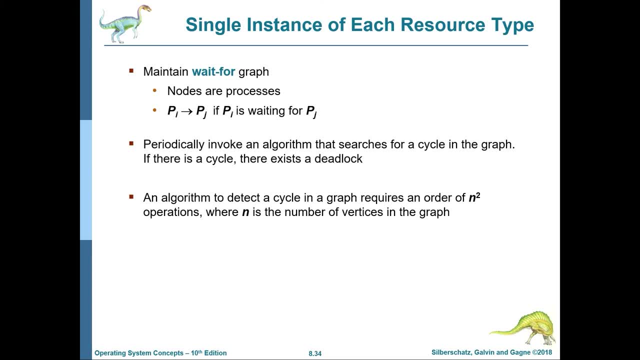 but it is not getting that resource because process two is currently allocated that resource. Now, once we maintain a wait for graph, and if that graph at any one point of time has a cycle, then a deadlock has happened. So we have to run this algorithm from time to time to 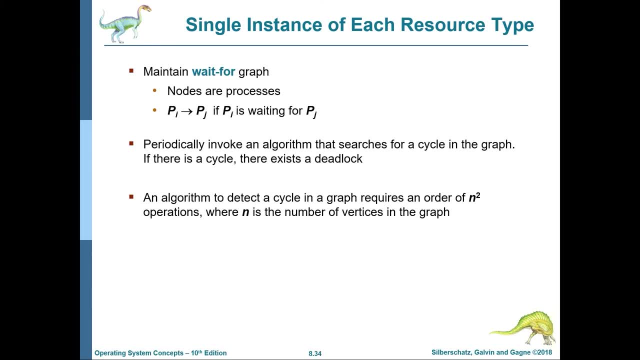 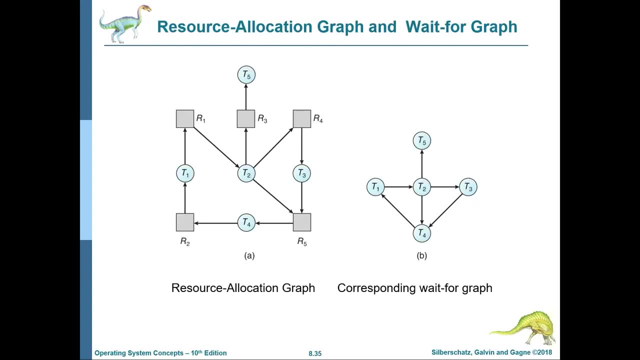 see if the wait for graph has a cycle and at one point of time. if we find a cycle, then there is a deadlock. Here you can see an example of the wait for graph. Now on the left side we have a resource allocation graph and on the right side we have the 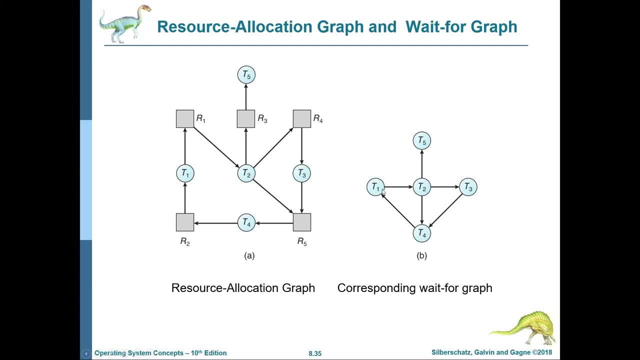 corresponding wait for graph. Now, why is there an edge from T1 to T2? because T1 is requesting the only instance of R1, but that has been given to T2.. So since it is waiting for T2 to give up that resource, there is a edge from T1 to T2.. Why is there an edge from T2 to T3?? 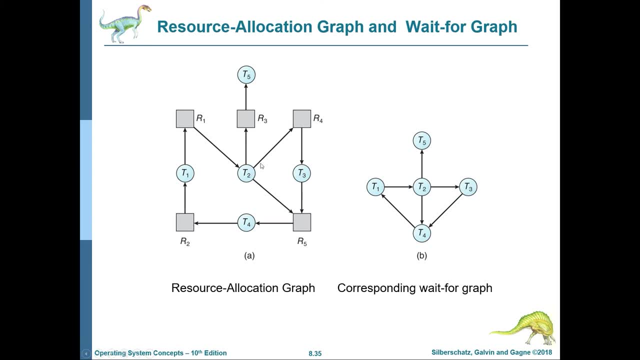 Because T2 needs. it has requested an instance of R4, which is currently given to T3.. So T2 is waiting for T3 to finish so that it can get that only instance of R4. So on and so forth. Now does this graph have a cycle? Yes, it has cycles. It has more than one cycle and this is: 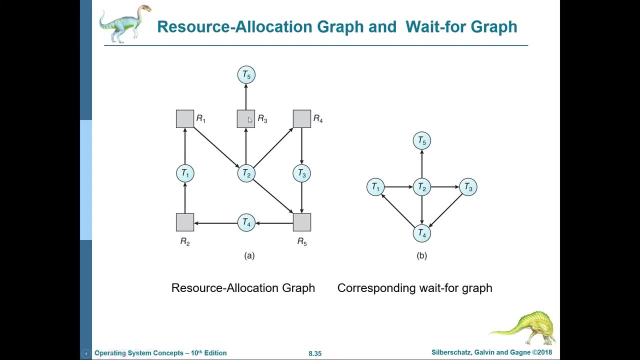 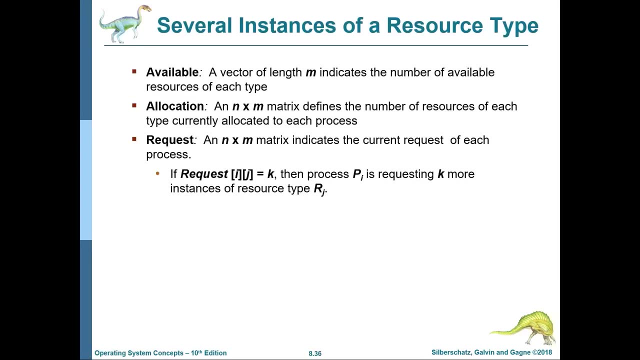 a deadlocked situation. You can actually look at the resource allocation graph to realize that this thing is a deadlock. Now, what to do? if several instances of a resource type are there, Then we will maintain the same available matrix, the same allocation matrix, but we will add a new matrix. 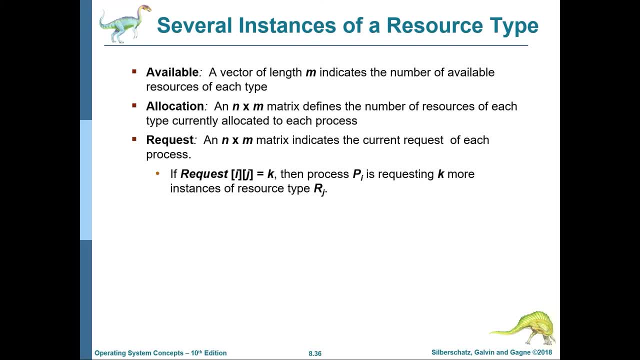 It is called the request matrix. It is the same size as the available in the allocation matrix, That is, it is of size n cross m. and if a certain cell right has a value of 3, let's just say then whatever is the process number, then that process has requested three more instances of that resource type, So that 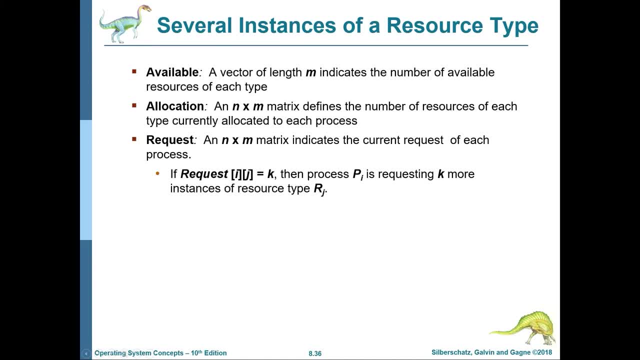 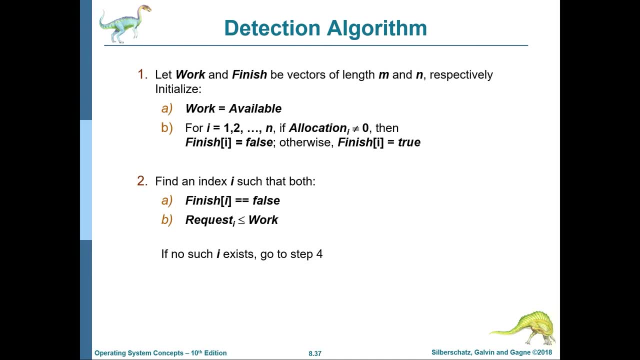 is the request matrix. So now this is the detection algorithm. So, as before, we will maintain two vectors: work and finish. So you already know the sizes of work and finish. We use this in the bankers algorithm to figure out if the state is safe or unsafe. Now we will set work as a. 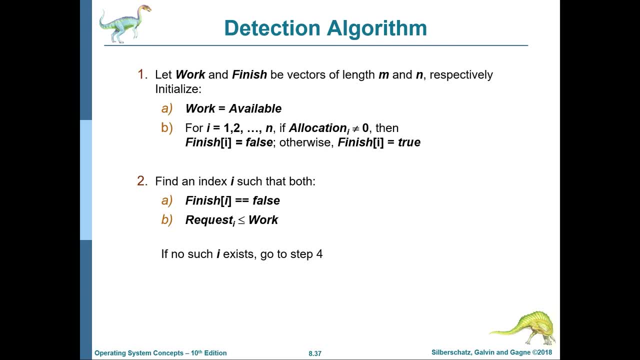 available- and we have done this before- and this time around we will not set all the finishes to false. We will only set the finishes to false if they have some allocation. If they don't have any allocation, then we will set their finish to true. So if allocation is not equal to zero, that means 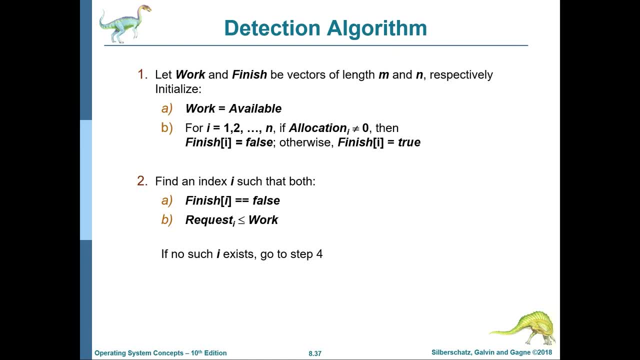 they have something allocated to them, that process, then the process has not finished. If they have nothing allocated to them, then we will mark that finish to true. Then in step two we will find an index such that the process has not finished and its request can be. 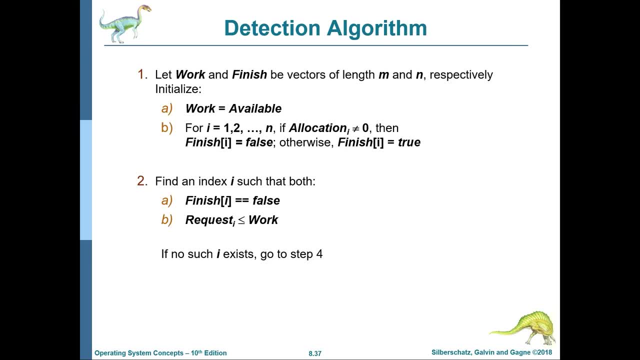 satisfied with whatever we have in the work pool, with whatever number of resources we have with us in the system. If the request for that process can be granted, with whatever we have, then we will find that index. If no such index exists, then we go to step four and in step three, what are we going to do? 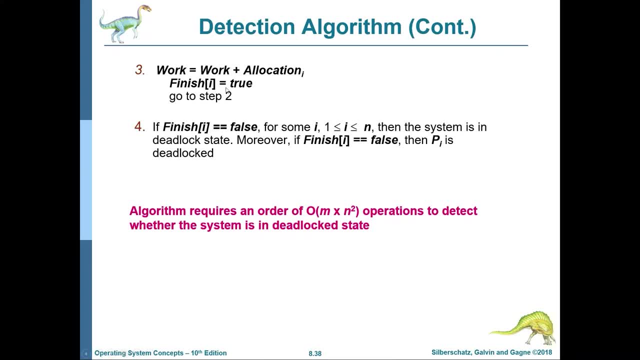 Just like before, we will mark the finished state of the process to true and we will take its allocation and add it back to the work pool, and we have already done this in the bankers algorithm also. So we will assume that the process has finished, because whatever it might request can. 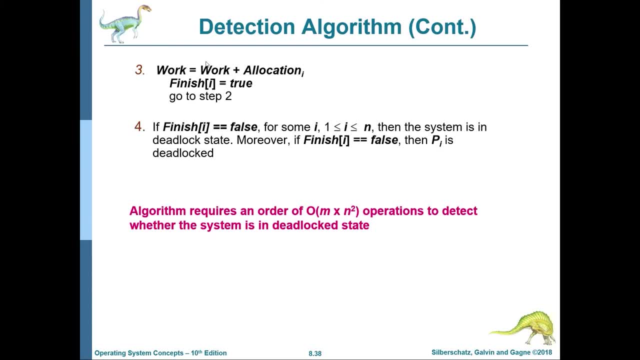 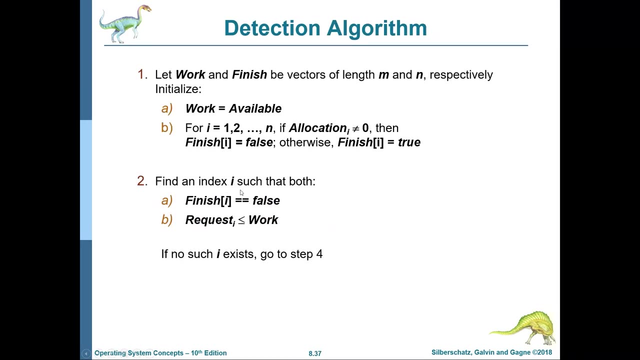 be satisfied with the work pool that we have. So we will mark the process as finished and we will take its allocation and add it back to the work pool, and then we will go back to step two. Again and again we will find some index, the index of a process which has not finished and whose 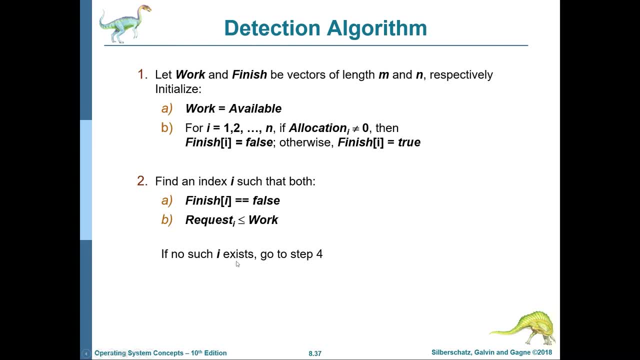 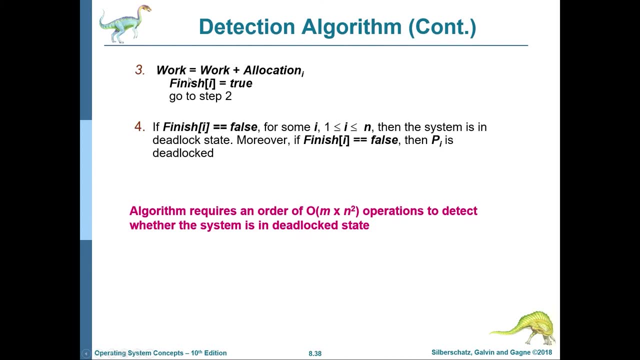 request can be satisfied with whatever we have in the work pool. If there is no such i, then we will go to step four or we will go to step three. So we will keep doing this. at one point we will not be able to find any i. either all of them have finished or there is. there are one or more. 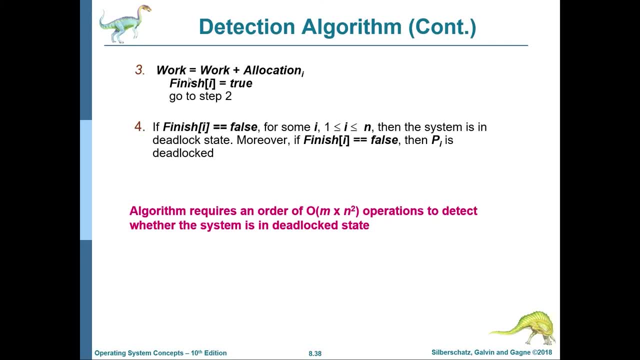 processes whose requests are so high that the work pool that we have will will not be enough to satisfy that. So once we reach step four, we will see. is there some i which has not finished? and if that is the case, then there is a deadlock in the system and, in fact, all those indices which are false, they are. 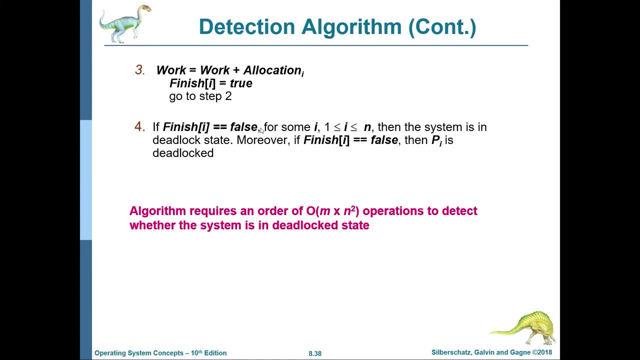 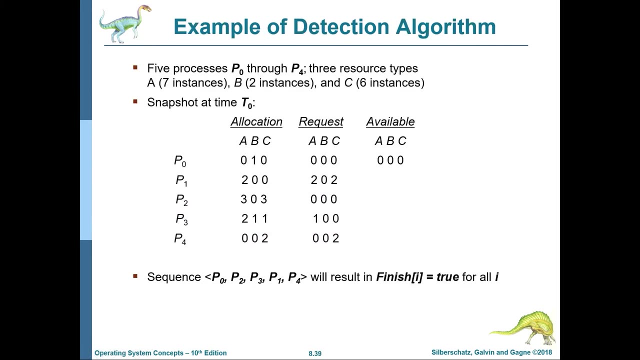 deadlocked. they are not finished, they are in a deadlock and they are not able to proceed further. This algorithm requires an order of o of m cross, n square, where m is the number of resource types and n is the number of processes. Now let's look at an example of the detection algorithm. So we have five processes, p, zero through. 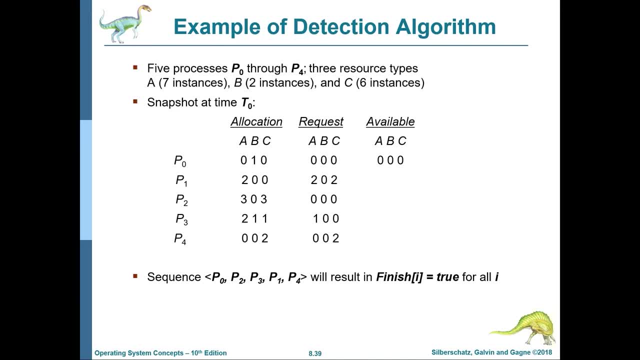 p four. We have three resource types: a has seven instances, b has two instances and c has six instances, and the snapshot of the resource allocation state at p zero is given. Now we have the allocation a matrix, the request matrix and the available vector. At this point of time, nothing is. 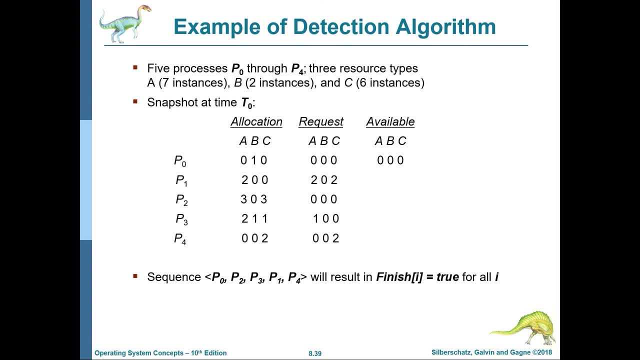 available. so we will set work to zero, zero, zero. Now let's see is: is the allocation of any process zero? completely no, So we will begin with finesse as false for all the processes. Let's see: if we choose p zero, its request is zero, zero, zero. Can that be satisfied by whatever is available, In fact? 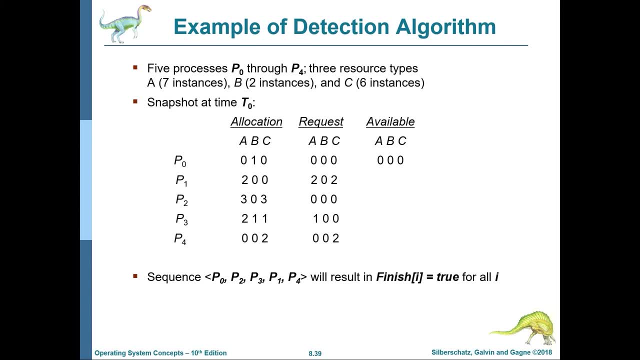 that is work, zero, zero, zero, Yes. So what we will do, we will mark the finesse of p zero to true And we will take its allocation of zero one zero and add it to work. So work is currently zero one zero. Then let's see what else can be satisfied. whose request can be satisfied? I think only p two's. 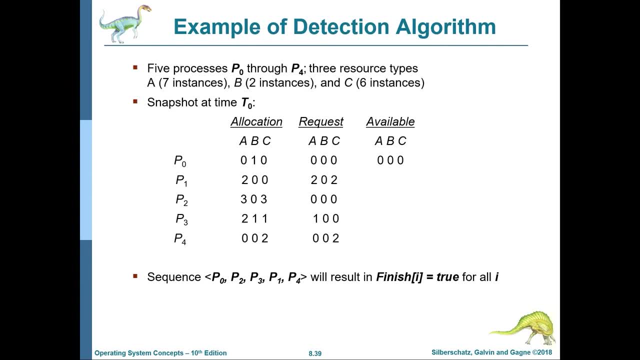 request can be satisfied, of zero, zero, zero, And so we will mark its finesse to true and we will take its allocation of three zero three and add it to zero, one zero, which is work right now. So work will become three one three. Then we can see that 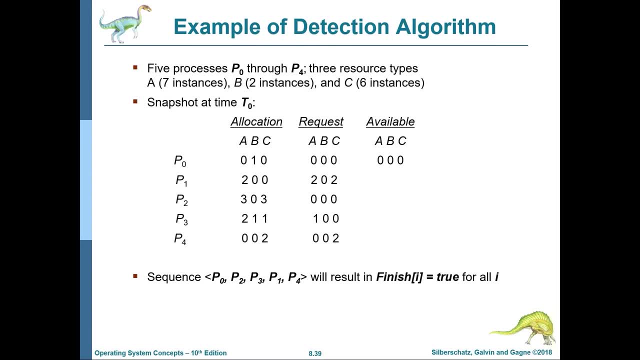 The request for P three and then the request for P one and the request for P four can be satisfied in that order And in the end the finesse of all the processes will be true. So there is no deadlock in the system. I recommend that you work this out in the notebook to understand how this algorithm 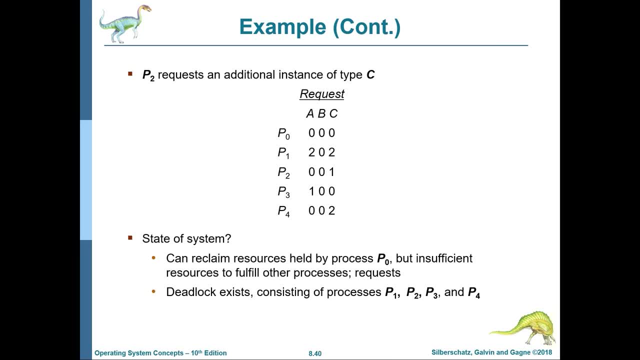 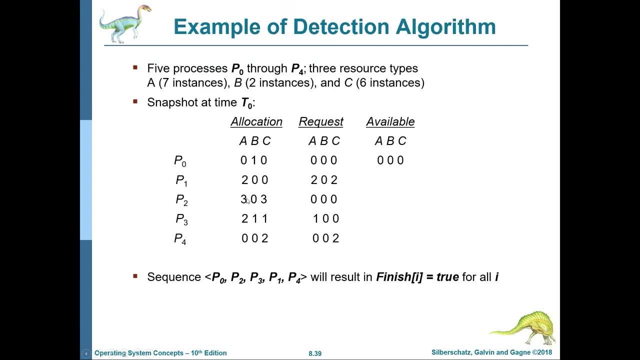 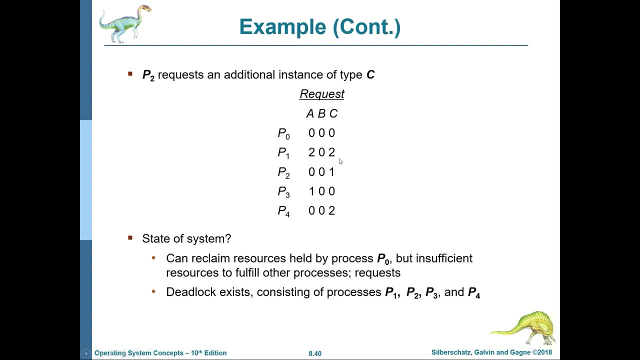 works. Now what if p two requests an additional instance of type C? Now P two was zero, zero, zero. before. in this slide, as you can see, P two was 000. now p2 has one request for type c. what would happen is that. you will see if you really 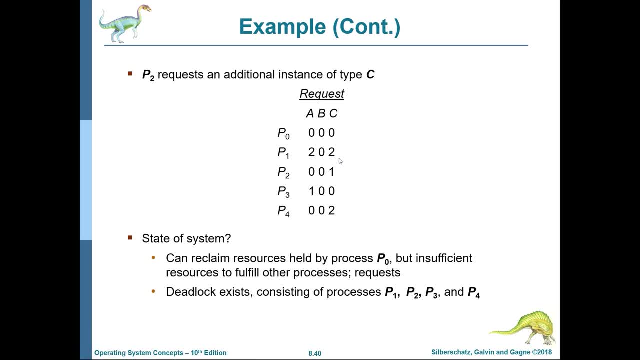 work this out on paper is that a deadlock will be introduced. now you can reclaim the resources held by process p0, but that is going to be insufficient resources to fulfill other processes requests. all right, because you will start with p0 and once p0 is done, you will take everything. 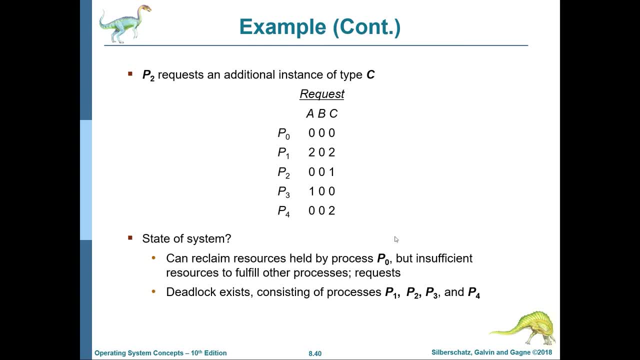 that was allocated to p0 added to the work pool, but after that none of the processes can proceed. in fact, processes p1, p2, p3 and p4, the all of them- will be deadlocked because the finesse values for those processes will still be false if you go over the deadlock detection algorithm on your notebook. 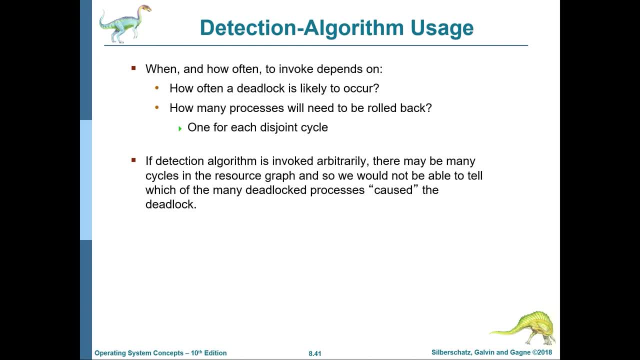 now that we have studied the details of the algorithm, we have to see when and how often we need to invoke it. it all depends on how often a deadlock is likely to occur and that depends on the system and the operating system. it is very hard to come up with, say we should run this every five minutes. 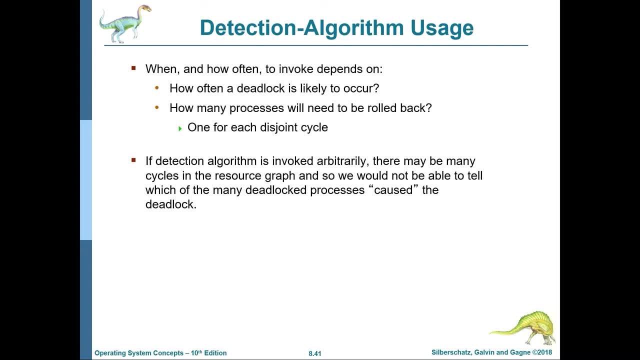 for everybody in the world. that is not possible and we have to see how many processes will need to be rolled back. so we need to roll back one for each disjoint cycle in the graph. so if the graph has many cycles now, those cycles can have common nodes. a disjoint cycle will not have any common. 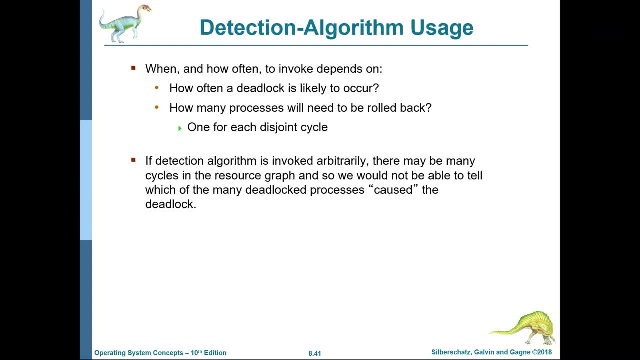 node with another cycle and if you just roll back the operating system, it will not be able to take one node on that cycle. then the cycle breaks and then the deadlock can be recovered from. if the detection algorithm is invoked arbitrarily, as in at one point of time you say i am going to 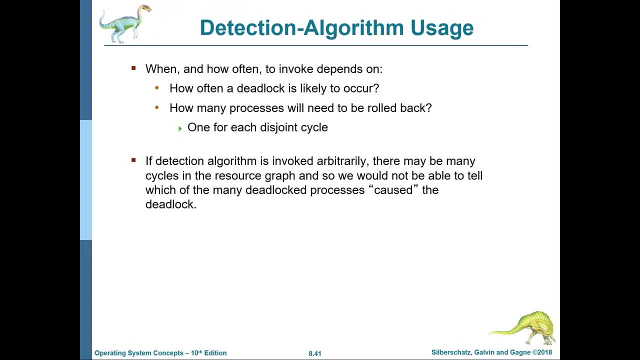 invoke this algorithm and i am going to find out who caused the deadlock. well, that is not possible from the resource graph, because the resource graph might have so many cycles that it is impossible to tell which is that one process. that is not possible. and if the resource graph is not possible, then 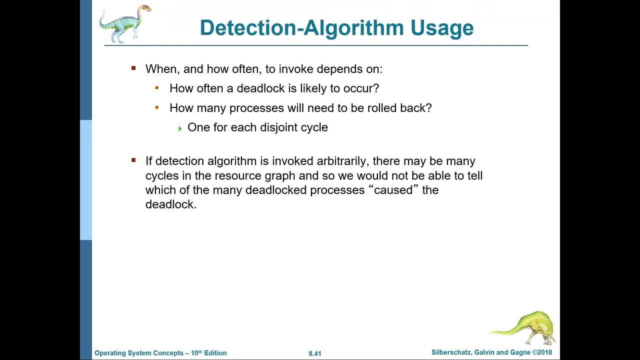 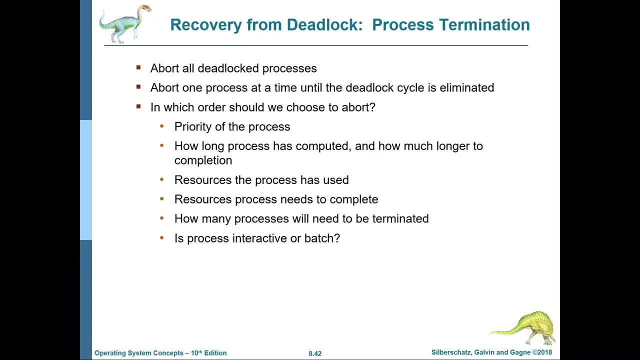 started this entire problem. now you can recover from deadlock by terminating processes. well, you can abort all the deadlocked processes, or you can abort one process at a time until the deadlock cycle in the graph is gone. in which order should we choose to abort the processes? well, we can. 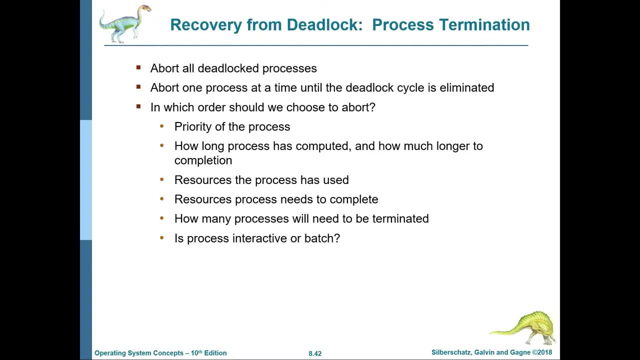 consider the priority of the processes. we can terminate low priority processes first and we can maybe look at how long the process has computed and how much longer to completion. if a process is almost near its completion, then we should not abort that process because by giving it a few more cycles it will be done. why waste all that computation? whereas a process which has 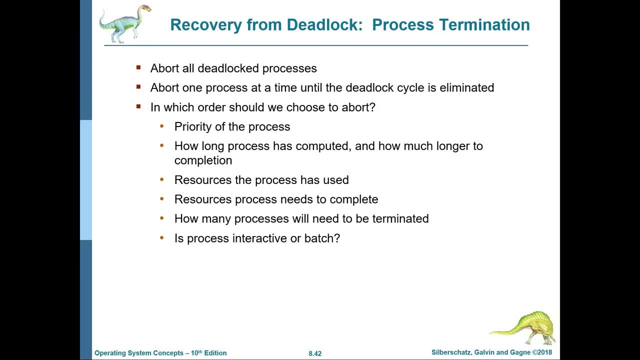 just begun executing should be aborted, because not a lot of, not a lot of work will be lost. that way we can also look at the resources the process has used. if a lot of resources have been used by the process, then we should probably let it run to completion, because 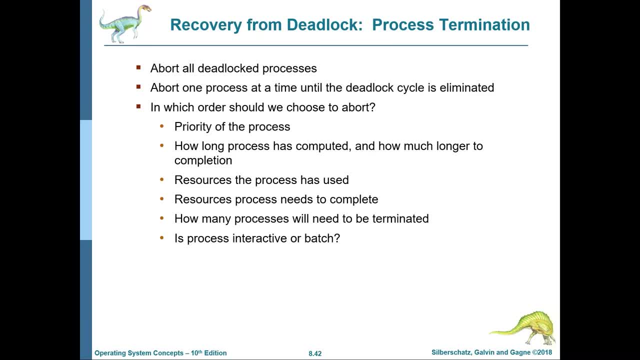 all the energy, all the time that was invested by the process will just go in vain if we just abruptly abort the process. then how many more resources the process needs to complete? well, that can be taken into consideration. we can also look at how many processes will need to be terminated, and are the processes that we are going to terminate? 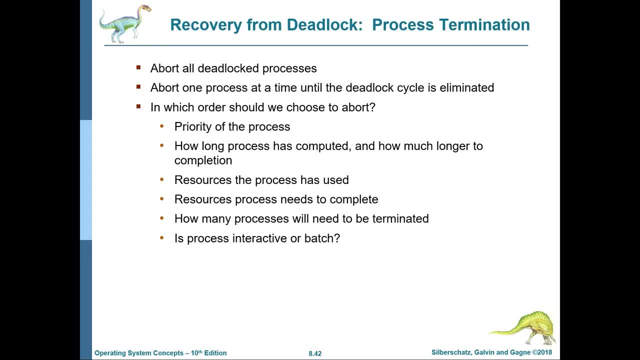 interactive or batch processes. well, interactive processes. if you abort them, it is going to be a really bad user experience for the users. just imagine you were trying to book something- a railway ticket or a plane ticket- and then the system just crashes the browser and says that: well, this is the browser process that is responsible for the deadlock and i'm going to abort this. 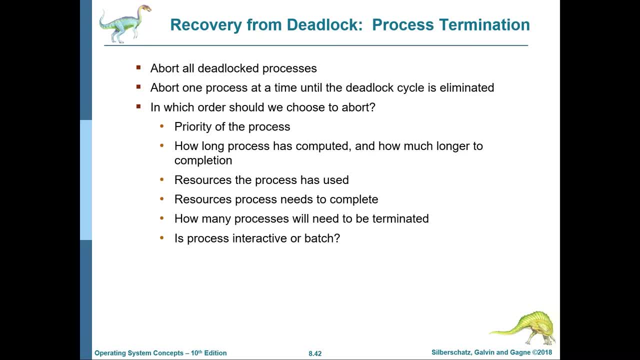 process. it is going to be a bad experience for the users and i'm going to abort this process. but if it is a batch process, as in, it just keeps working on a bunch of records like payroll or printing of mark sheets and things like that. if you abort it, it is very easy to restart it. 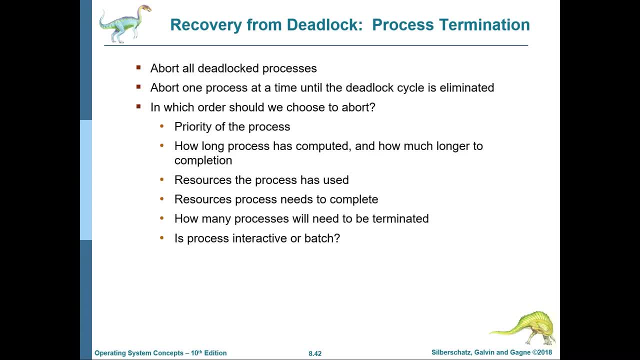 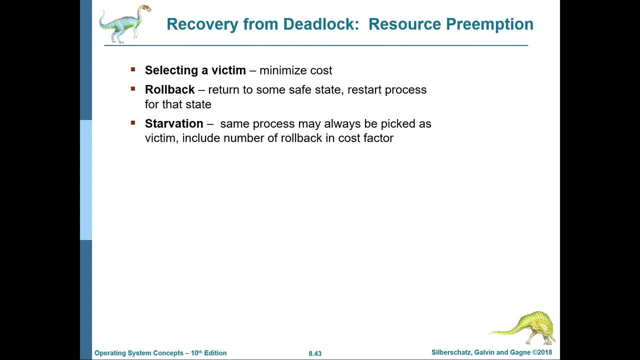 and users are not going to be unhappy because of a small delay in a batch processing system. there is another way to recover from deadlocks and that is by doing resource preemption. so processes have been allocated resources and you can take those resources away from those processes. and if you can take those resources, 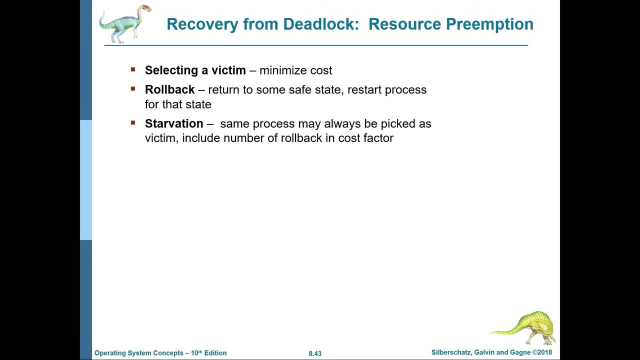 away from the processes and then allocate them to deadlocked processes, then maybe those deadlocked processes can resume their operations. so we have to select a victim. a victim is going to be a process from which you are going to steal a resource, and you have to steal it in such a way. 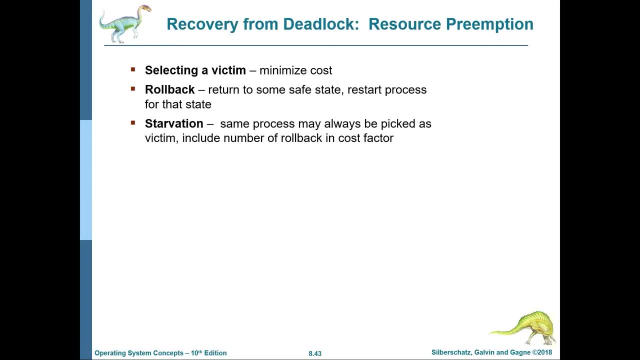 that the costs associated and the costs might depend on different factors, and some of the factors that we are going to deal with are the costs associated with the process and the costs that we are going to deal with are the costs associated with the process and the costs. 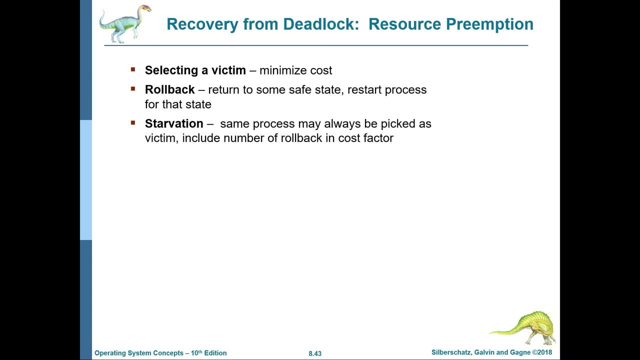 also studied in the previous slide. you have to minimize that cost. you just cannot take away a very important resource from a very important interactive process and say, okay, i'm going to take it away from you, and that is also going to be a really bad user experience to the user. 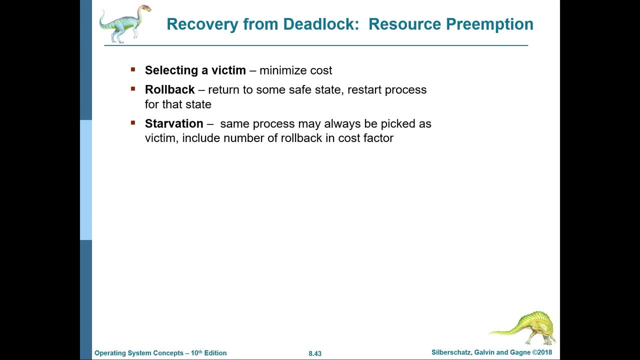 so you have to make sure that the cost of preempting a resource from a process is minimum. then you can roll back so you can return to some safe state and restart the process from that process state. and and you will only hope because, uh, when you are detecting deadlocks and you're trying to 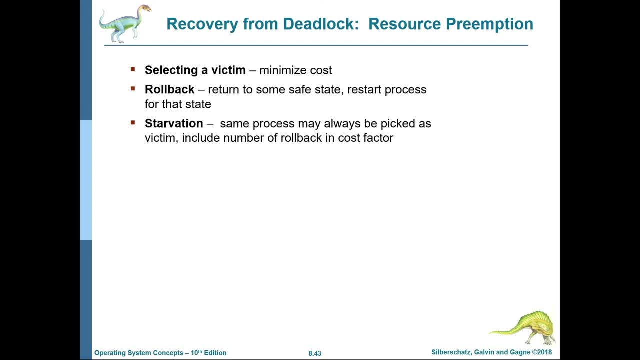 recover from a deadlock. it is very clear that you're not trying to prevent or avoid deadlocks, so you can just hope that this time around the process will go through a different path and deadlocks will not happen, so you will roll back to a safe state and restart the process from. 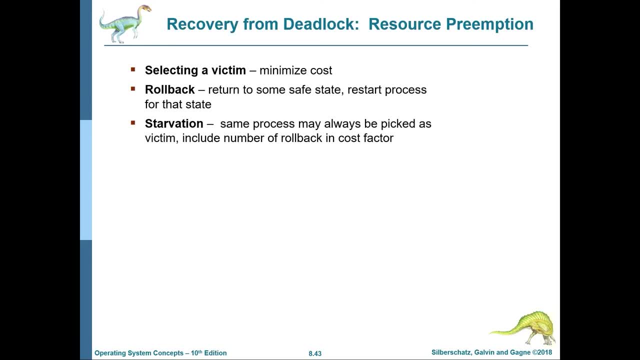 there. after you preempt the resource or a bunch of resources from that process, you can just hope that the cost of preempting a resource from that process will go through a different path. now you have to also make sure that starvation does not happen, because if you always roll back,